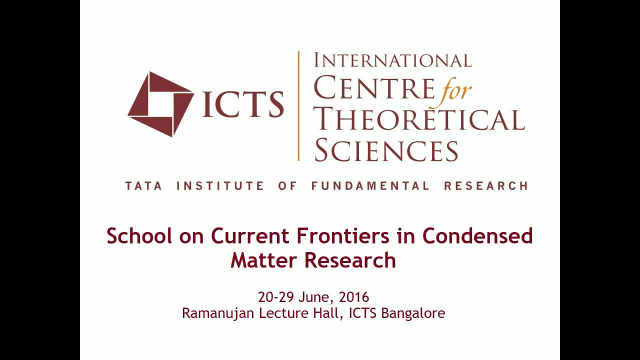 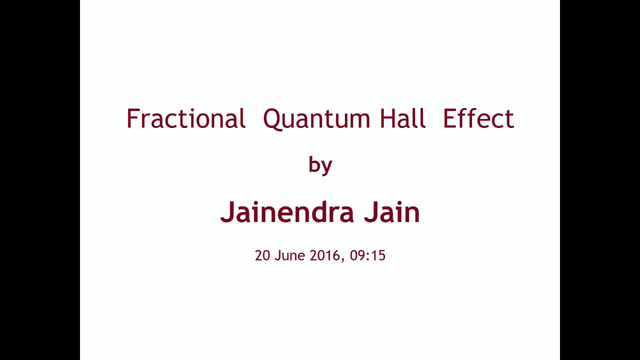 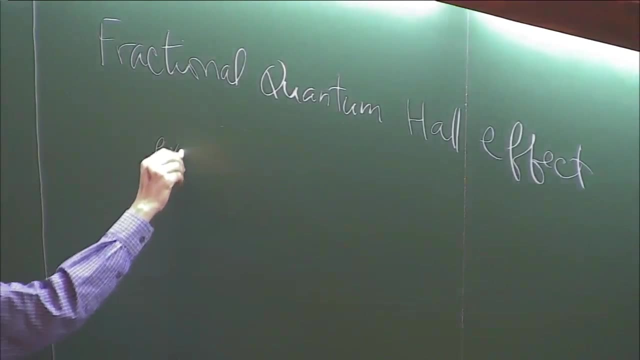 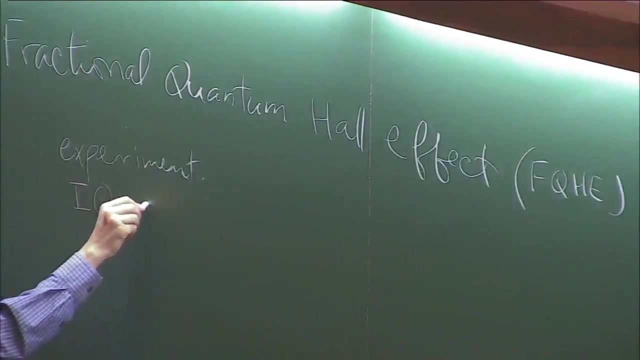 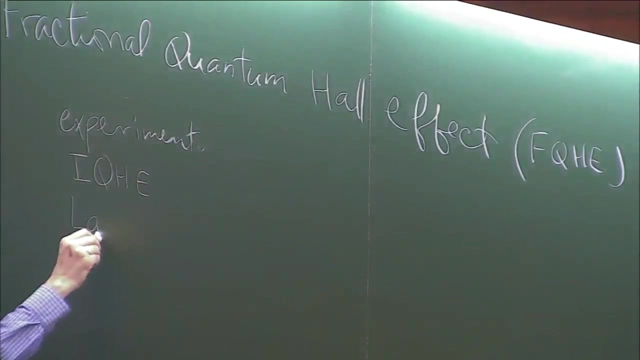 Outline of the lectures would be: I would begin with Experimental Phenomenology, Then I will go on to Integer Quantum Hall Effect Theory. So this is FQHE And I will go to Theory of Integer Quantum Hall Effect. Then I will go to Laughlin's Theory And in this 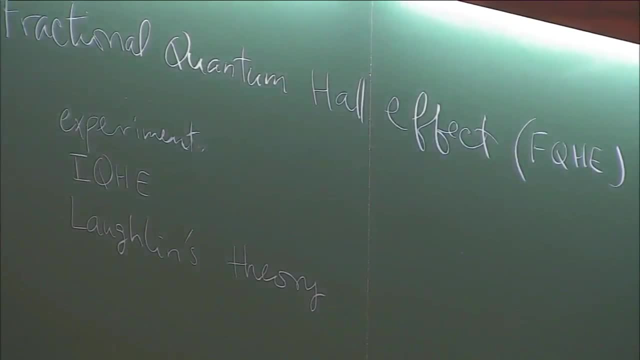 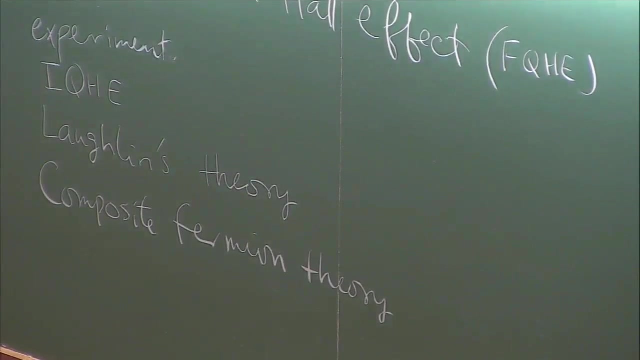 context, I will derive some very nice concepts such as fractional charge and fractional statistics, And at the end I will go on to Composite Fermion Theory And we will see how these things relate to the experiments. So some of these lectures are very difficult to understand. A lot of the things that I 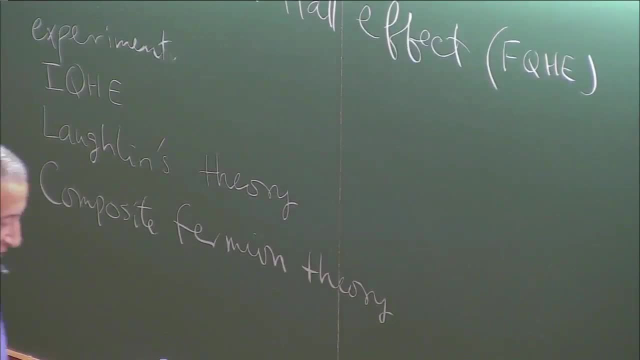 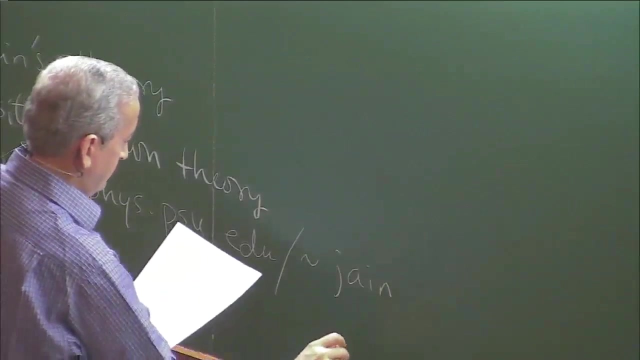 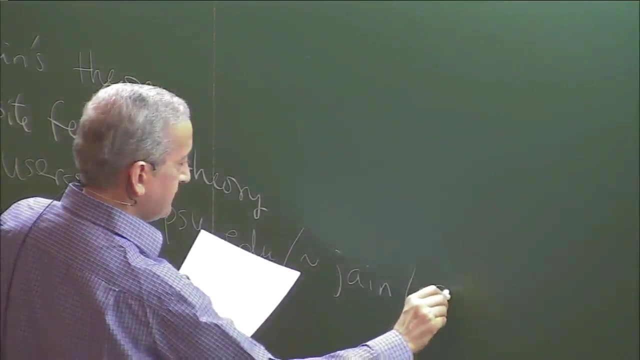 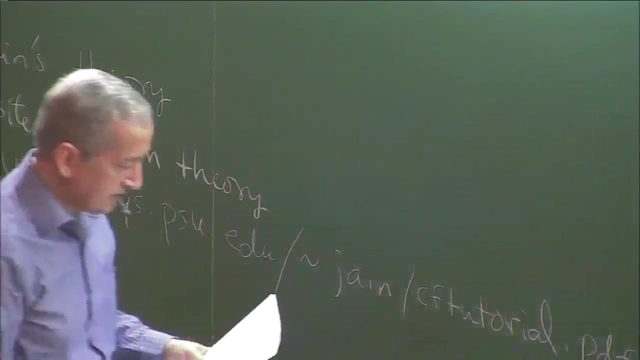 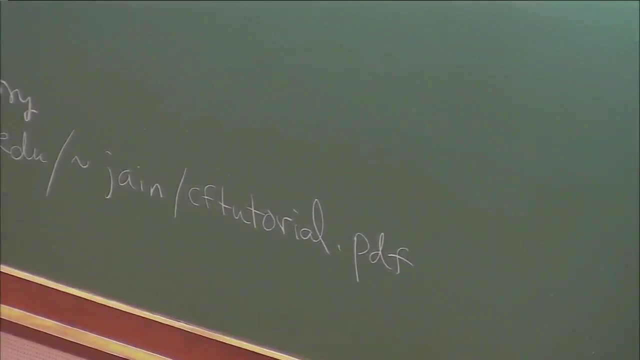 idea. it exists on the on the web. you can go to my web page. so let me list so you can consult some writer. that was based on a previous set of lectures i had given, actually in in a workshop conducted by the icps. there are also very nice lectures by david tong. 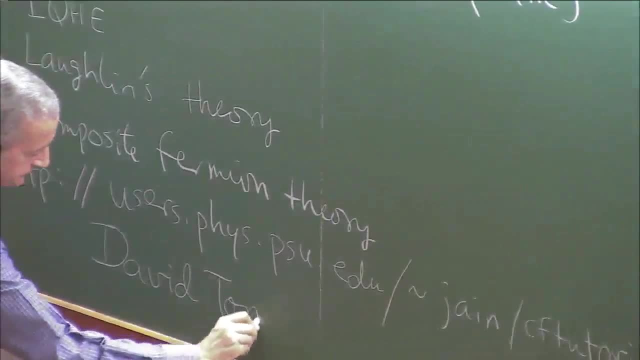 i believe these were emphasis lectures at tata institute. i believe if you put in david tong, factual, formal effect, such, with those keywords, you should be able to locate those lectures. and i have a problem set which you should be receiving at some point by email. so those who 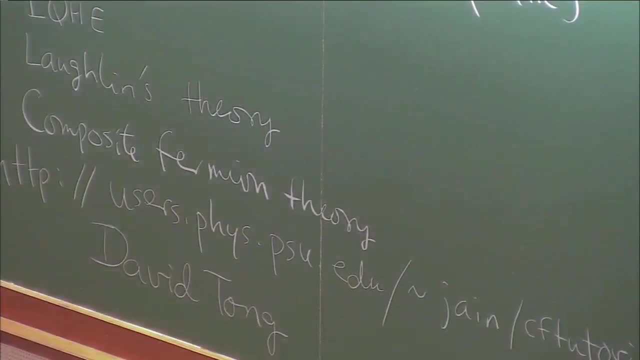 be things that you can just think about and work out in preparation for the tutorial at the end of the day. today the tutorial is two hour long and i will be converting one hour of that into a regular lecture, because i think having a two hour long tutorial just after 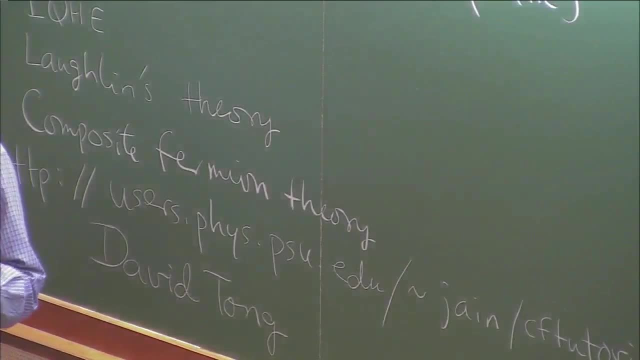 one lecture is probably not. i mean, we don't have enough material to do problems on a regular basis, so i'm going to give you a little bit of time to do that. so if you have any questions, please feel free to reach out to me and i will be happy to answer any questions that you may have. 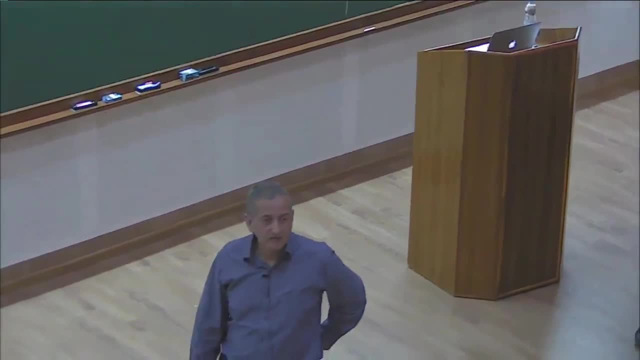 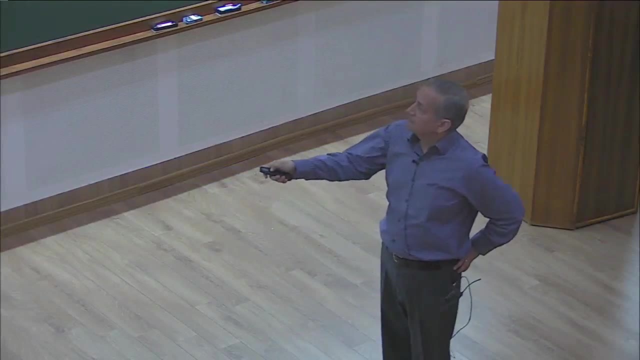 so thank you very much for your time and i will see you in the next lecture. thank you so much for your time and i will see you in the next lecture. thank you, it was discovered by edwin hall in 1879 at johns hopkins university. he discovered that 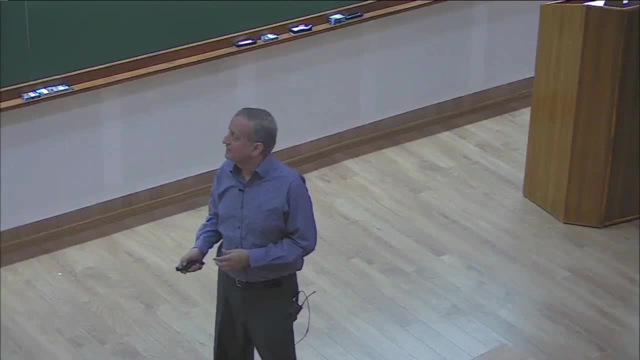 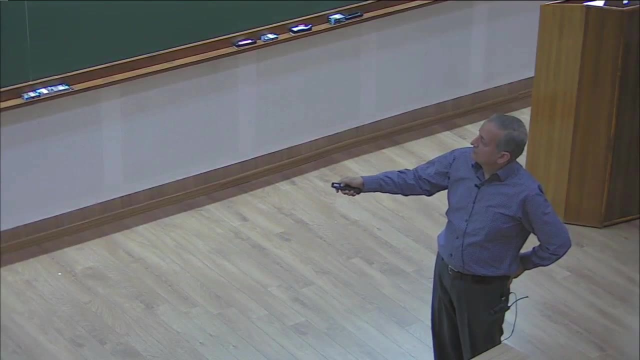 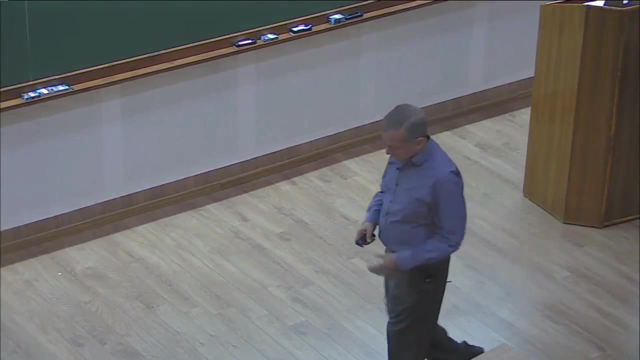 in the presence of a magnetic field. if you apply an electric field in some direction, current actually is a magnetic field and it is a magnetic field. and he defined the quantity that's called the hall resistance, which is equal to the voltage across the current path divided by the current and from. 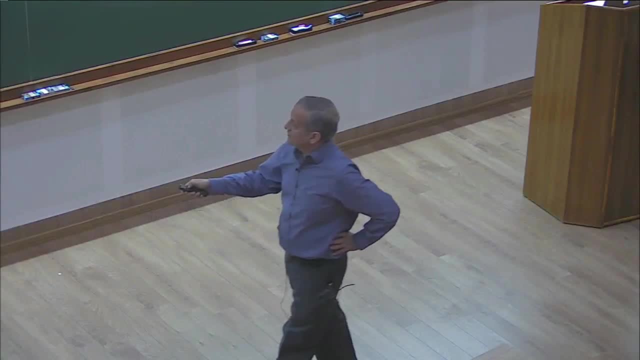 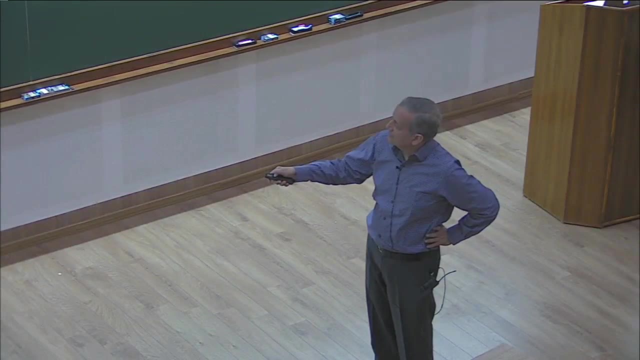 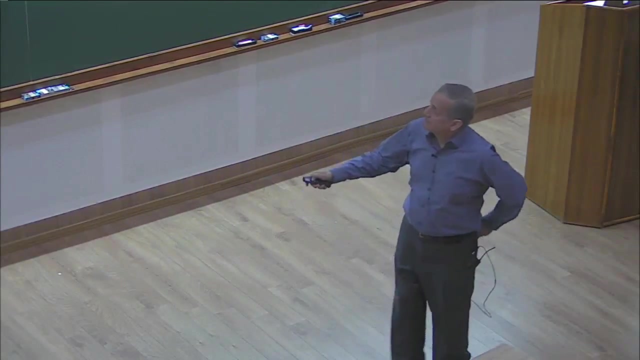 simple classical electrodynamics. one can show that this and we will show it later today. this quantity is equal to a magnetic field divided by the density of charge carriers times e, which is the speed of light. so the basic idea from this is that if you plot hall resistance, 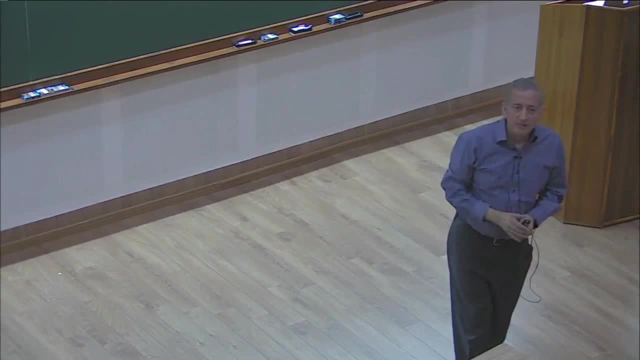 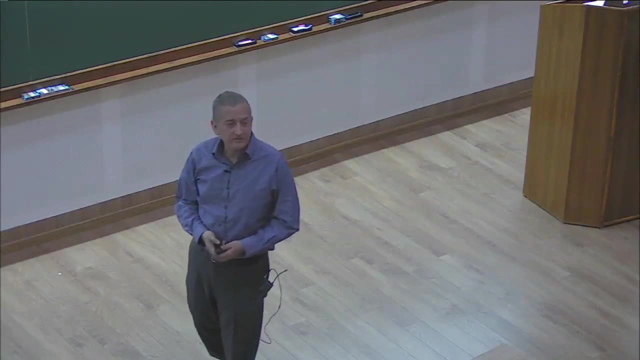 as a function of magnetic field. you get a straight line and the slope of the straight line will tell you what is the or. it depends on the density of charge carriers. in fact, this is one of the standard ways of measuring the density of charge carrier. it just measure. 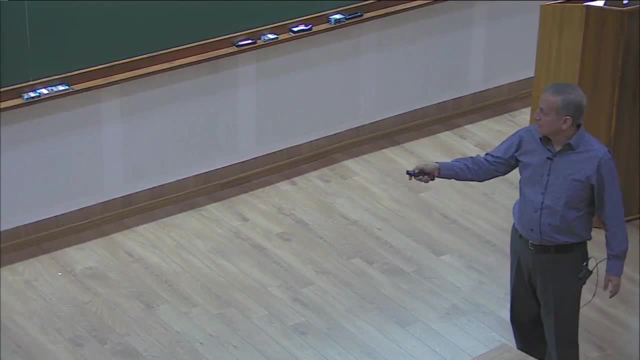 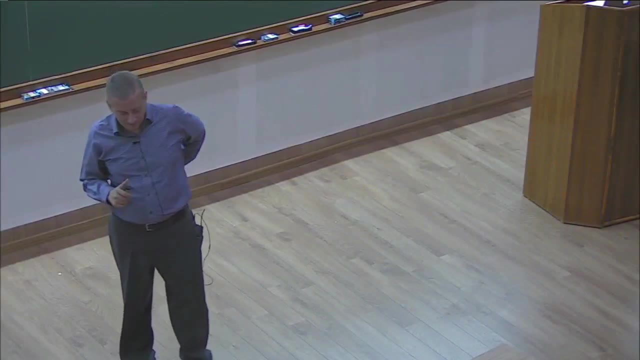 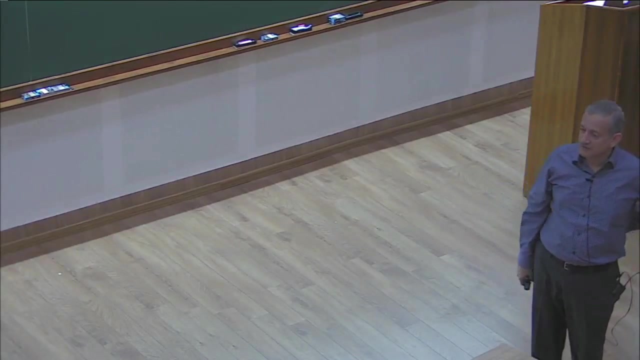 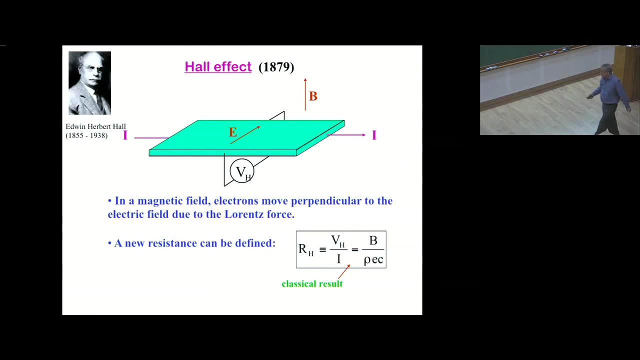 the hall resistance and from that you can read off the density. In fact, this was also how holes were discovered, because during some of these hall effect measurements they found that the sign was not coming out correctly and that was then understood in terms of holes. so this was the situation for about 100 years, about 100 years later. 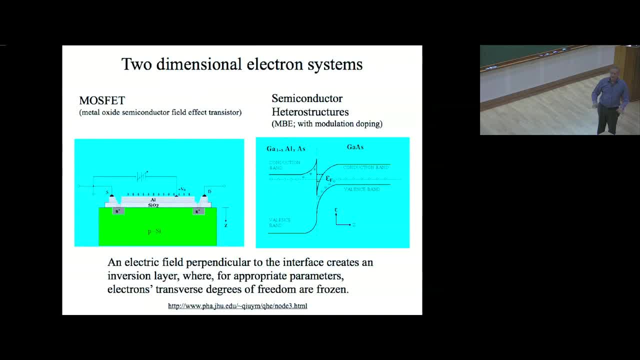 Klaus von Klitzing repeated these experiments and systems which are confined to two dimensions, and here I have shown a couple of ways of obtaining two-dimensional systems. so these MOSFETs that you have in your smartphones, they actually have two-dimensional gas of electrons at the interface between two different semiconductors. more recent experiments are: 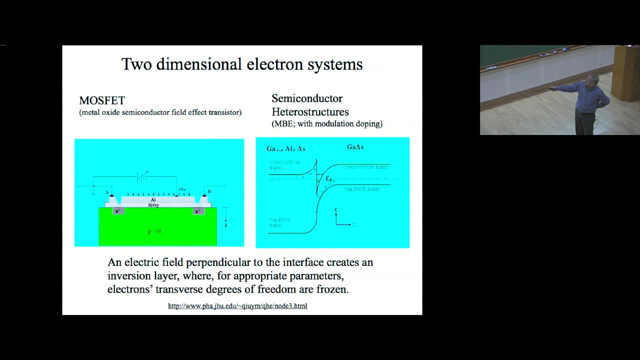 done with electron system, So this is a very interesting experiment. This is a system at the interface of gallium arsenide, gallium aluminum arsenide semiconductors. I am not going to go into the details of how or why a two-dimensional gas occurs at the 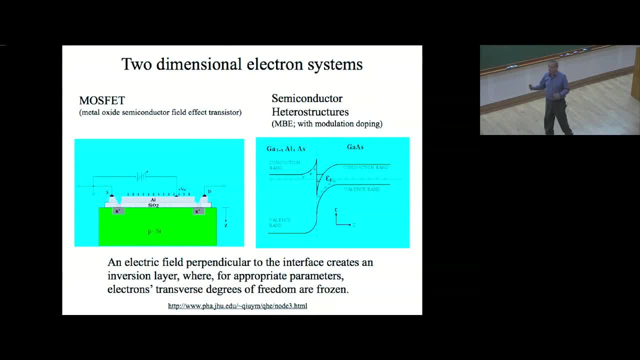 interface, but for us it will suffice to know that there is such a system. The system is two-dimensional in the sense that only the lowest sub band is occupied. lowest sub band, The lowest quantized sub band in the transverse direction, is occupied and therefore there. 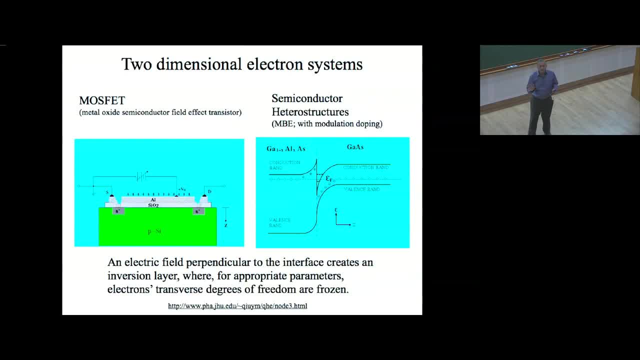 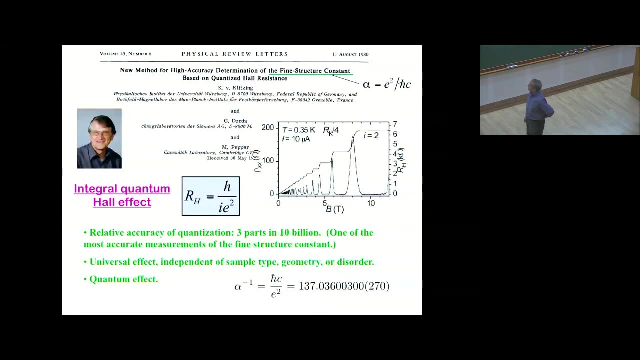 is no degree of freedom in the transverse direction. Electrons can move freely within two dimensions, but they cannot do anything in the perpendicular direction. Okay, so when Klaus von Klitzing repeated the experiment in these two-dimensional systems, he found something very surprising. 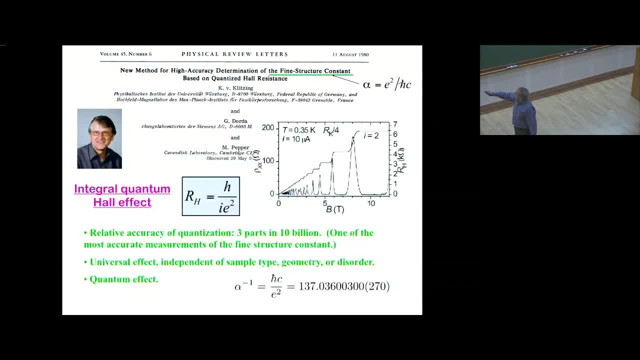 So initially at low quantization, At low magnetic fields, the Hall resistance started out the way we expect, going up linearly with magnetic field. but at higher magnetic fields he found that there were these regions where the Hall resistance was constant, it was not changing at all. 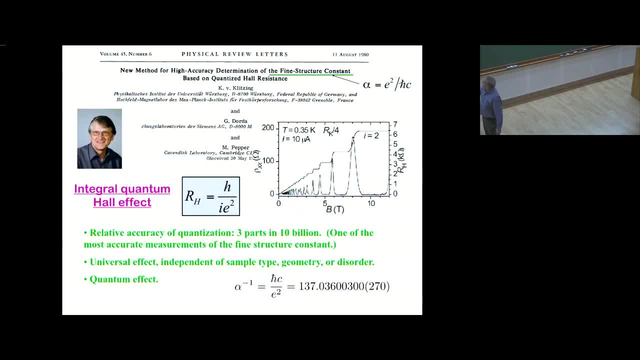 And, moreover, the ordinary resistance which is shown by this lower curve. it almost vanishes in this region. So whenever you see a constant Hall resistance, the ordinary resistance is almost zero. It is not exactly zero, but it is exponentially small and it is going to zero as temperature. 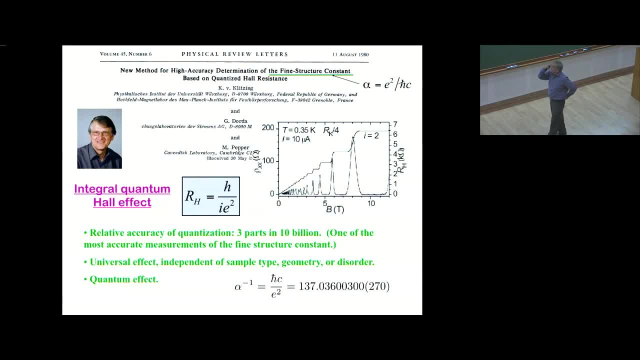 goes to zero. So this is, this was his discovery. and furthermore, he noticed something very neat. he noticed that the value of the Hall resistance on these plateaus, These plateaus, is given very precisely by this formula. So it is equal to h, the Planck's constant, divided by an integer times e, squared. 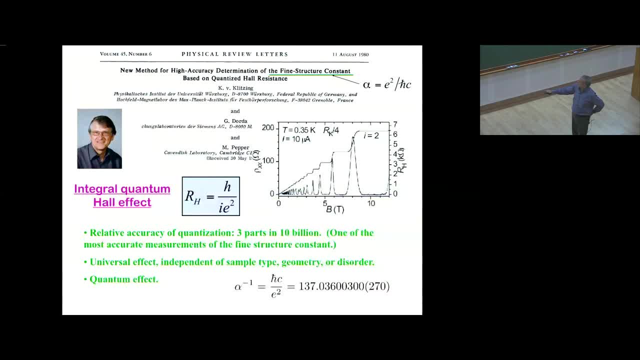 So, for example, here the value is h over 2 e squared. So this was very surprising. it was not predicted by theory, It was surprising because I mean. so first of all, you could ask how accurate or how precise is the quantization of the Hall resistance? and at this moment the resistance can be measured. 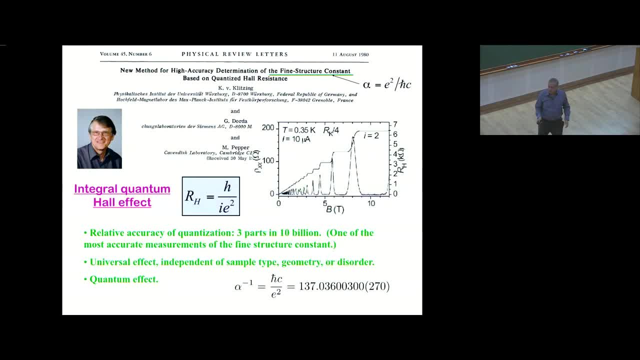 to about 7 significant figures. So it is certainly precise to that level. but it can take two different quantum Hall samples and you can ask how equal are the resistances for those samples. and that has been confirmed to a part in 10 billion. 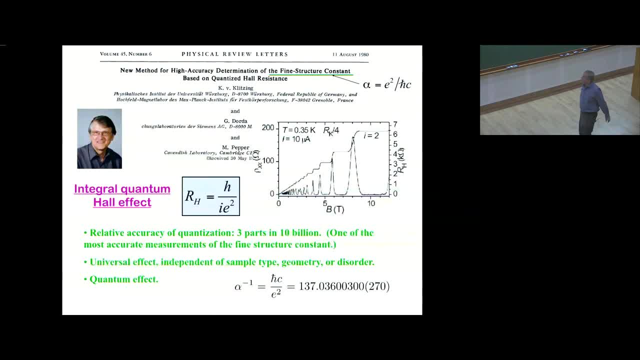 Okay, So as far as we know, Okay, So as far as we know, this equation is exact. in fact, this combination, h over e, squared, also appears in the definition of the fine structure constant. it also contains the speed of light, but that is known extremely precisely. 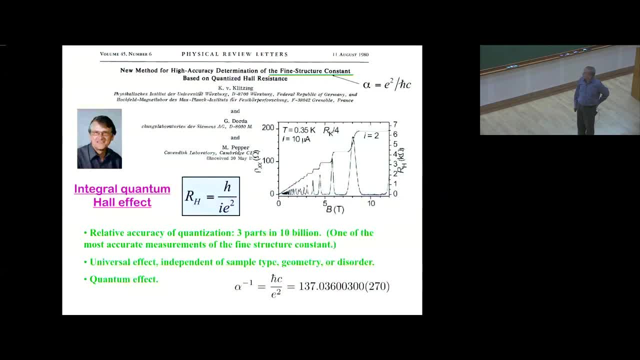 So these experiments are actually a measurement of an accurate measurement of the fine structure constant, and that was actually already there in the title of this paper. This effect is universal. it does not depend on what sample you take, how big or small the sample is, what is its geometry? it actually does not depend to a large degree on the amount. 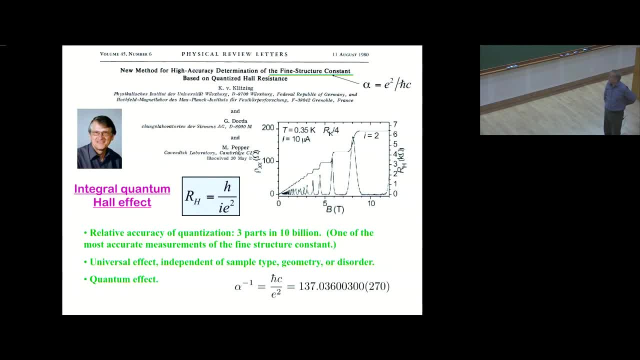 of disorder that is in there in the sample, So it is a very universal effect. Okay, So this was the discovery of the integer quantum Hall effect. it is called integer because this number- i here- is an integer. and it is called integer quantum Hall effect because 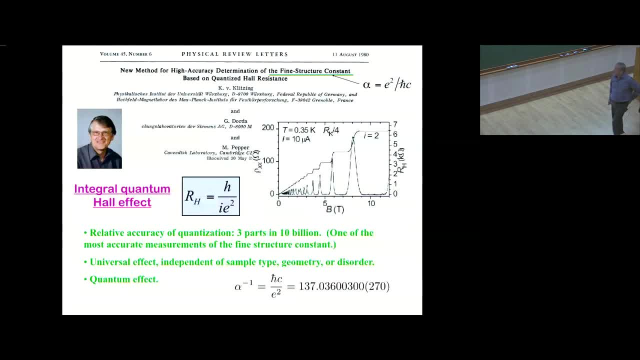 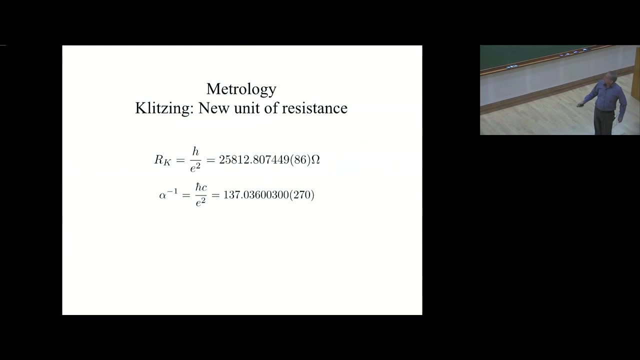 we will see that this number can also be a fraction in the next slide. Okay, So the basic phenomenon is a quantized Hall plateaus in regions combined with very small ordinary resistance. In fact, the ratio h over e squared has now been adopted as the new unit for resistance. 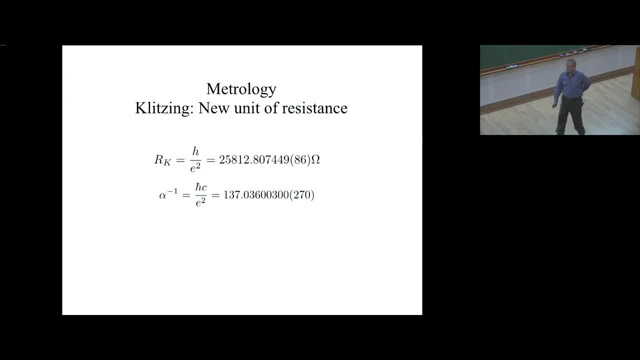 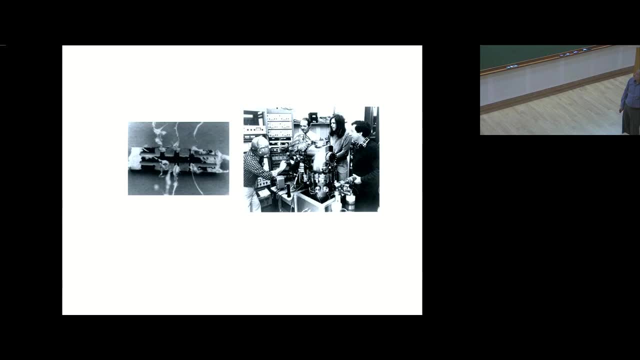 it is called the Klitzing constant- after the discover of Klitzing Okay, Then soon after that experiment. So this is a very simple experiment, It is called the Klitzing constant Okay. So this was, I think, in 1980, soon after that, some of these gentlemen went to yet higher. 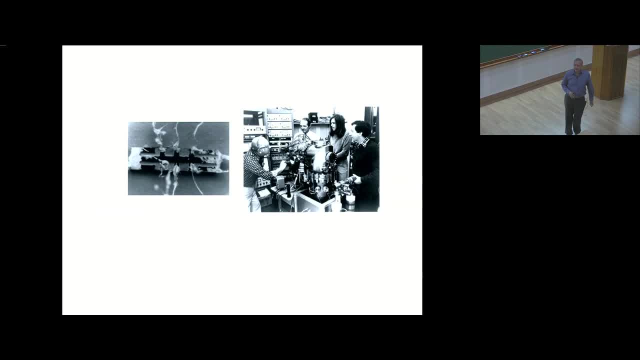 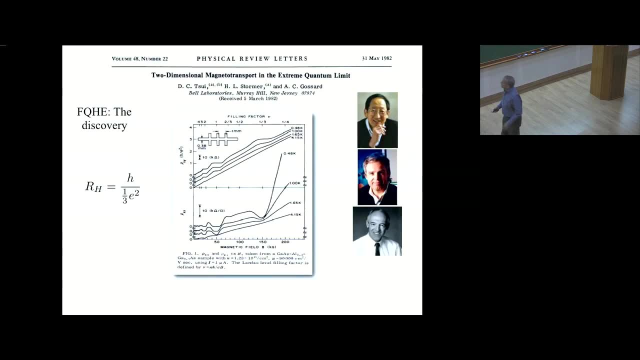 magnetic fields in better quality sample. and these better quality samples were these gallium arsenide, aluminum gallium arsenide samples, and they discovered something very surprising. They discovered that they discovered a plateau here where the Hall resistance is given by h, over one-third e squared. 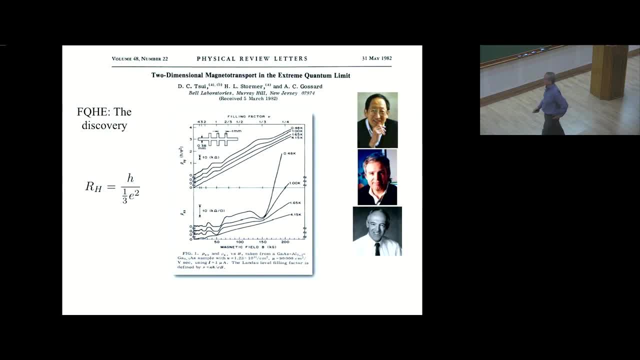 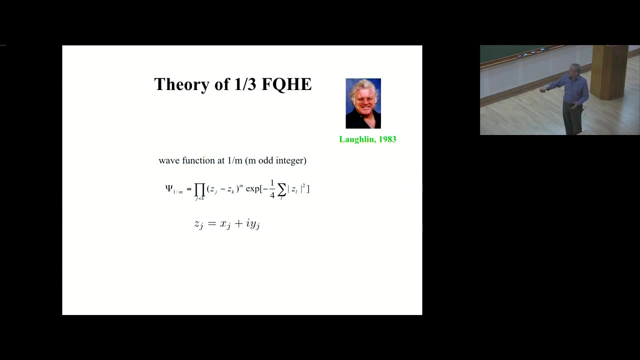 Okay, So instead of an integer we have a fraction. This was extremely surprising because that again was not anticipated by our understanding of the integer quantum Hall effect and a theory for this effect. the one-third plateau was written by Laughlin and I am going to I have shown you the basic answers of his theory. 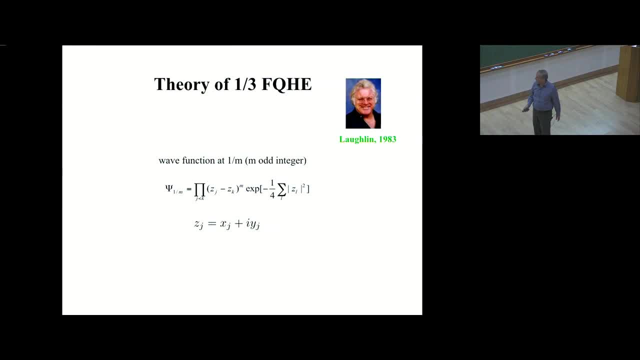 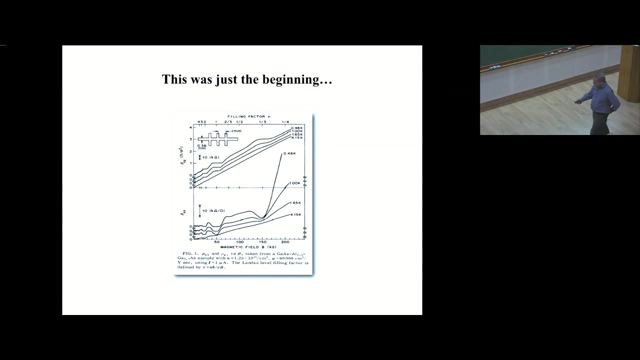 but we will come back to this in much detail later on. Okay, And it is for this that Laughlin Sui and Stormer won the Nobel Prize in 1998.. Now, it turns out that one-third was just the beginning, so this was the initial data. 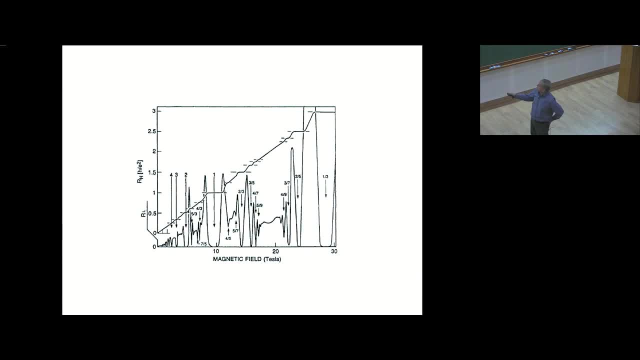 In a few years, data started looking like this. so these are all plateaus. this is ordinary resistance, so each minimum here has a plateau associated with it. each plateau has a fraction associated with it. so fractions like one-third, two-fifths, three-sevenths, four-ninths, a huge 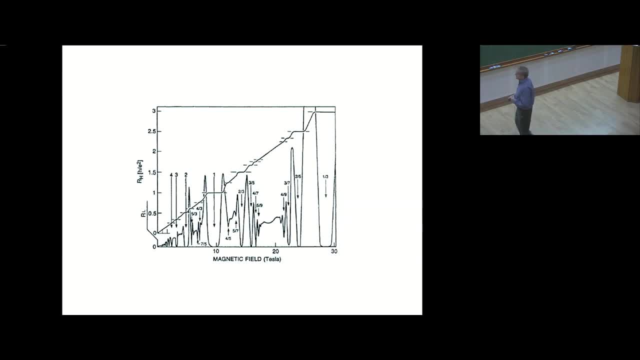 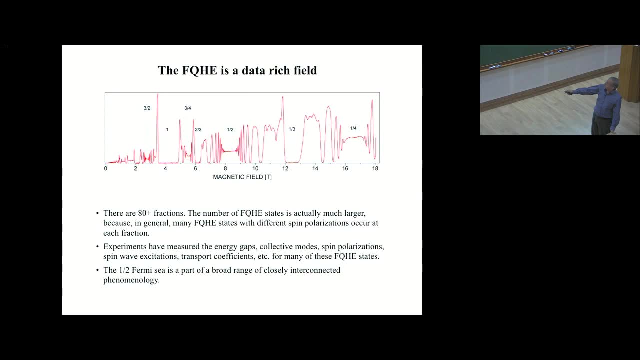 zoo of fractions was seen very soon. In fact this is another such picture where I show only the ordinary or the longitudinal resistance. but remember, each minimum here has a fraction associated with it. so I mean to date there are hundreds of them. 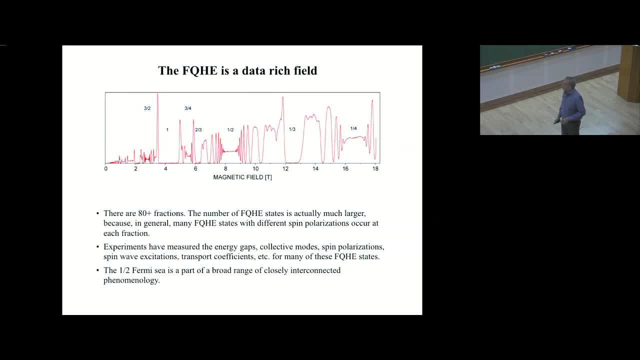 Okay, Okay. So in the last few years there are more than 80 fractions that have been observed. Experimentalists can measure various properties of the states at each of these factors. so, for example, they can measure energy gaps, elective mode, excitation, spin polarization. 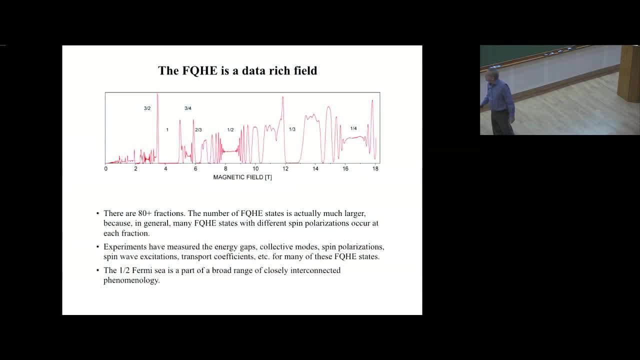 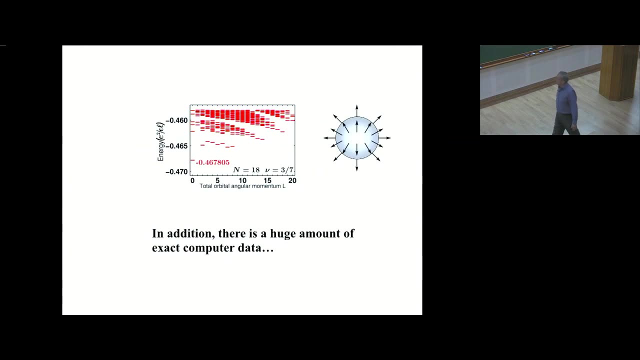 spin wave, various transport coefficients et cetera, is a huge. I mean it's a data rich field, huge amount of data, and to this we can also add theoretical data. so we'll see that in Paxil-Hollifax one can actually- I mean theorists- 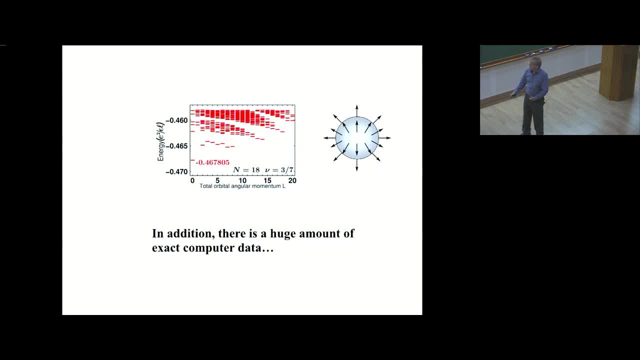 can take a few particles, put them on the computer and generate the full spectrum to all eigenstates and eigenenergies. so you can take different numbers of electrons, expose them to different amount of field and generate lots and lots of such spectra. okay, So this is the phenomenology. so please tell me. let's talk a little bit about what puzzle. 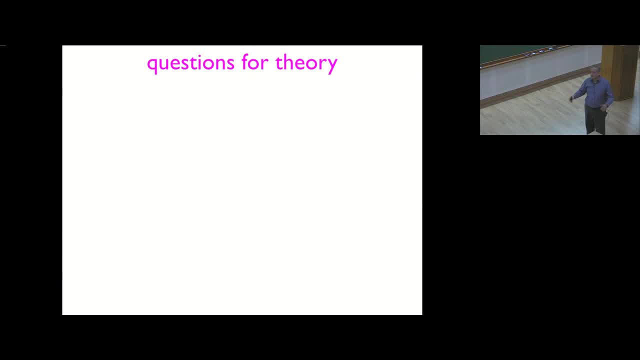 or puzzles. it presents us with what questions can theory ask? Can somebody? I mean, how many questions are there? why? so you can ask, for example: why is there Paxil-Hollifax right? what else? sorry, excertations, yeah, what are the excertations? 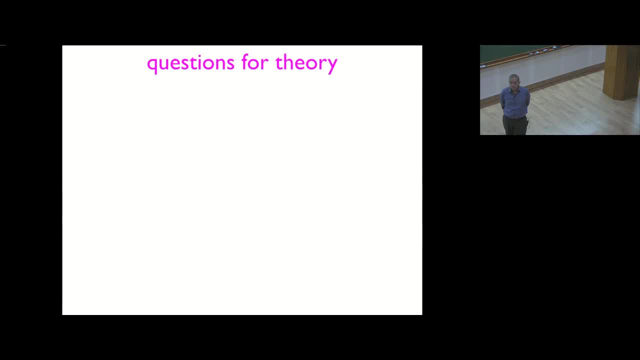 for example, What do you speak louder? What are the limits in which you see the fractional quantum hall and which limits you see integer? Okay, so in which dimensions do we see Paxil-Hollifax and at which dimensions is the integer Hallifax? 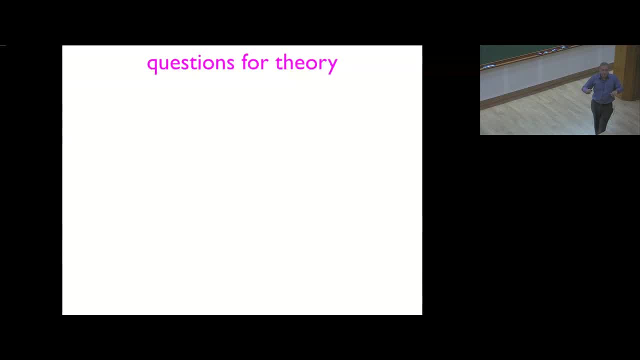 So the The experiments I showed you, they're all done for particles confined to two dimensions. No, as in. But one can certainly ask whether any of these phenomena are possible in higher dimensional systems. No, as in. I meant in which materials you would see. 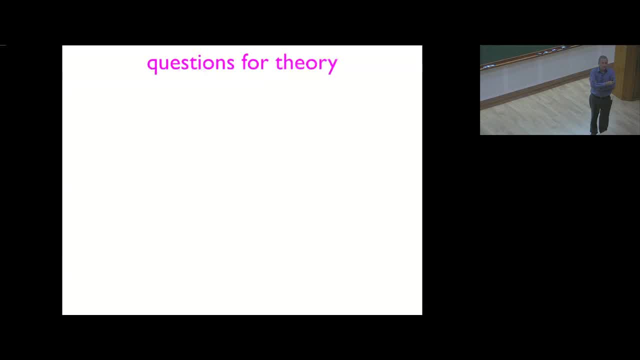 Oh, in which materials? Okay, The limits. Yes, Certainly very interesting, And there are lots of ideas on that. So there are even ideas on how to see these things in cold atom systems, for example. So what else? 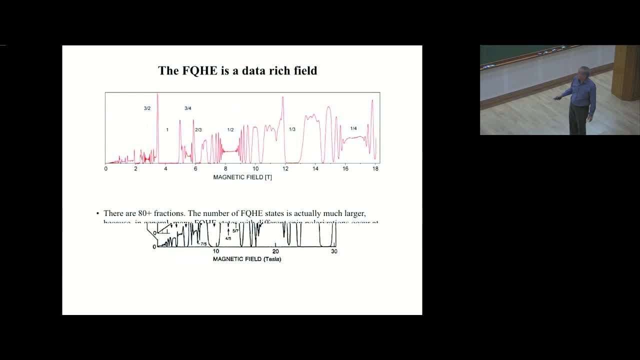 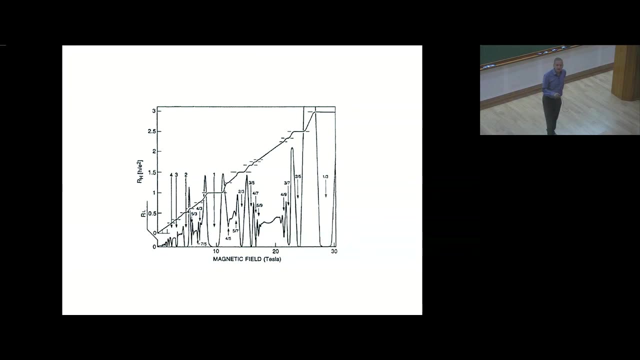 See. another question one could ask is: why are we seeing these fractions? Why one-third, Why two-fifths, Why three-sevenths? You know, if you stare at these fractions for a while, you realize that they all have odd denominators. 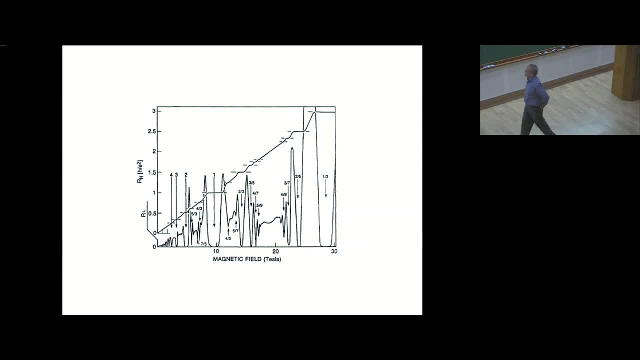 In particular, if you look somewhere here you might say: why don't I have a one-half, Why don't I have? So one could ask the question. I mean, in fact, the theory of fractional Hall effect must answer the question of why these are the fractions which are seen, why we don't. 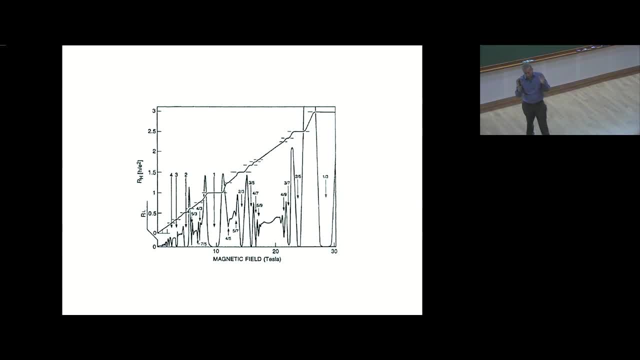 have odd denominator fractions. sorry, why do we have odd denominator fractions? why don't we have even denominator fraction? You could then ask: why is this much stronger? You see, this plateau is much stronger than this one or this one, So there is some sort of ordering of stability of these fractions. 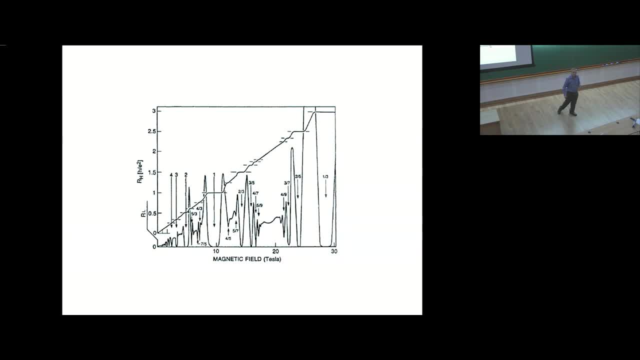 You could ask: why is that happening? So there are lots of different questions. You could ask: what's the role of spin? Can we have spin playing a role at any rate? Yes, Ok, Any other questions? So you know, I showed you these theoretical data. at some level you know computer data. 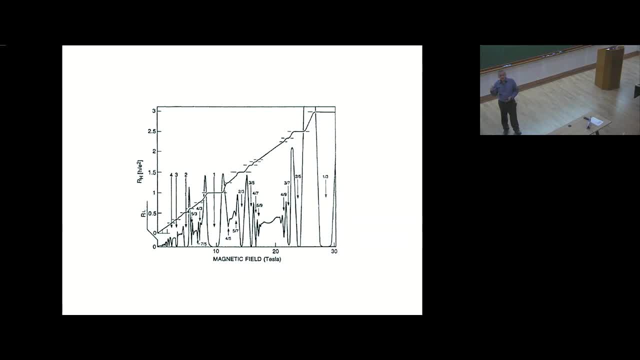 I should say The computer can produce data which are as good or better than what experiments would produce, because computers give us the full way to solve the problem. function all Eigen states and Eigen energies, So we would like to understand what are those. 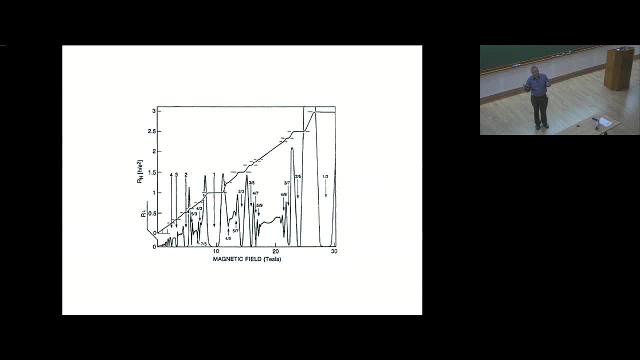 Eigen states, what are the Eigen energies, etcetera. okay, So this is the part with experimental phenomenology. any questions about it? I mean, why is this effect robust against changes in geometry and disorder and presence of defects or any other features? 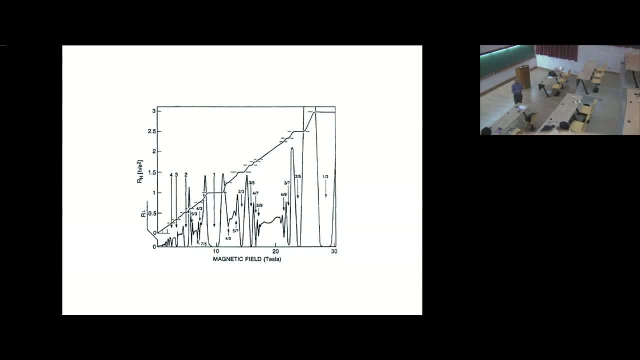 That's another very good question. So why is the effect so universal? Why is the quantization so precise? Yeah, Okay, So that's a question we'll come to later on, but it's a question that you know is certainly a very valid question in light of the data. All right, So all of. 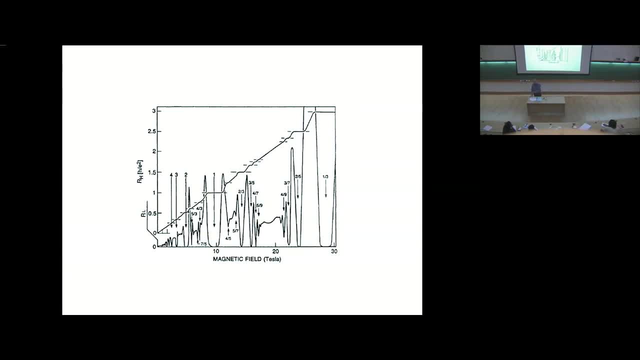 these questions will be answered as we go on. Okay, So the first thing we need to know is how to think about electrons in a magnetic field, quantum mechanically. So we all know what electrons do classically in the presence of a magnetic field. Classically. so, if an electron is going in a certain direction and 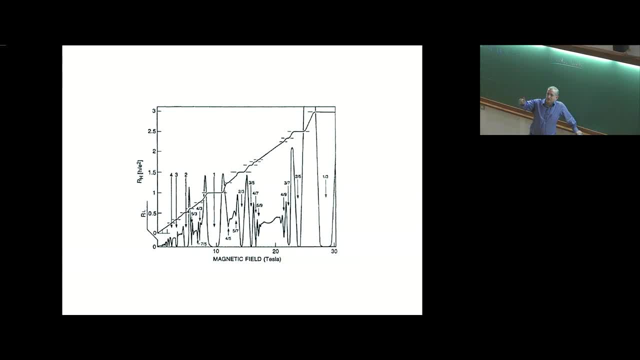 if you apply a magnetic field, it's going in a certain direction. and if you apply a magnetic field, it's going in a certain direction, Then there is a centrifugal force on the electron and that will force the electron to go around in circles. So that's the classical picture we all know. Let's try to understand. 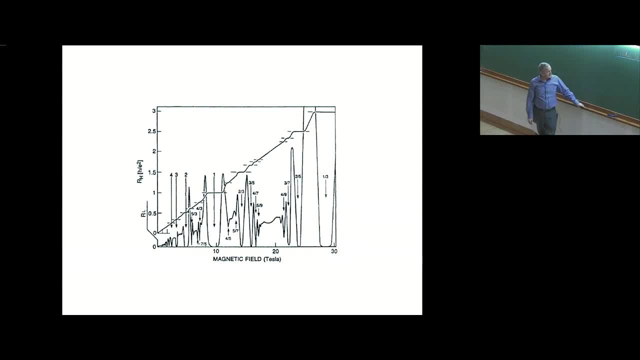 what electrons do quantum mechanically, and this is a problem that was solved fairly early on by Landa, Okay, Okay, So let me show you. So this is very simple problem. So this is a very simple problem, So the solutions of this are called Landa levels. In fact, it was solved a couple of. 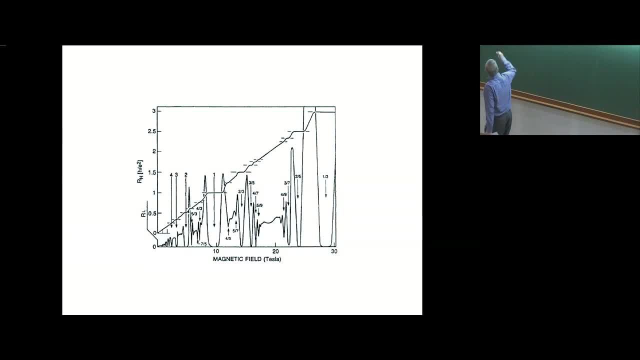 times, even before Landa, by some, by these two gentlemen, Darwin and Pock. In fact, they had solved a more complicated problem, in the sense they solved it in a much more complicated way. Okay, the problem of an electron in a parabolic potential, which is one of the home assignment. 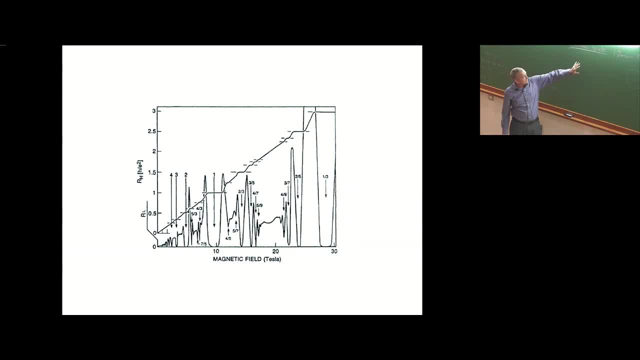 problems that we will be doing. but I think there is a law that every effect is named after somebody who is not the discoverer of the effect. so here it is called Landau levels, So the problem that we want to solve. so we are first going to take just one electron. 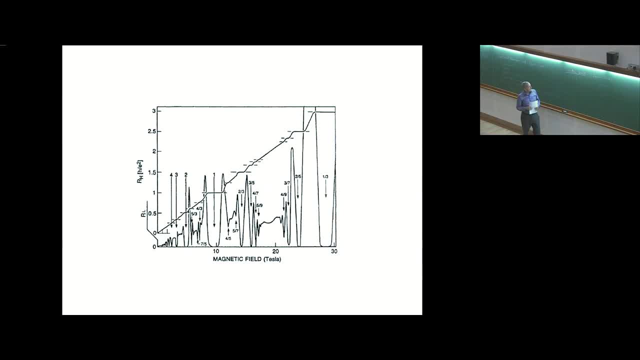 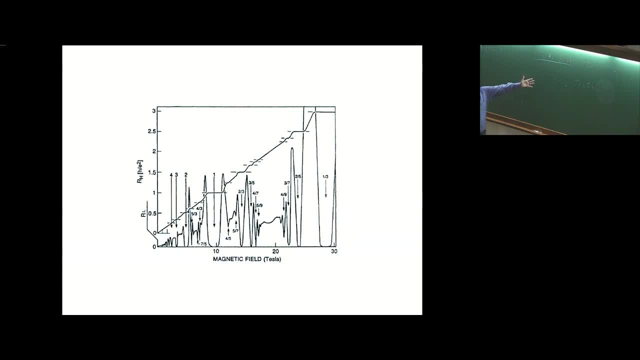 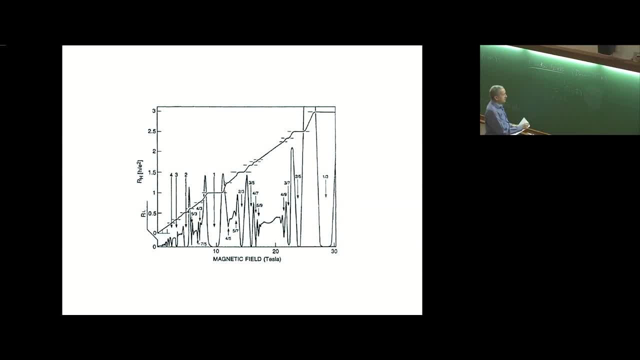 transformation. the two choices that will be useful for us in this lecture are: one is called the Landau gauge, and here, so you can easily see that if I take curl of this quantity, that gives me magnetic field pointing in the Z direction. the other choice is called the 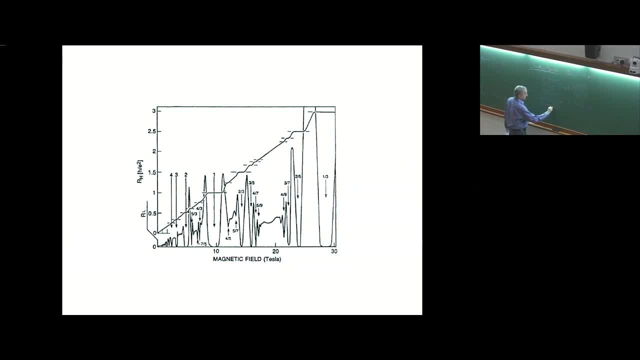 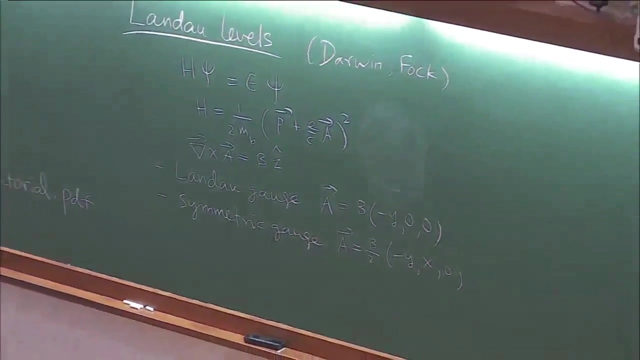 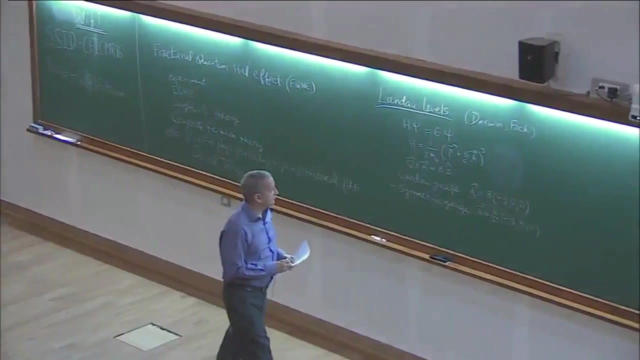 symmetric gauge. So again, you should confirm that curl of A gives you magnetic field pointing in the Z direction. So why we are working with these two gauges It will become clear as we go on. but let us quickly see what these two gauges do. 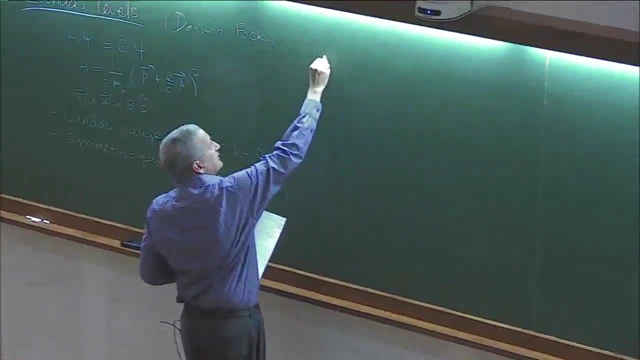 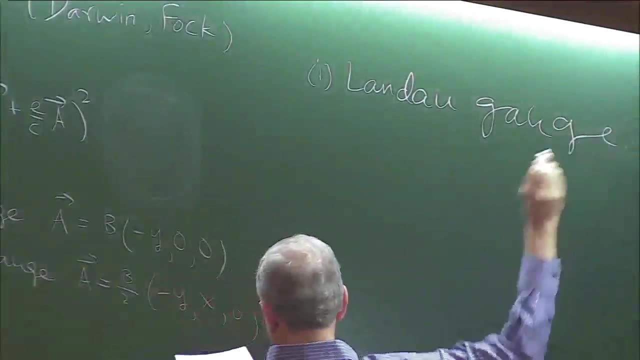 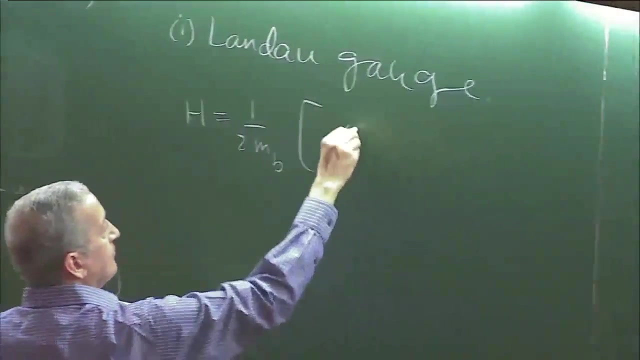 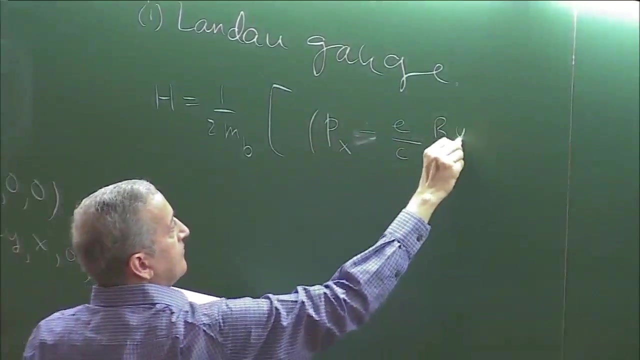 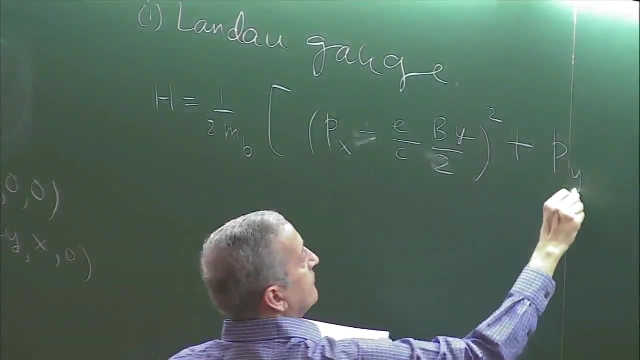 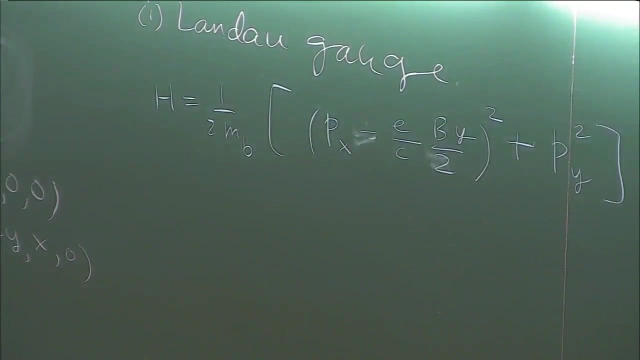 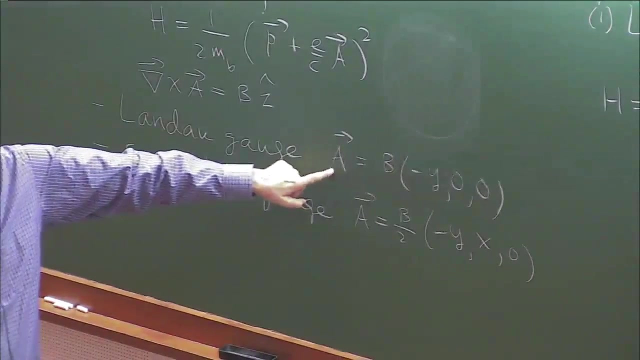 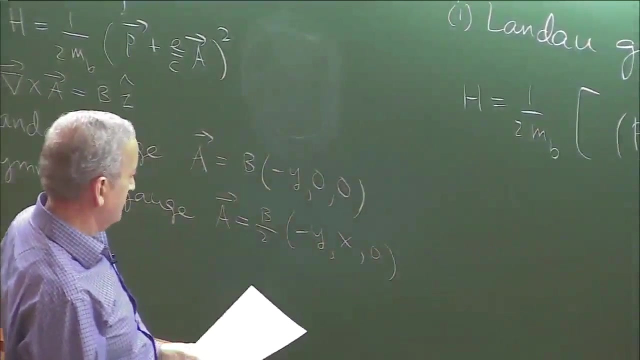 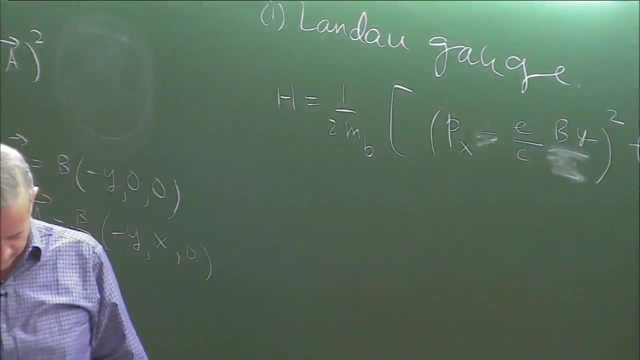 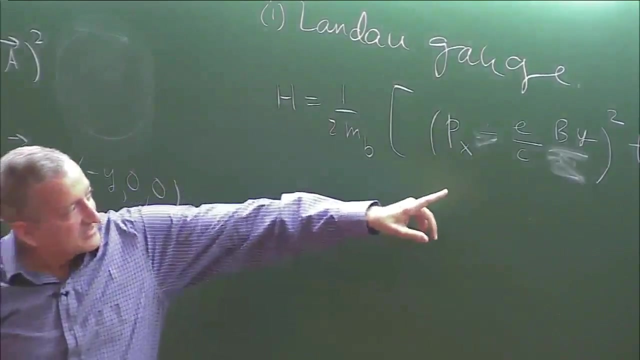 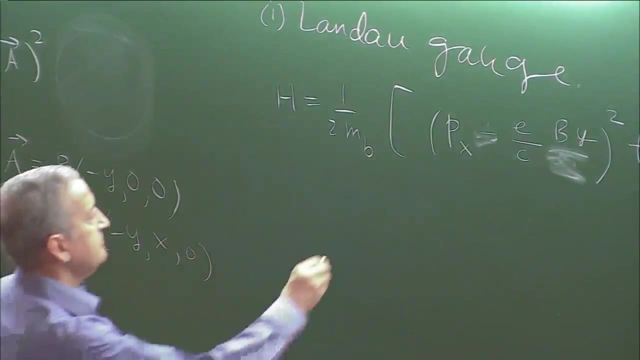 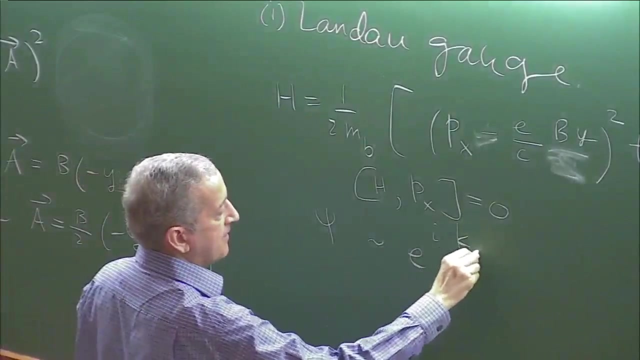 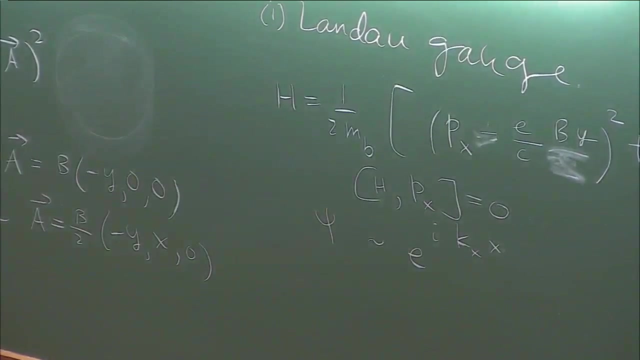 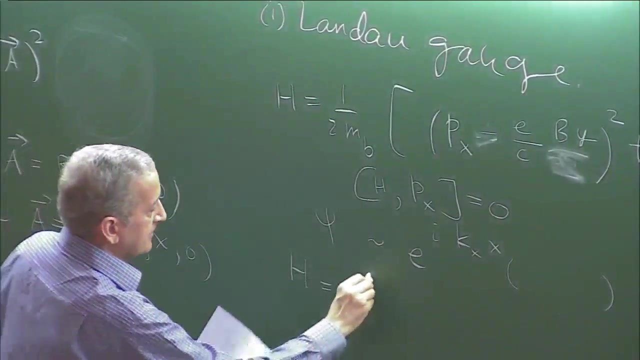 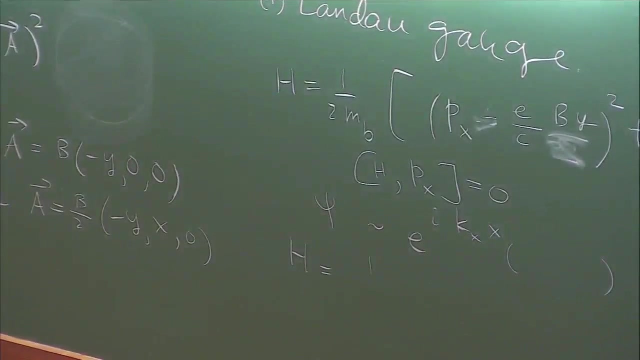 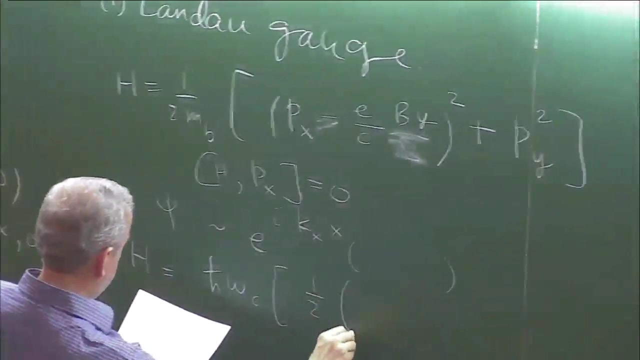 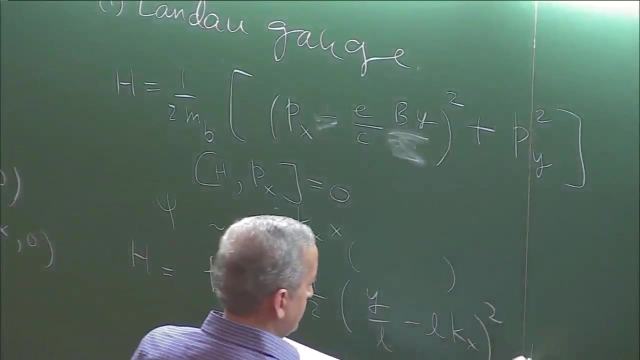 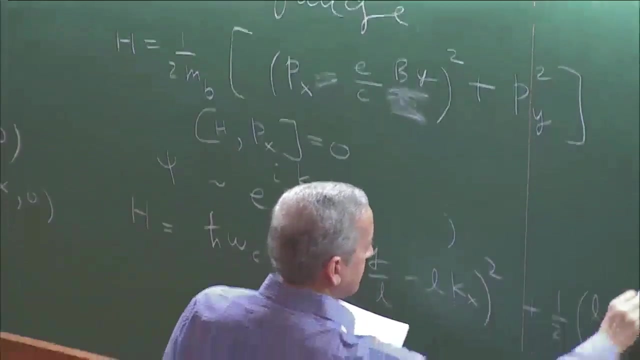 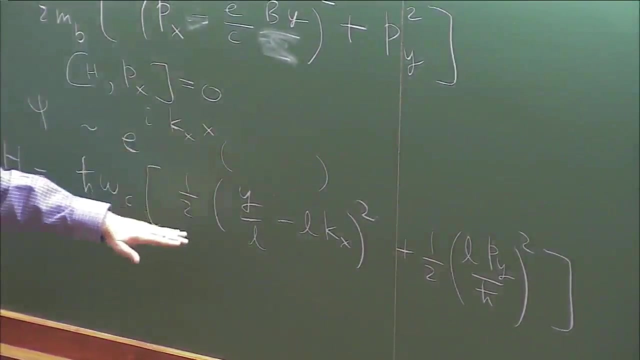 So let us first work with Landau gauge so I can make the substitution in the Hamiltonian that will give me. So here I have. I mean, you can already see that this equation is the same expression except for a definition, except that I have defined a couple of quantities. here one is: 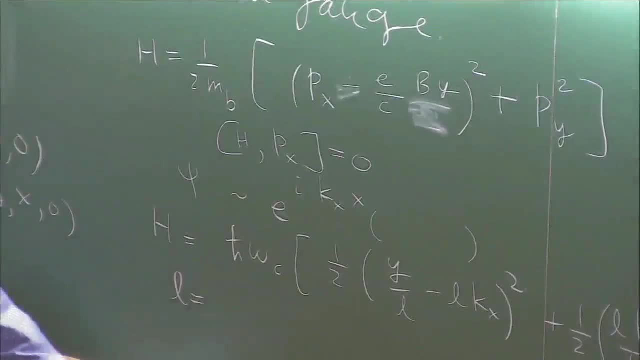 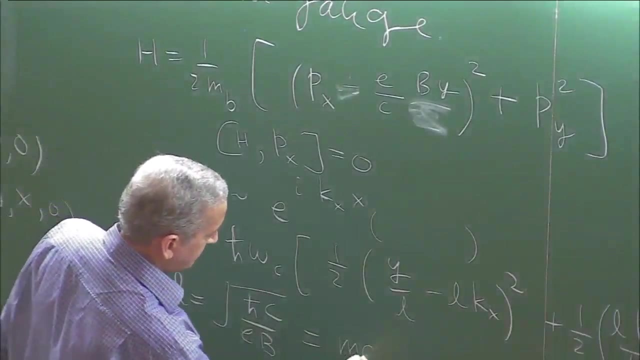 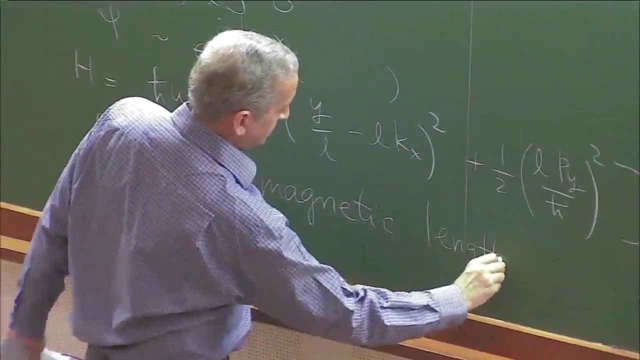 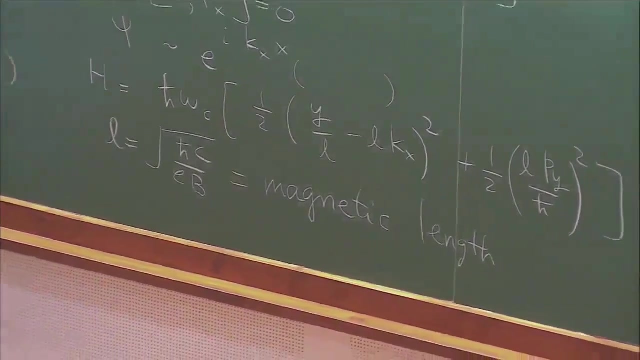 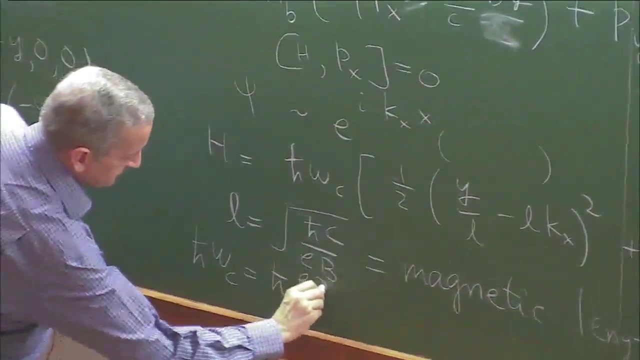 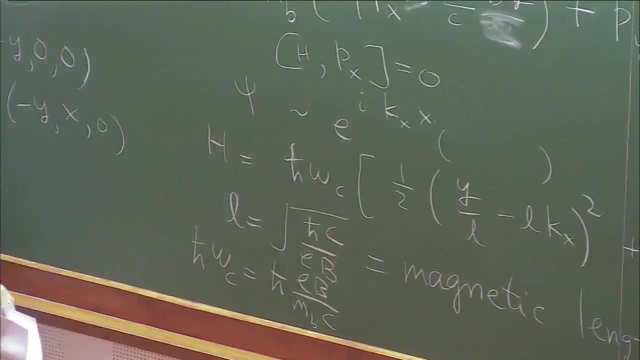 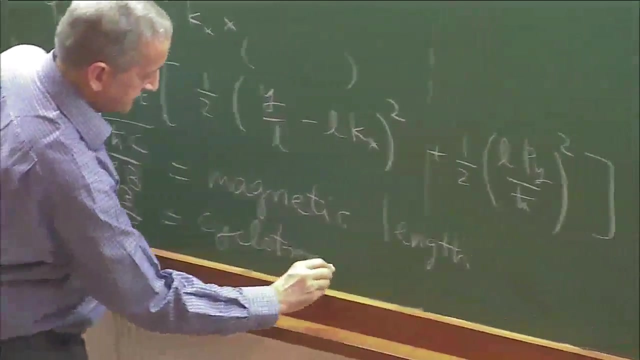 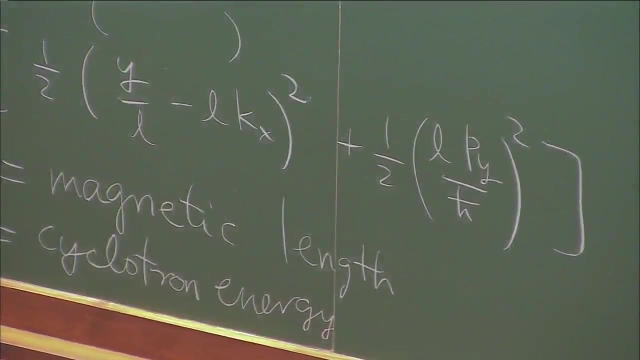 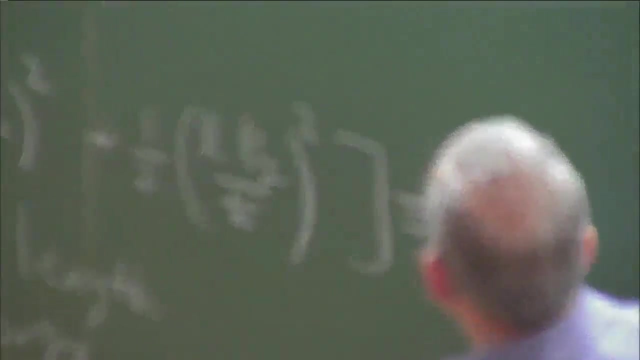 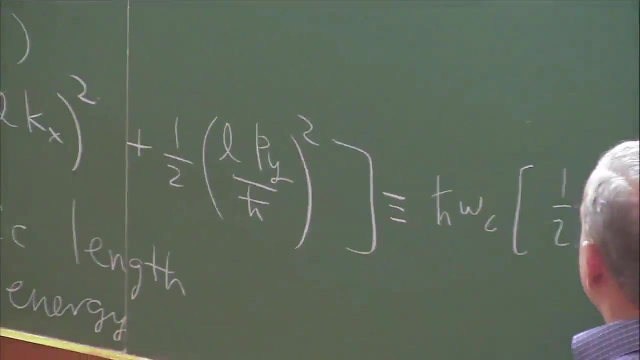 L, which is called the magnetic length, that is. //. Okay, so I can further define this as: h power, omega c, one half y, prime squared plus one. 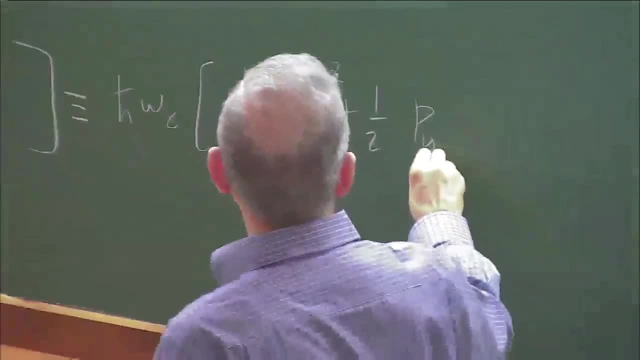 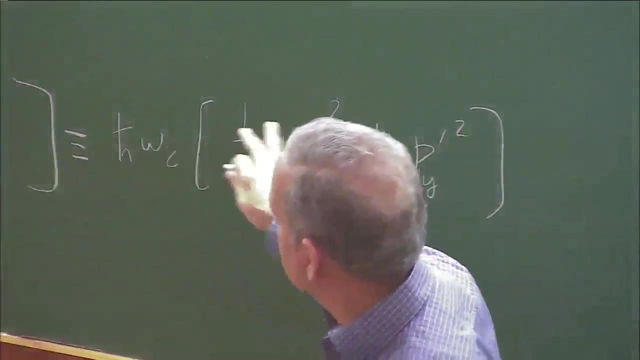 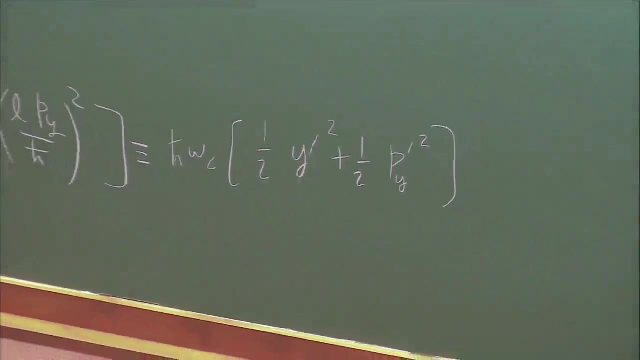 half okay, where the definitions of y prime and py prime you can read off from here. But the main point here is that this looks just like a one dimensional harmonic oscillator. So you could have seen this right in the beginning, because just by looking at this you know that. 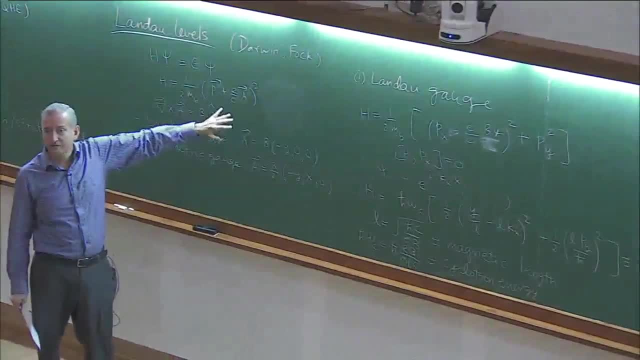 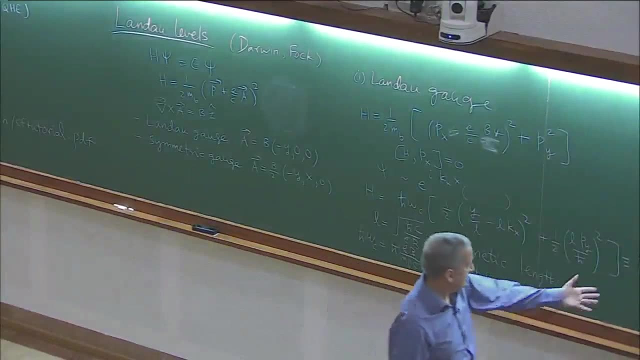 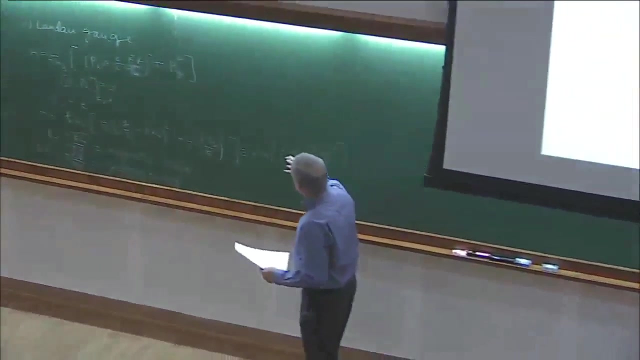 you get things which are at most quadratic in p and x and y. so therefore we can see here that this has the form of a harmonic oscillator, and that thing comes out very clearly here. So we can write down the solution to this. I will assume that you know that the solutions 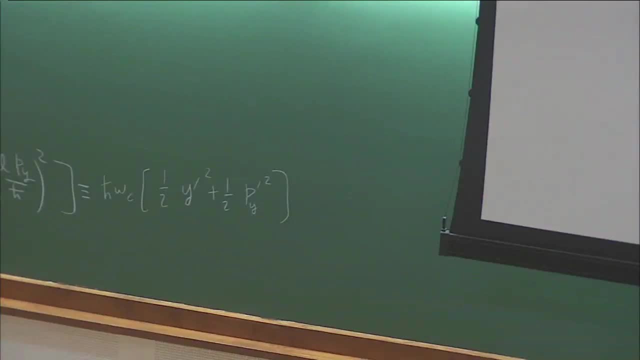 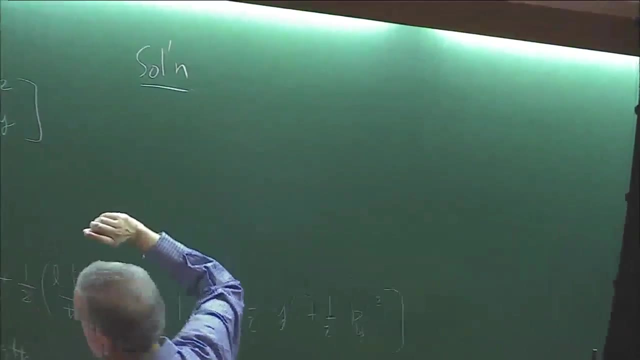 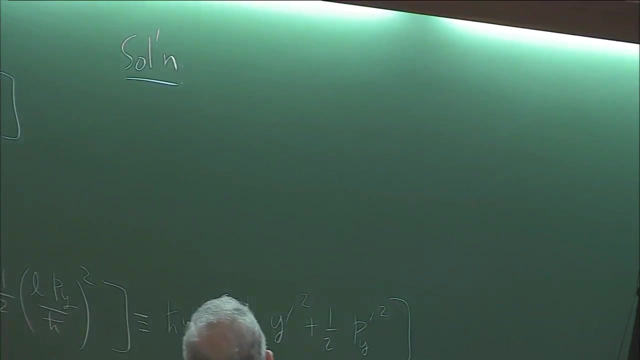 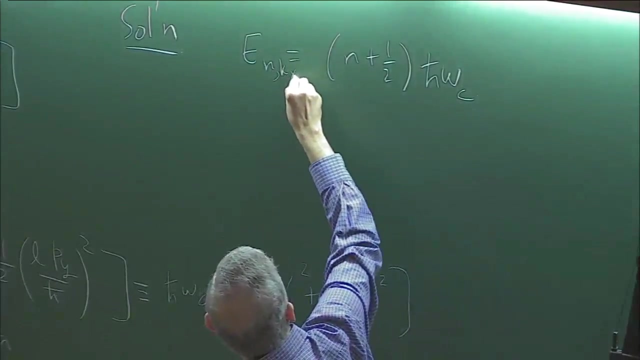 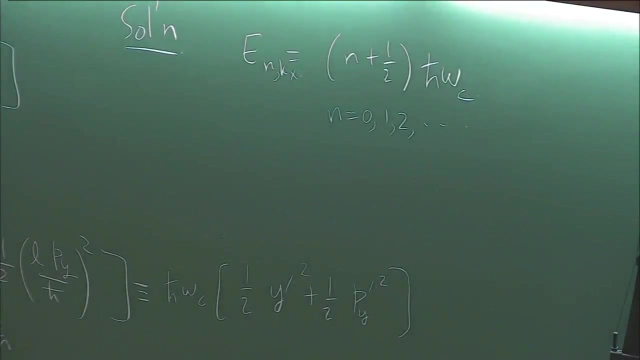 of a harmonic oscillator are the harmonic polynomials. So we have the solution to the problem there. the energy eigen values of these are- I will just try to put them into this: Okay, so the energy eigen values have this form. this is the this equation you should. 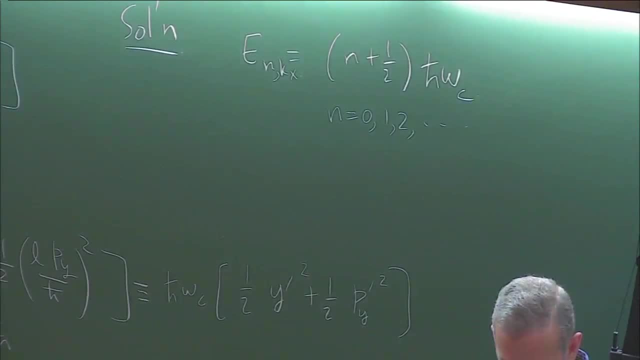 recognize from a single one dimensional harmonic oscillator and the wave function or the eigenfunction and the wave function and this is a. this is a two dimensional harmonic oscillator which is a single dimensional harmonic oscillator. So it's a single dimensional harmonic oscillator and the wave function or the eigen function. 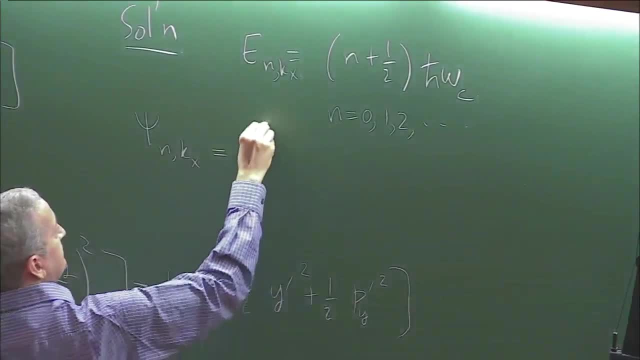 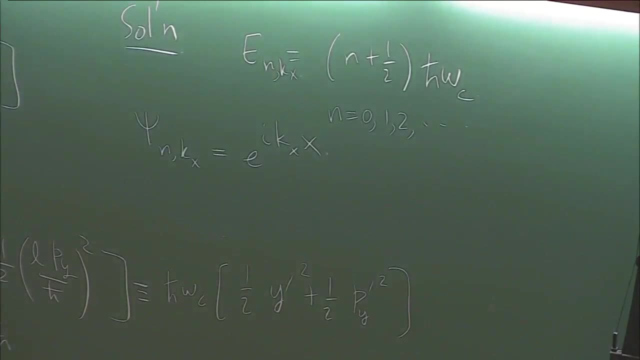 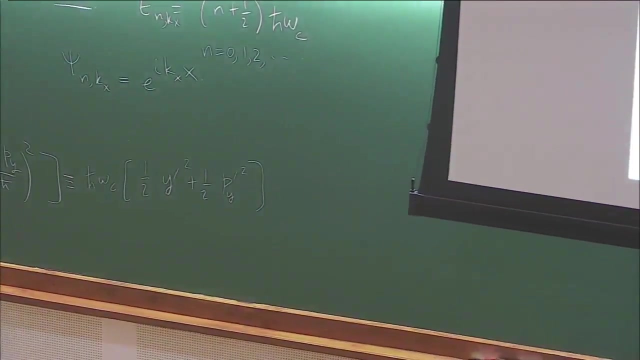 looks like this. so this part we had already discovered here. now we know the part that depends on the y coordinate. is there a way I can pull this up? I don't need this anymore and I can also. we can also remove this. 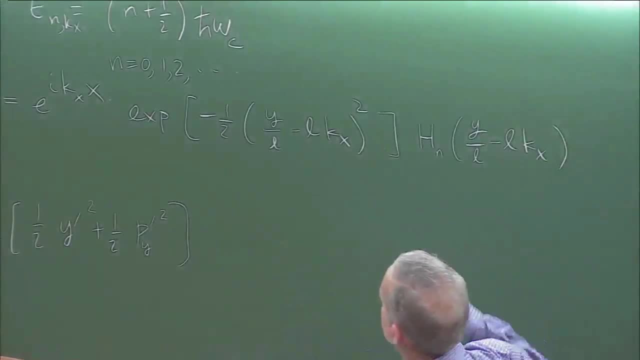 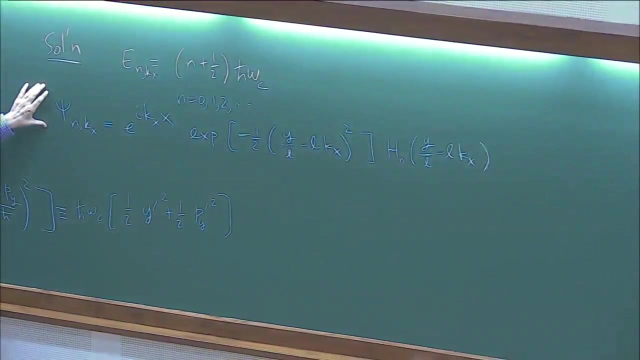 So this is the full solution, apart from normalizing factors. okay, so if you look at this, a couple of things are pretty noticeable. first of all, the energy does not depend on the wave vector tx, you know. so typically we are used to thinking of energy as the wave vector tx. 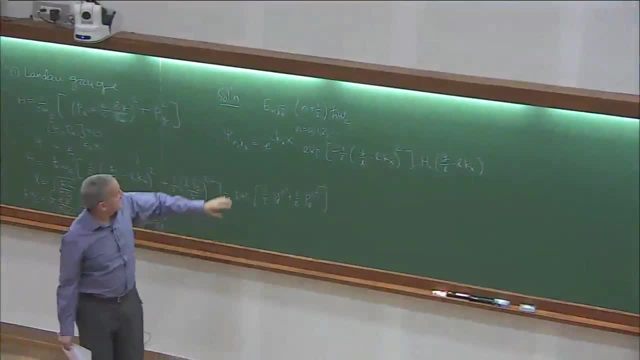 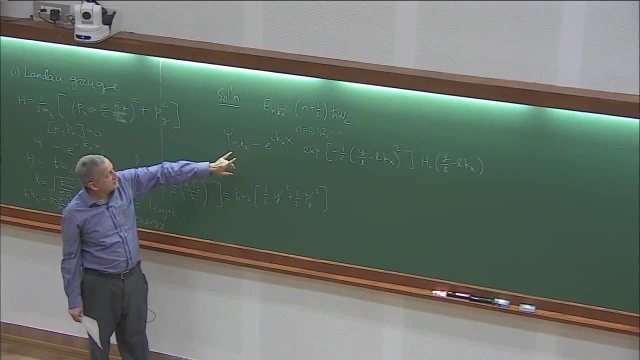 you know, so typically we are used to thinking of energy as the wave vector tx. you know so typically we are used to thinking of energy as depending on tx and ky. in this case, the energy is completely independent of tx. moreover, you find that the position of the wave function 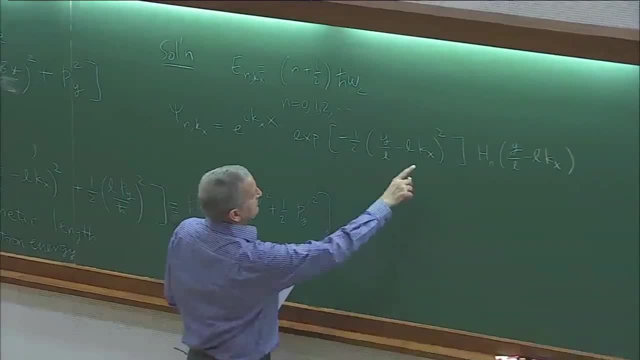 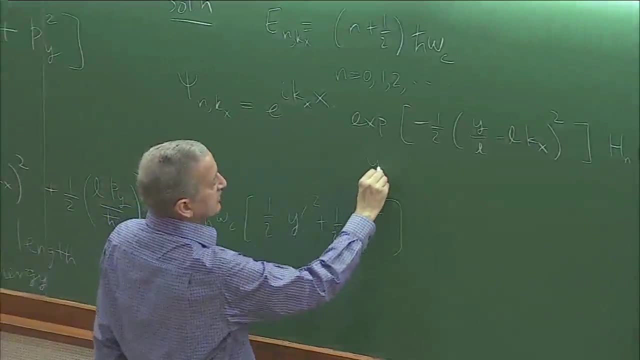 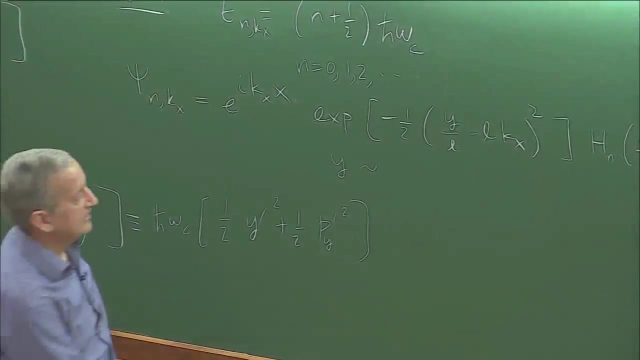 depends on tx, because there is this Gaussian factor. and from this Gaussian factor, if I fix the value of tx, then we know that it's localized somewhere where the argument of the exponential is zero, And that is when y is equal to kx L square. so these wave functions look like this. let's: 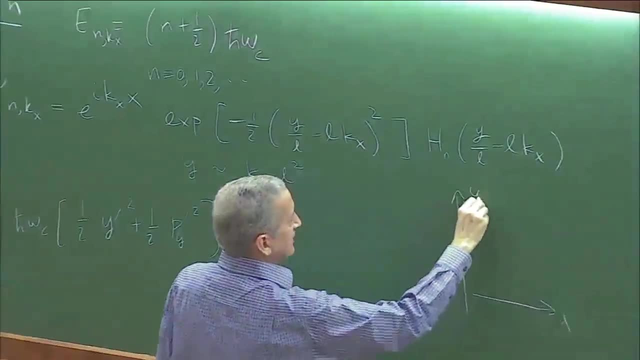 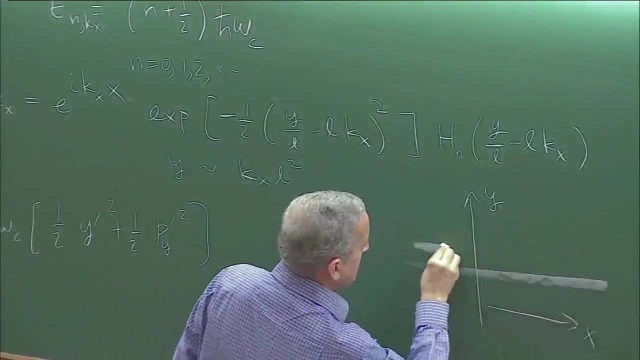 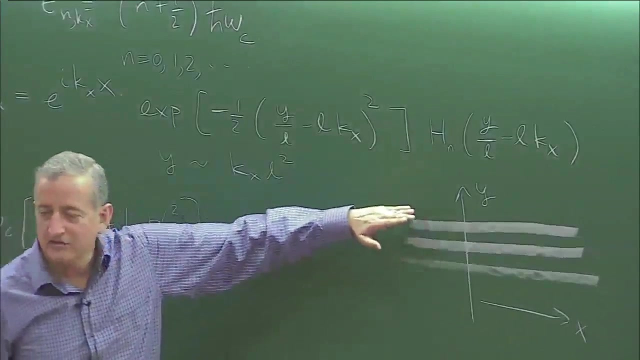 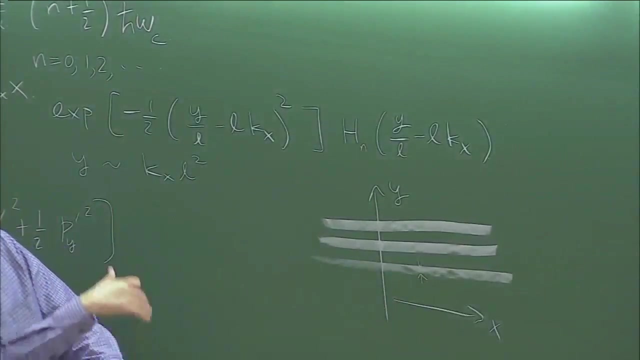 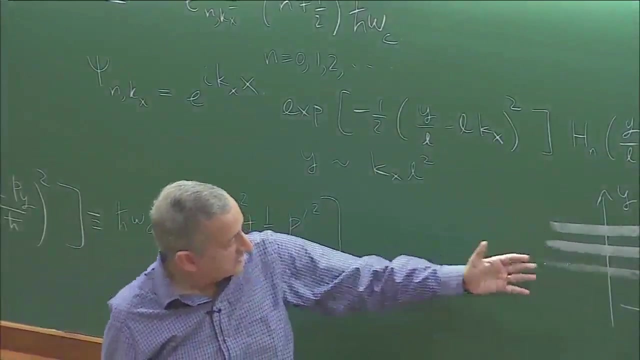 say this is x direction, this is the y direction, then they are strongly localized along lines like this. So these wave functions depend on kx and the extent in the along the y direction. it's roughly equal to a magnetic length. so these wave functions are like lines, the positions. 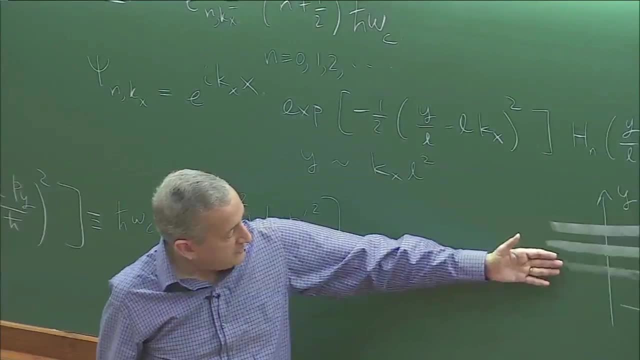 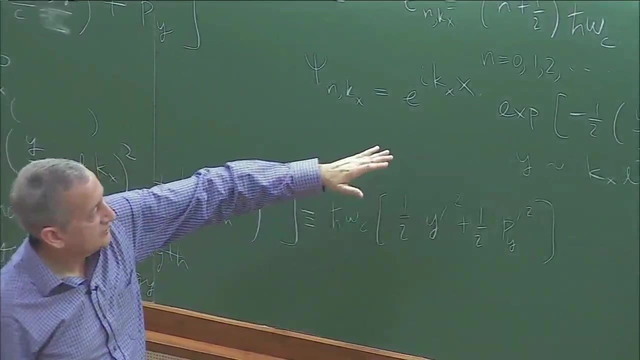 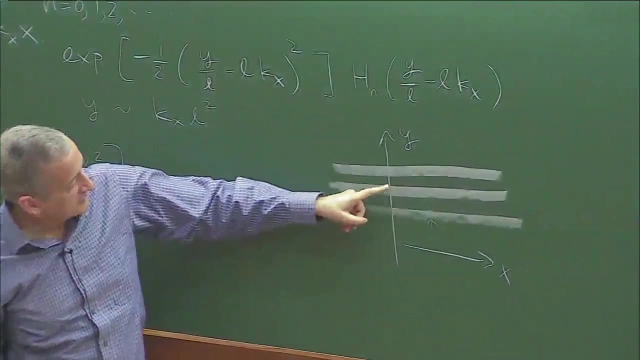 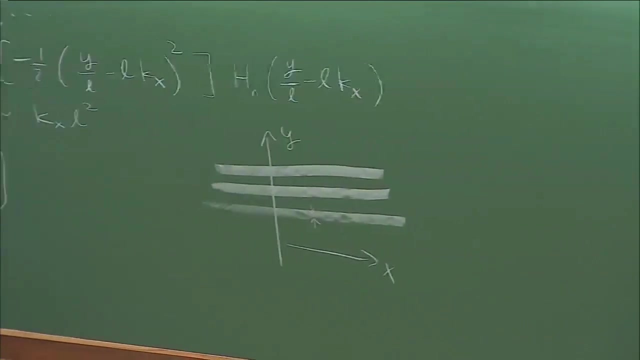 of which depends on kx, but the energy is independent of kx. so for each lambda level you have wave functions looking like this: The form of the wave function, the form factor in the y direction, depends on which lambda level you are at, and that's given precisely by this Hermite polynomial. 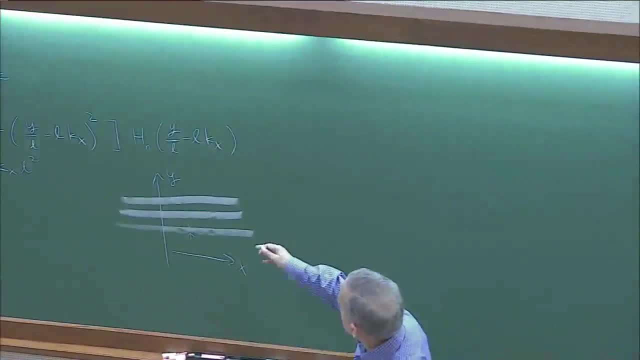 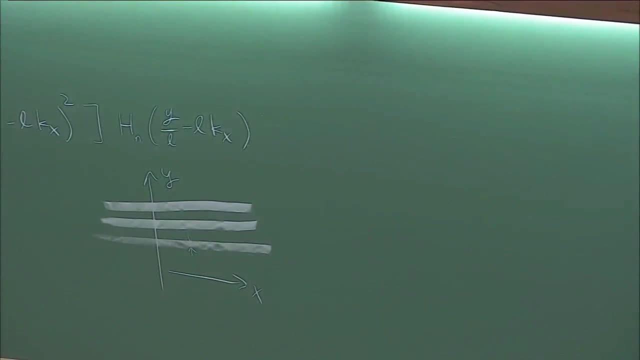 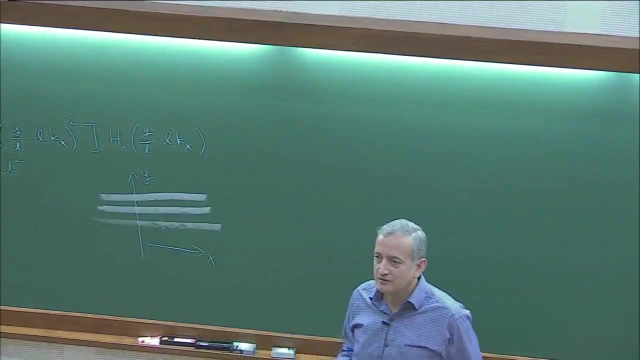 One more thing that we'll need is so here I just drew three lines. you can ask how many different. what's the degeneracy of a given lambda level? Okay, So how many electrons can we put in a given lambda level? well, that's equal to the number. 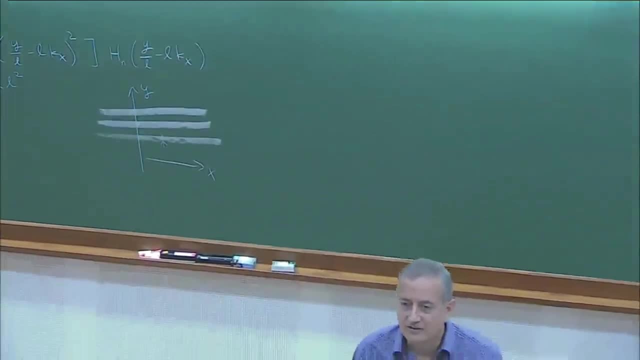 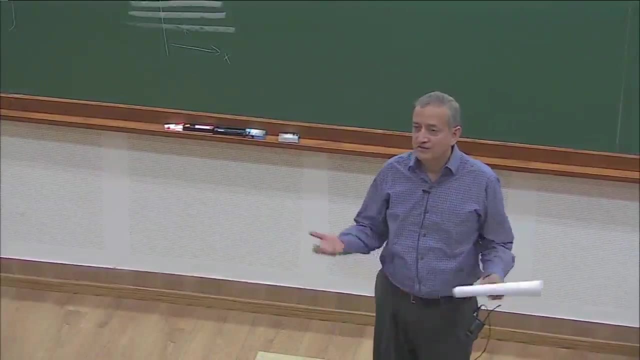 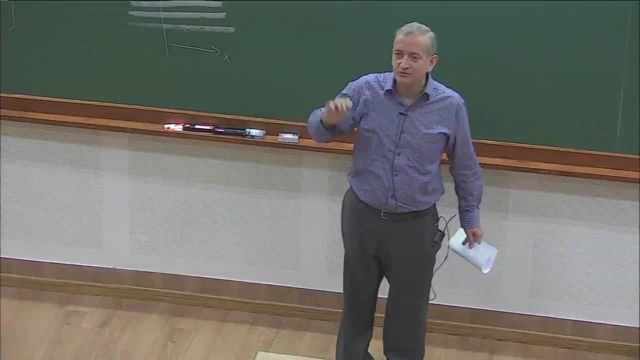 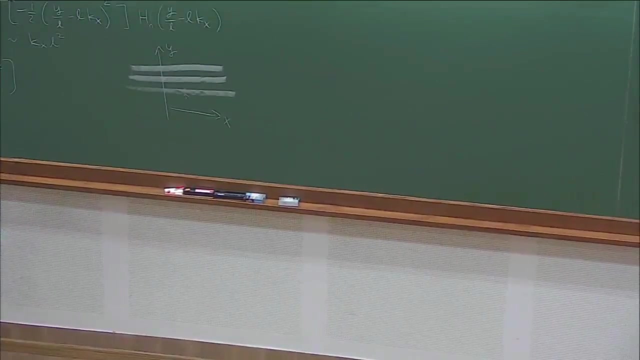 of. okay, how do we determine the degeneracy number of kx values? good, so we have to ask how many different kx values are allowed within a given lambda level, and the simplest way to do that The problem is to assume periodic boundary conditions. so if I say my sample goes from: 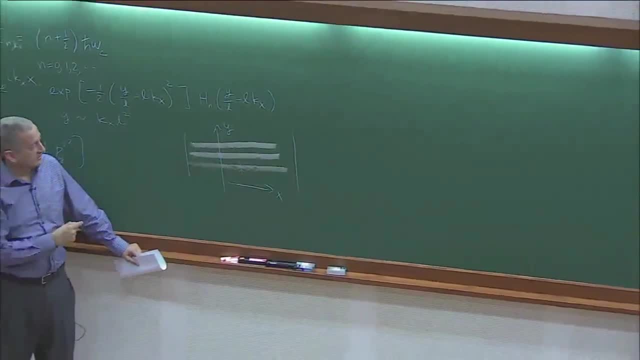 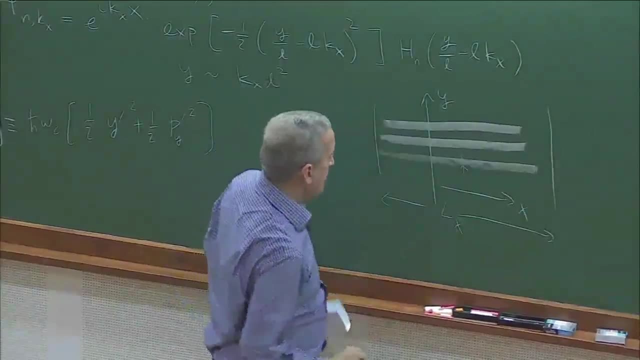 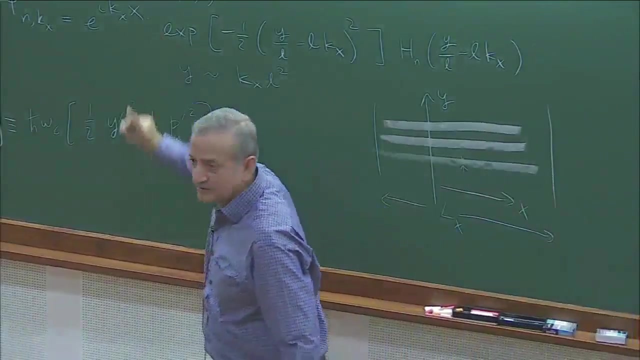 here to here, and I assume periodic boundary conditions. so let's say this length is l or lx? periodic boundary conditions would say that if I change x by an amount which is equal to lx, then the wave function remains unchanged. So that means e to the power of kx. 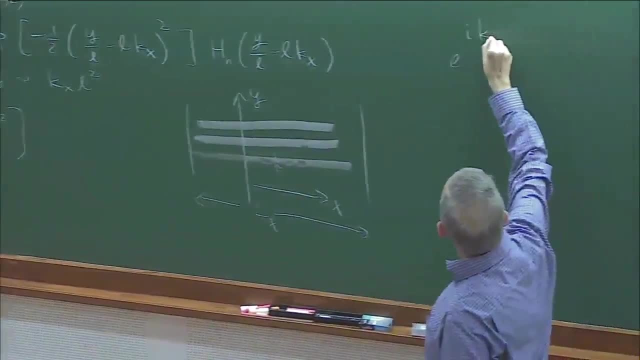 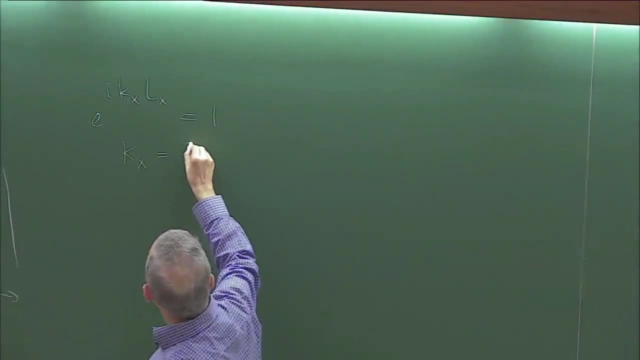 Okay, Okay, Okay, Okay. So for an equation of type 2, the wave function is equal to, in terms of y, kx, lx is equal to 1, so that gives me kx equals to 2, ni over lx. 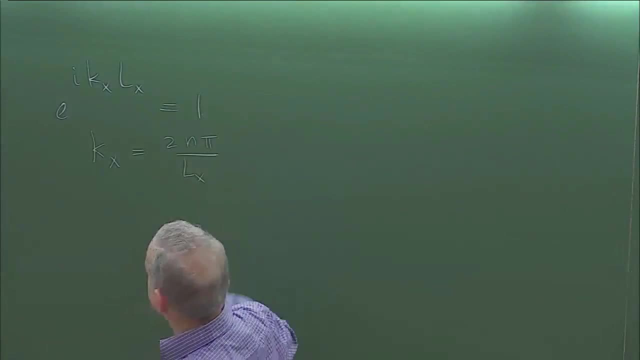 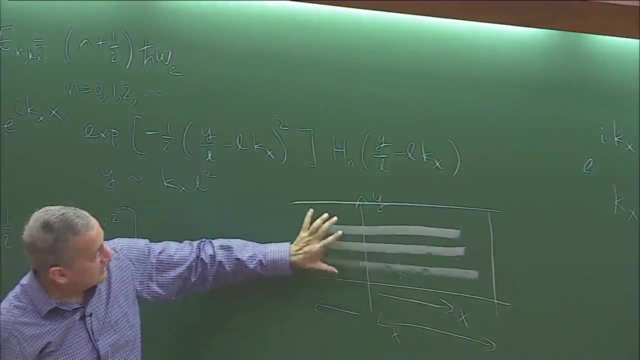 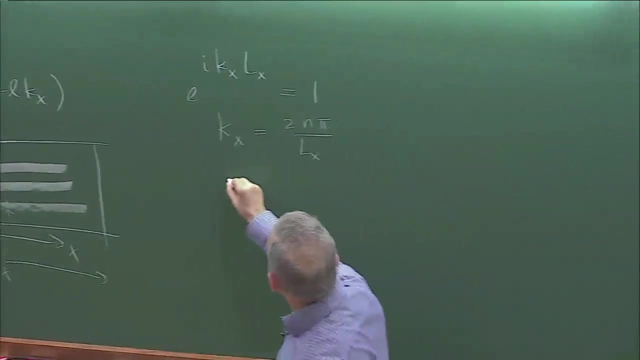 So this gives us discrete values of kx for this system. the second thing we can do is we can ask in sum, over time, over some length in the y direction, how many of these discrete kx values fall, and that will tell me how many different states I have within this region. so let us take n going. 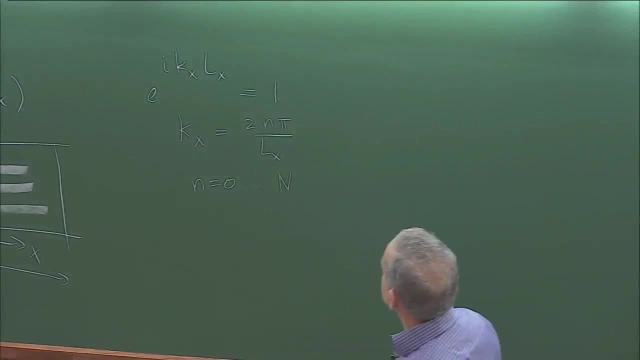 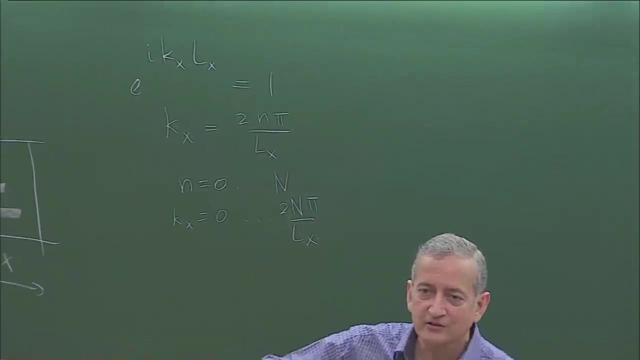 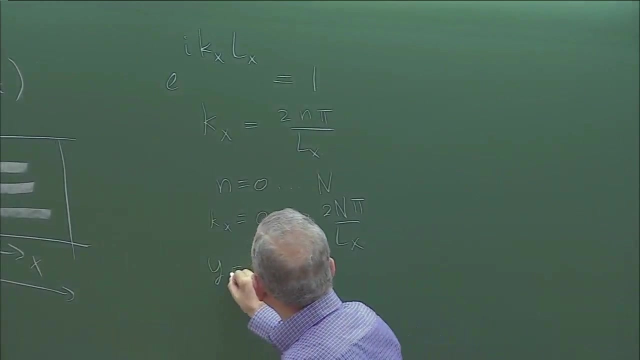 from 0 to, let us say, some capital N. kx will go from 0 to now. remember: kx tells me where the wave function is located. this means that y goes from 0 to a value. I am going to use a value of kx. 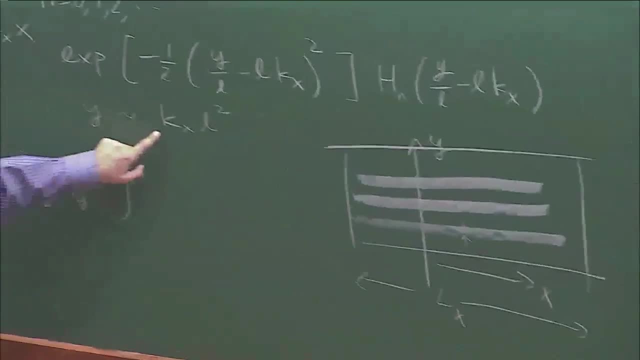 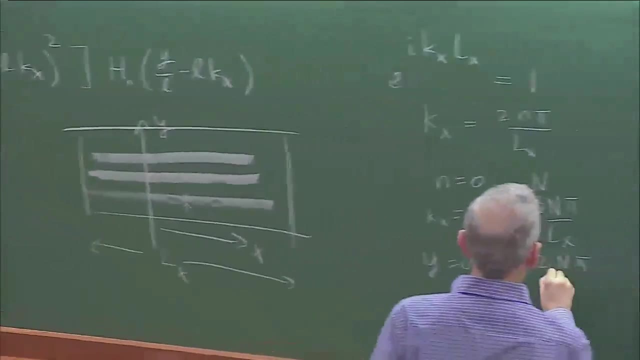 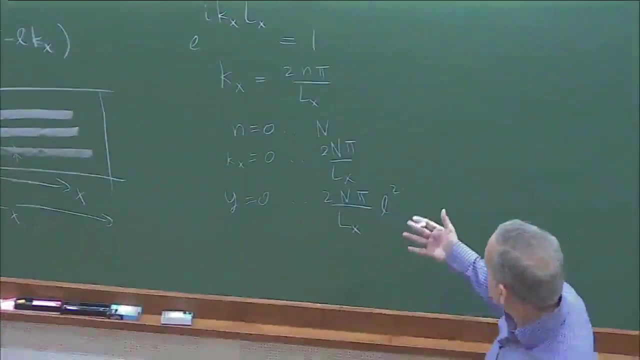 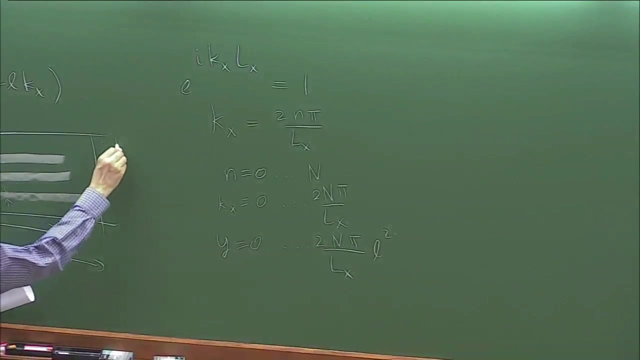 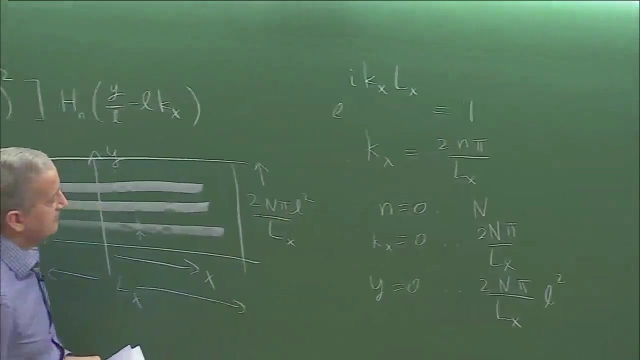 So what is kx? is this formula here: kx is 2n pi over lx. so what this tells me is that if I take length equal to lx in this direction and this length is 2n pi l squared over lx, then in this rectangle, 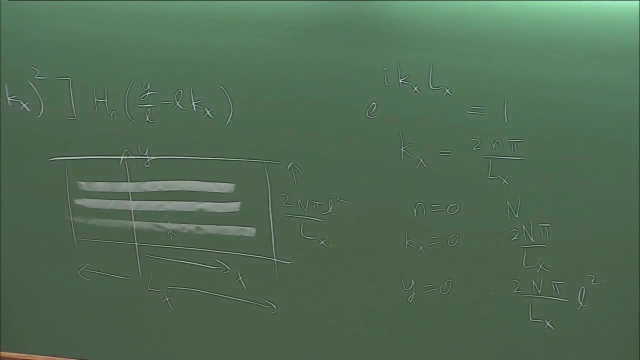 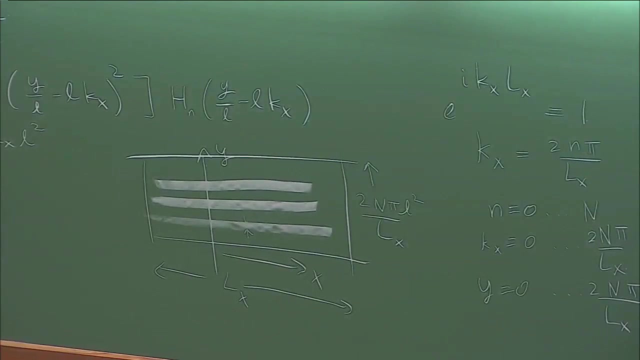 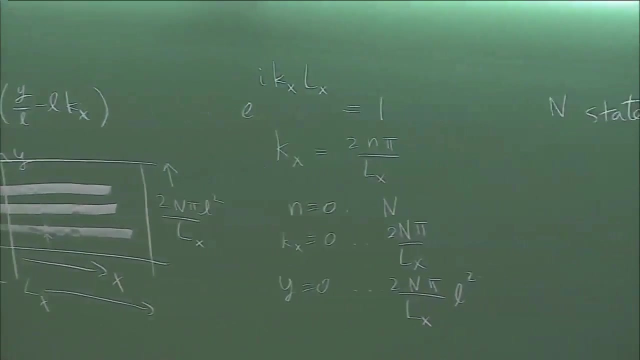 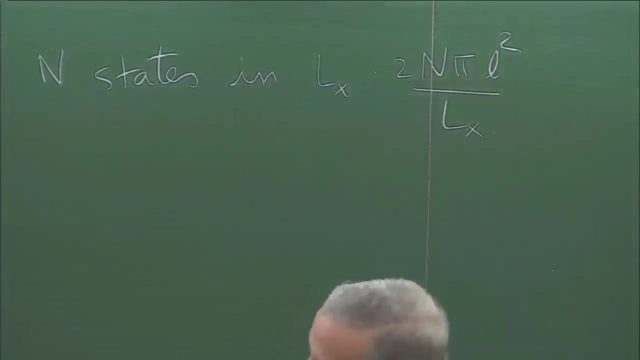 I have n states. in fact I have n plus 1, because I started counting from 0, but we are not worrying about order 1 effects, so I have a capital N states in this rectangle and therefore the So we have. the area of this is lx times 2n, pi, l squared over lx and therefore the degeneracy. 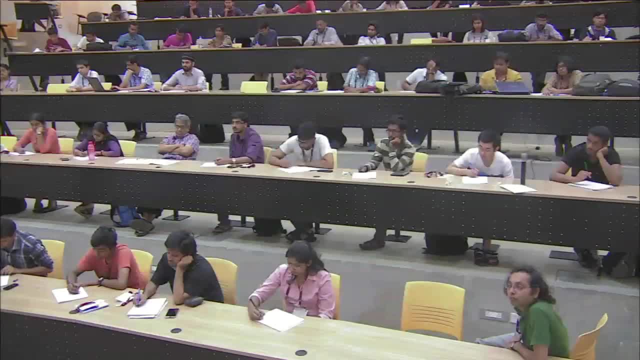 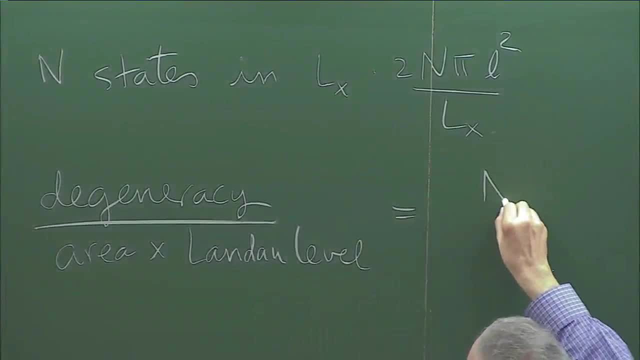 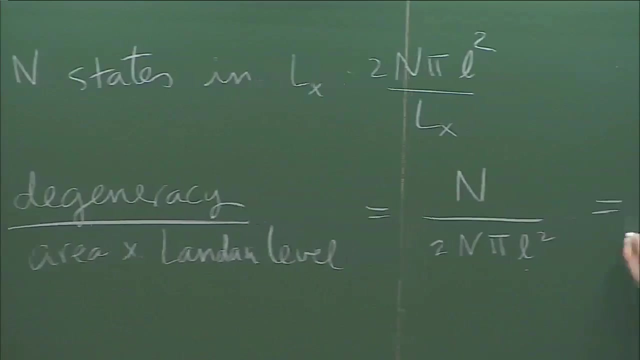 per unit area. So we have the area of. this is lx times 2n pi l squared over lx, and therefore the degeneracy per area or land level is equal to the number of states divided by the area. so that is 2n pi l squared. 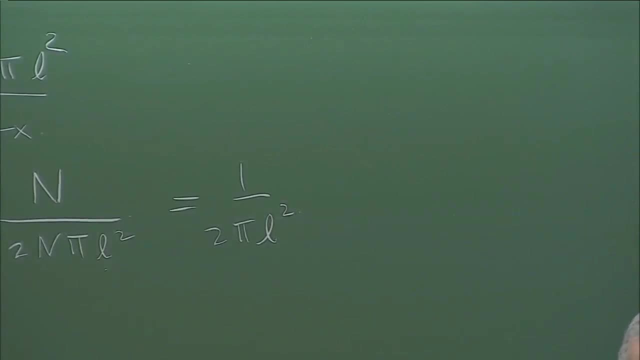 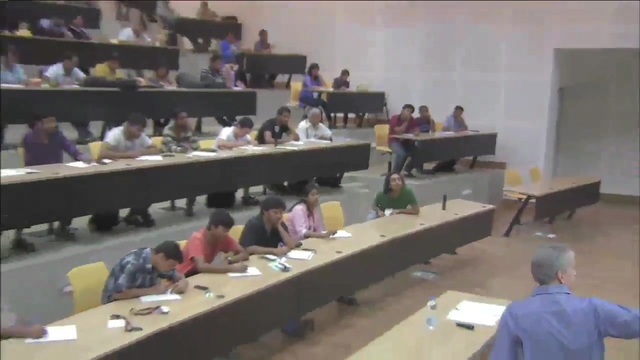 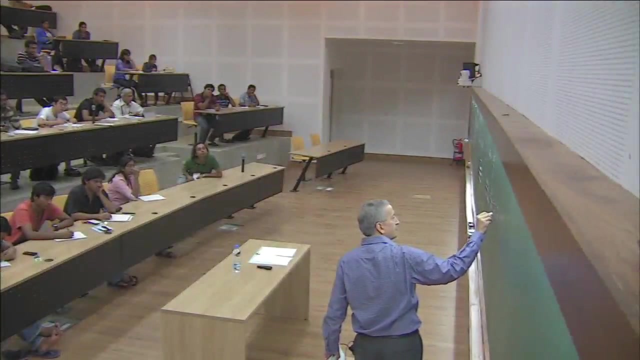 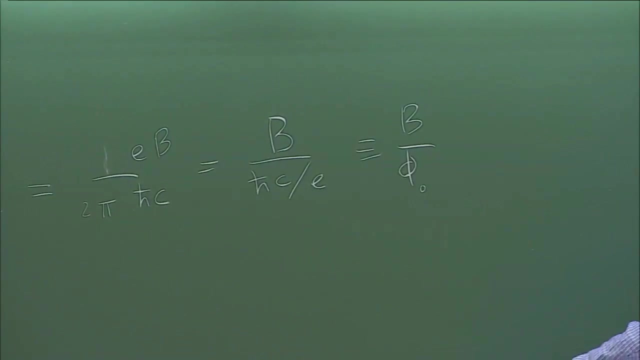 Why? Because Why? Okay, so in a unit area, in each lander level, I have this many states. Let's write it out a bit more explicitly. So. So I have defined here phi naught, which is hc over e. 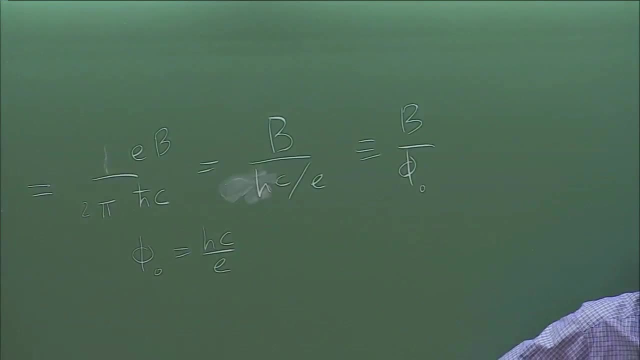 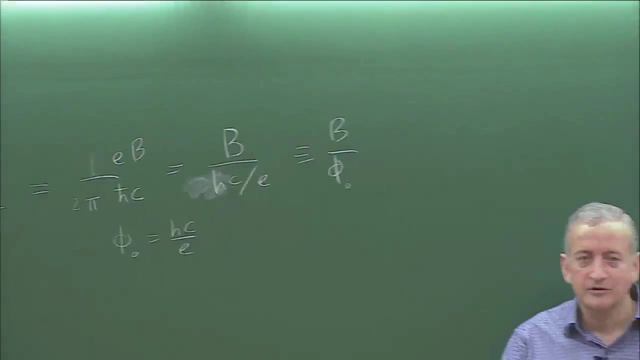 It's often called the flux quantum, although that's a misnomer, because flux is not quantized. You can produce any flux you want in the laboratory, But this is known as flux quantum. hc over e And what this tells me? So this is the flux through a unit area divided by flux quantum. so it tells me that the number 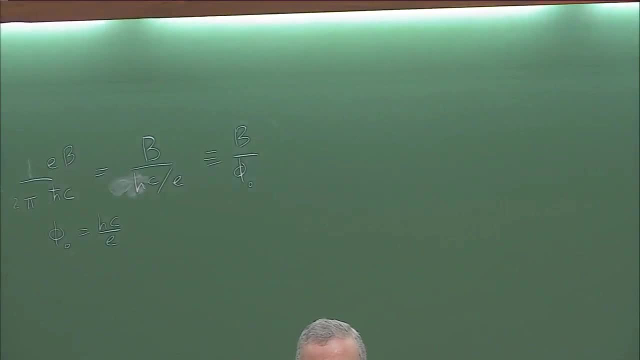 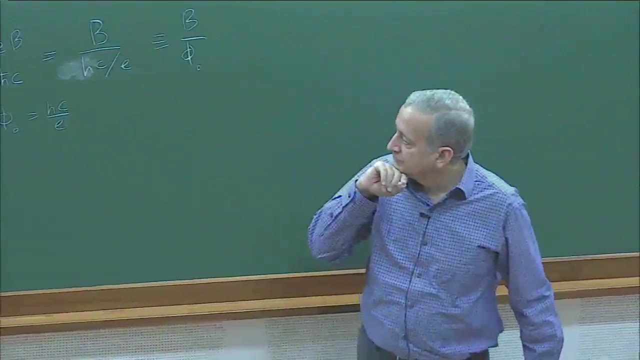 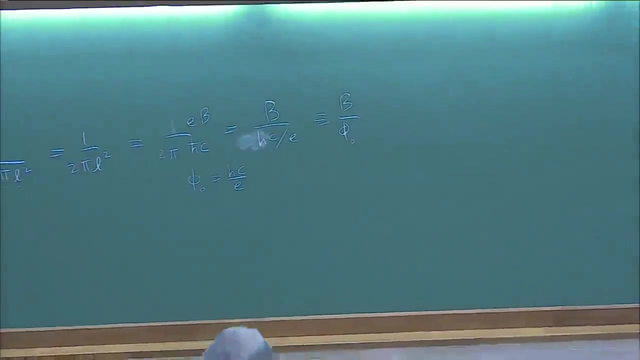 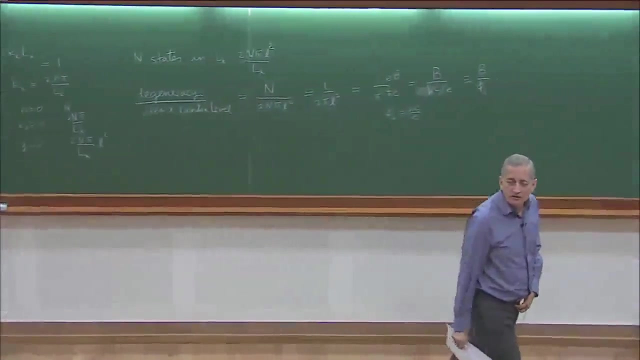 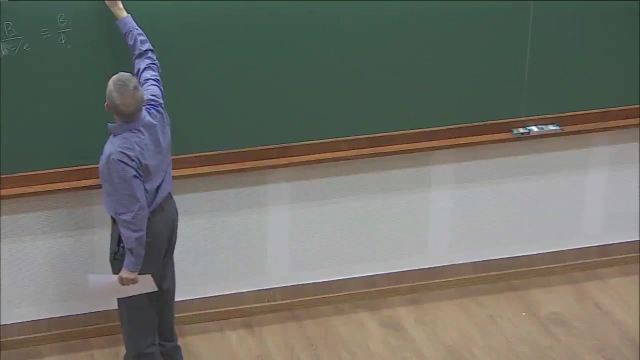 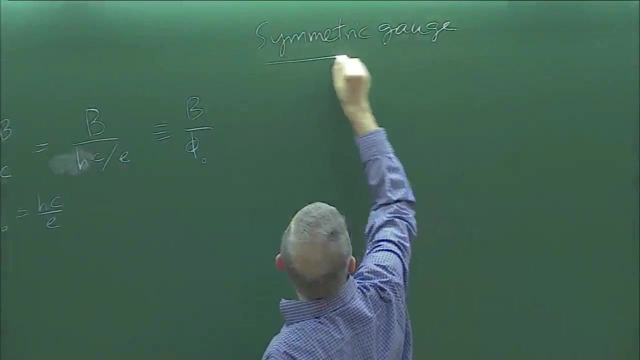 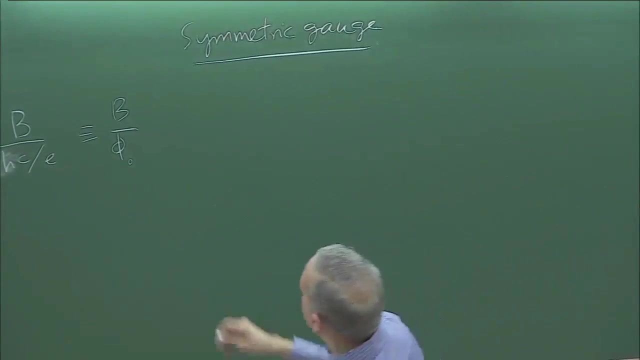 of states in each lambda level is equal to the number of flux quanta penetrating the sample. Any questions on this? Let us quickly do this symmetric gate. So here I am going to simplify my life by setting L equals 1, and h power. omega c is. 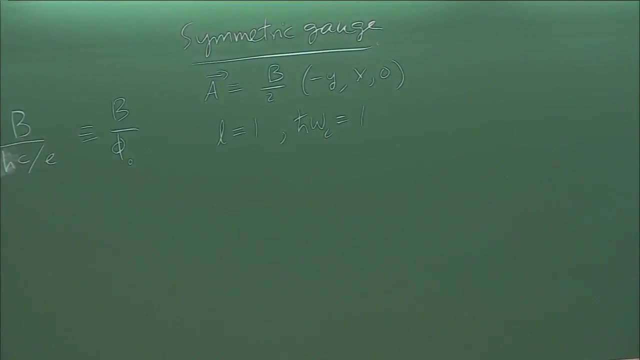 equal to 1.. You can always use the solution that I have described in my previous class if you have put them back in the final expression, just from dimensional considerations. So with this the Hamiltonian is written by: written as follows, so you can try to solve: 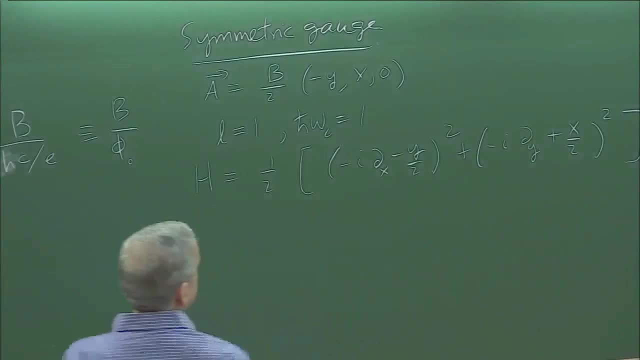 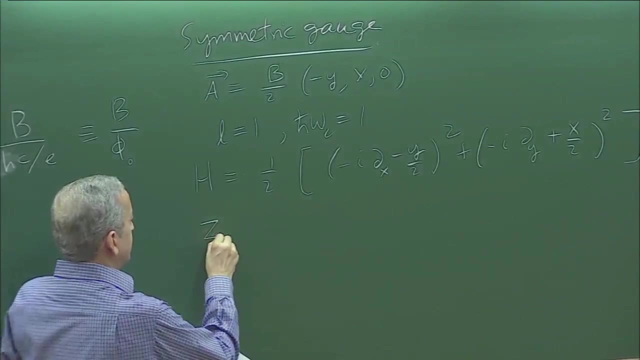 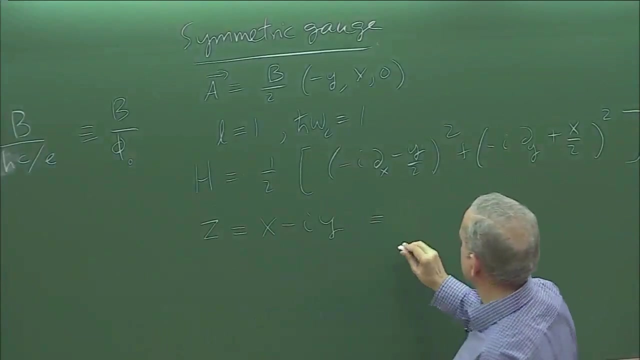 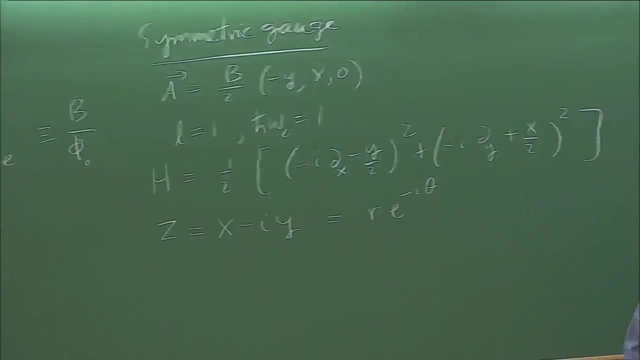 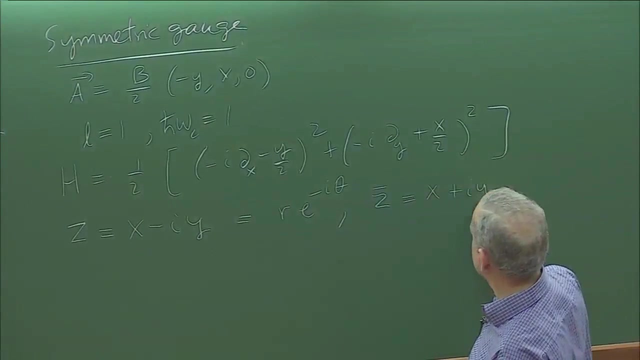 it. but it turns out that this takes a simpler form if I define this quantity. so I have defined a z and I can also define z bar. And you know the fact here that I have to define z as x minus iy, it's you know, just. 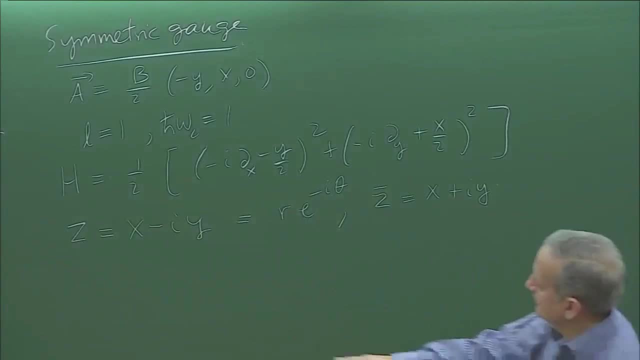 to simplify my life, you know, I could have defined this. I could have defined z as x plus iy, but then I would end up with lots of z bars later on in my formulas. So this is the way we are defining z. Then you can see that I have defined z bar as x minus iy. 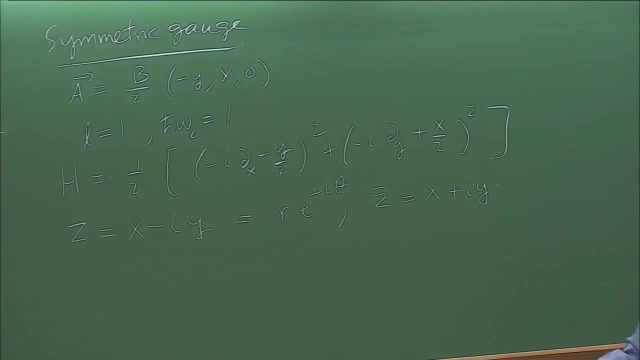 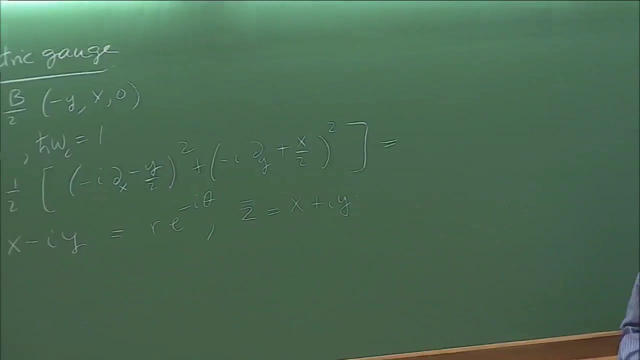 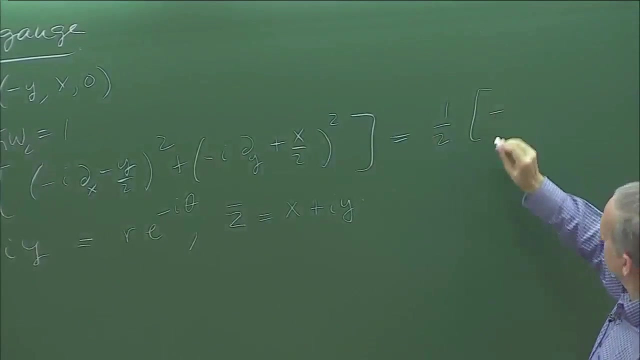 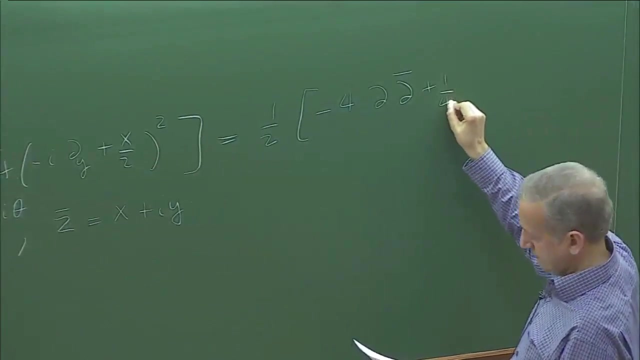 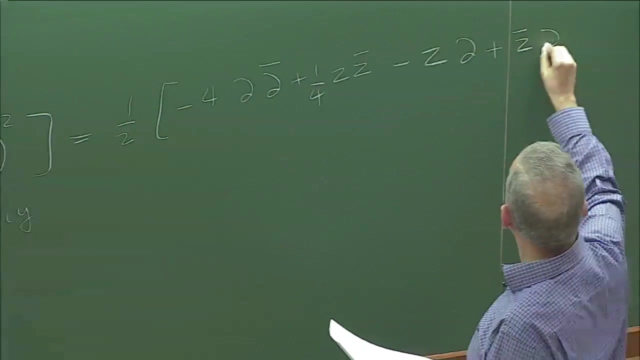 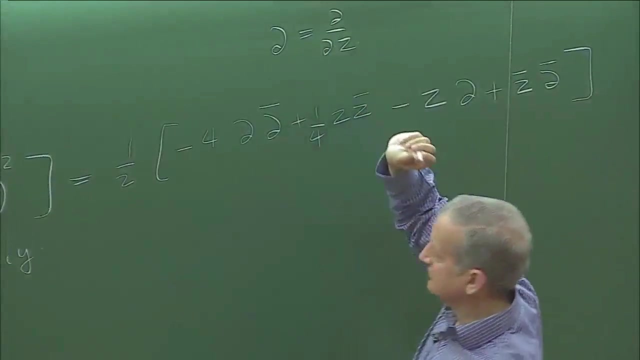 You have to do some algebra, which I'm skipping, but I ask you to do the algebra You can show that this Hamiltonian can be written in this form. So here, when I write del, that means del by del z, z instead of x and y. now I'm working. 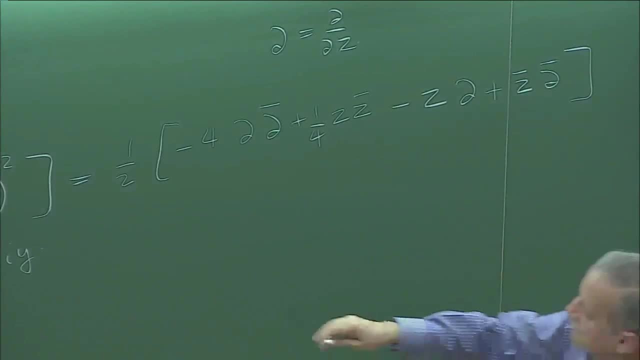 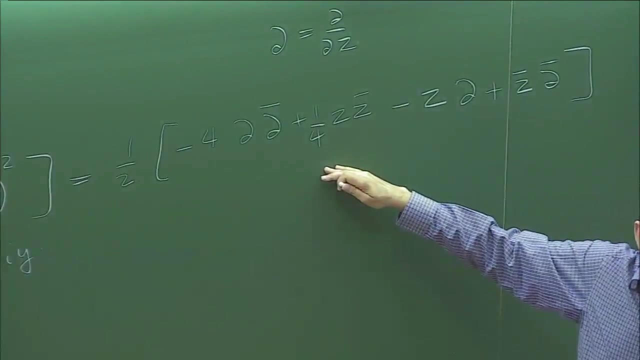 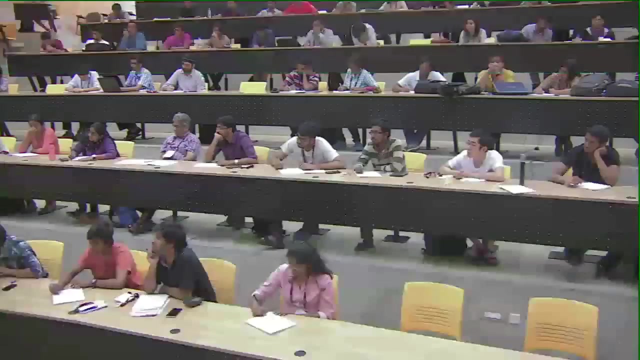 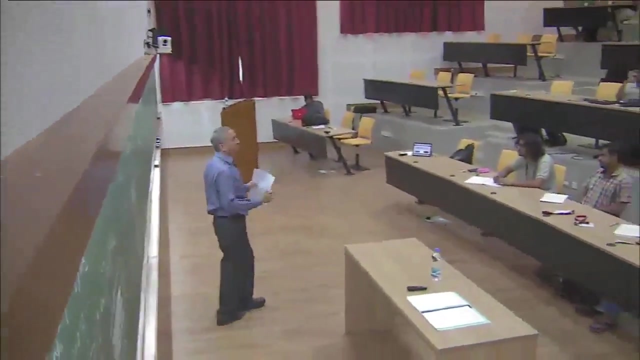 with z and z bar, And please do this algebra so that this can be written in this form. Then we can do some more algebra. So, Okay, Okay, to write it in a much simpler form that brings out the connection with the harmonic oscillator. 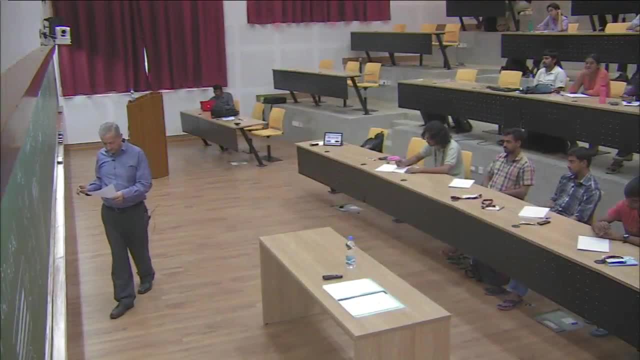 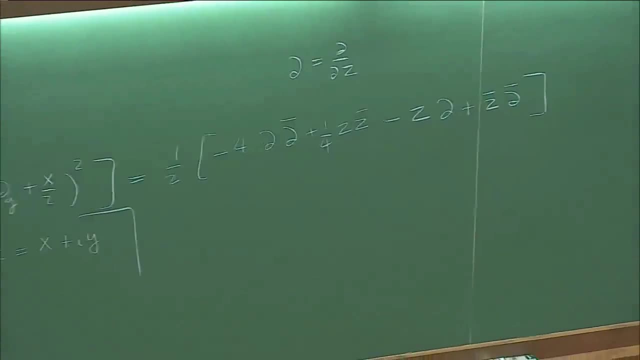 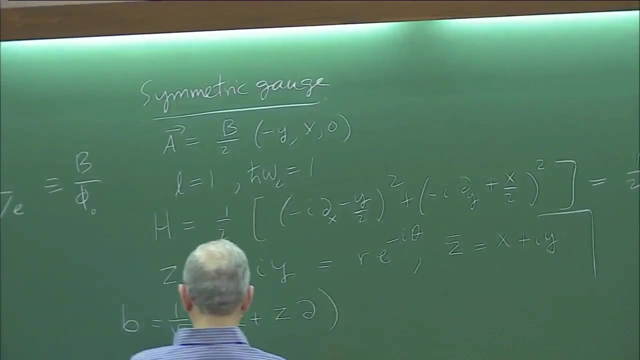 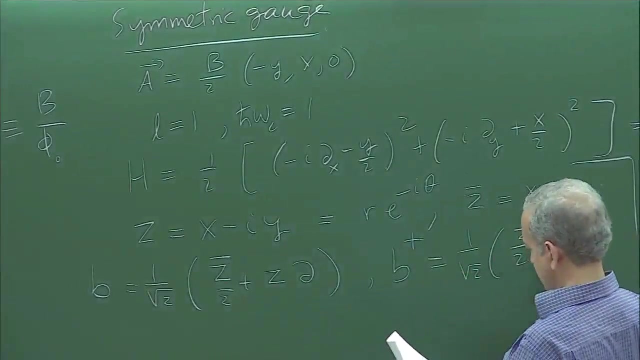 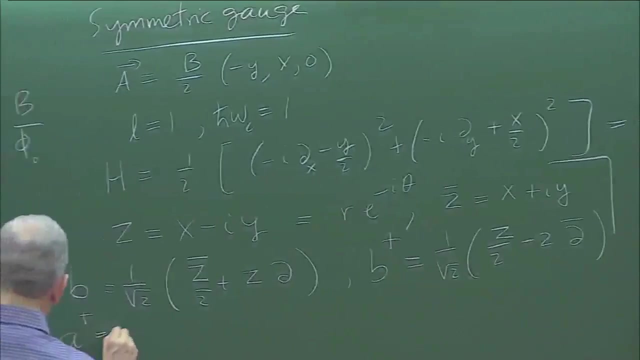 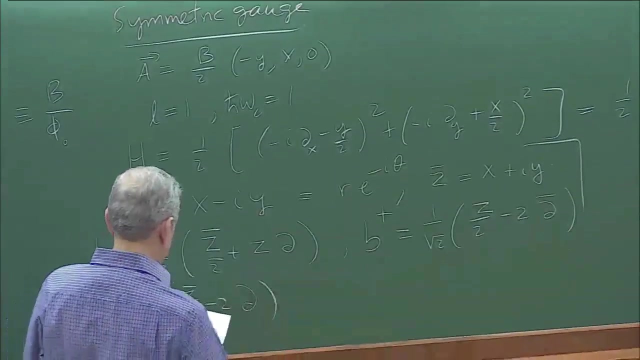 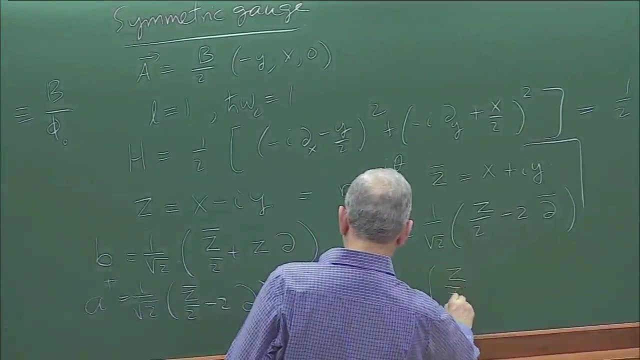 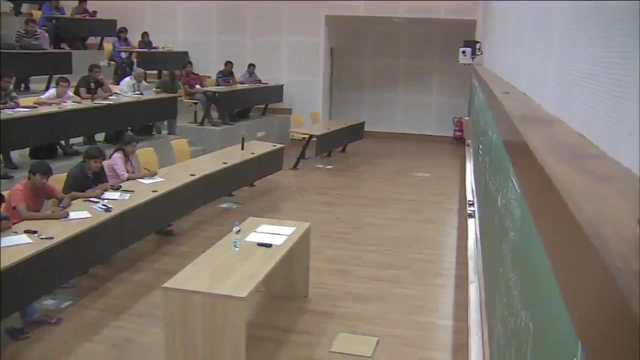 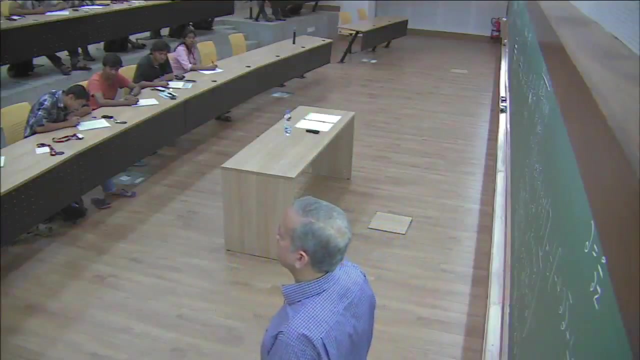 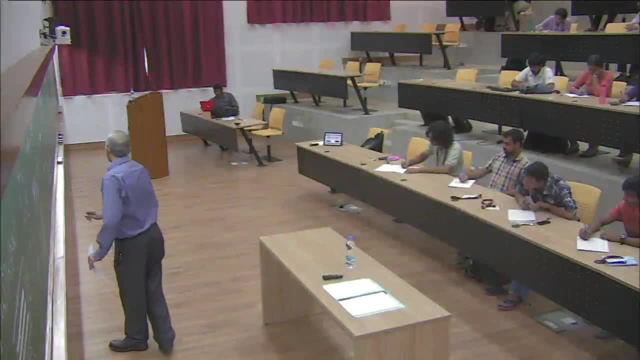 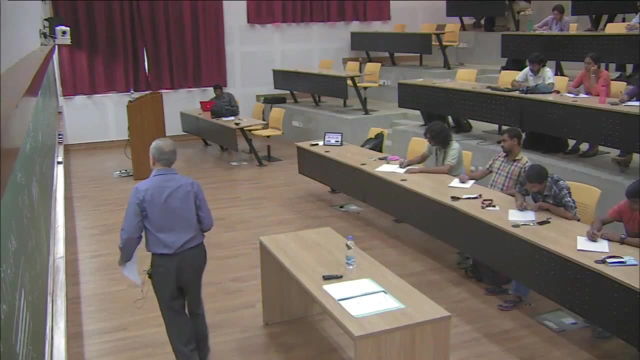 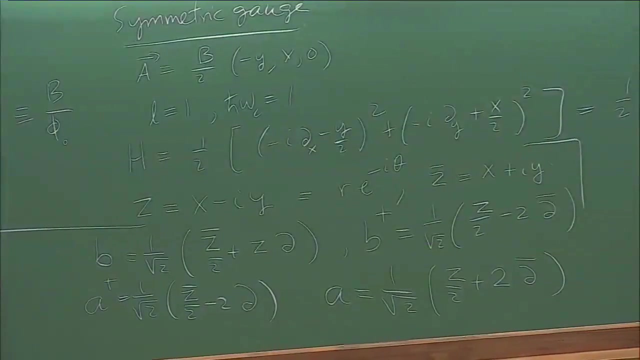 A A dagger. so some of these steps which I am leaving out are part of the tutorial, because it's a good exercise to work these things out, but you should be able to work out that the commutator of B and B dagger. is there a question? 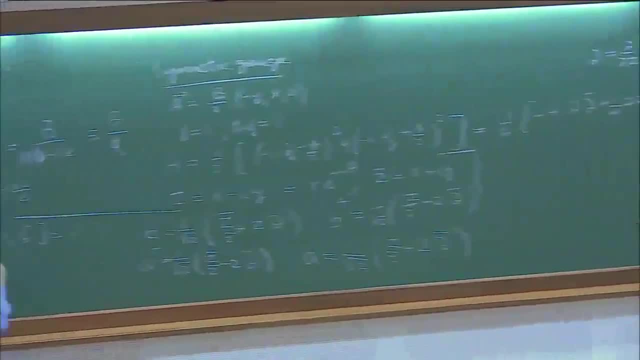 No, is one. the commutator of A A dagger is one, and all of them are commutators of A A dagger. All of them are commutators of A A dagger. All other commutators are zero. 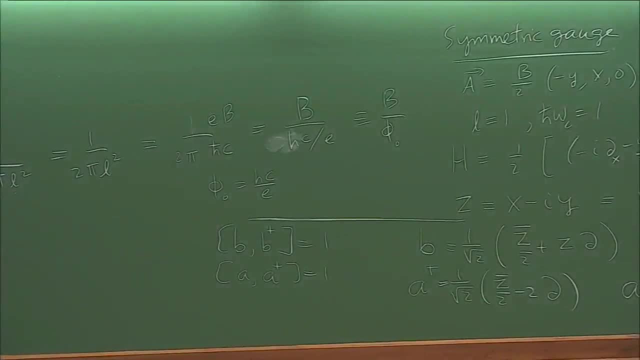 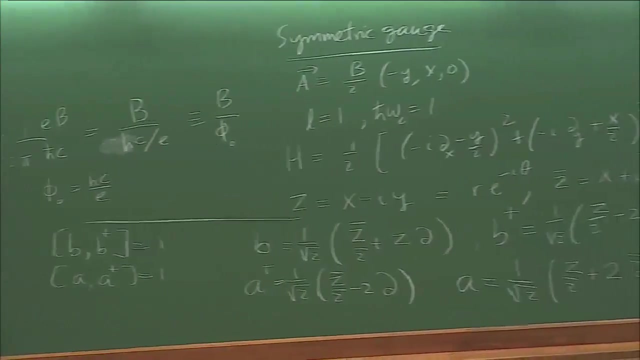 If you calculate the commutator between A, B or A dagger, B, A dagger, B dagger, whatever, they are all zero. So these are the only non-zero commutator. So now, in terms of this, this Hamiltonian will take this very simple form. 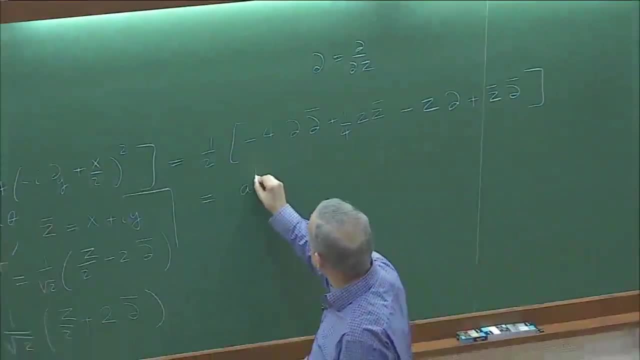 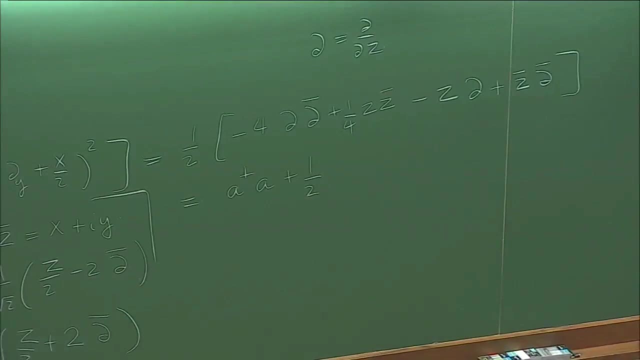 Again, this is some algebra that you should work out, but it's equal to A dagger, A plus a half. Okay, so you can see that this is just like a simple harmonic oscillator: A, A dagger. these are the ladder operators, and we know how to construct all states for a harmonic oscillator. 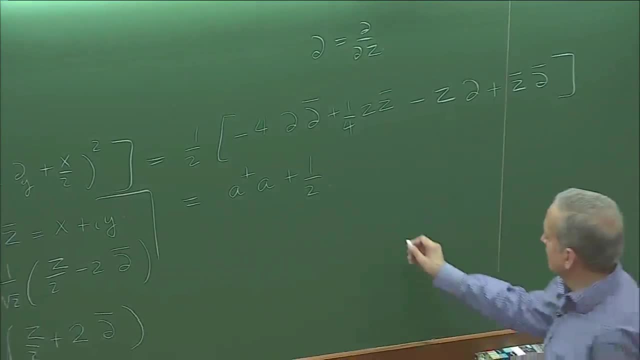 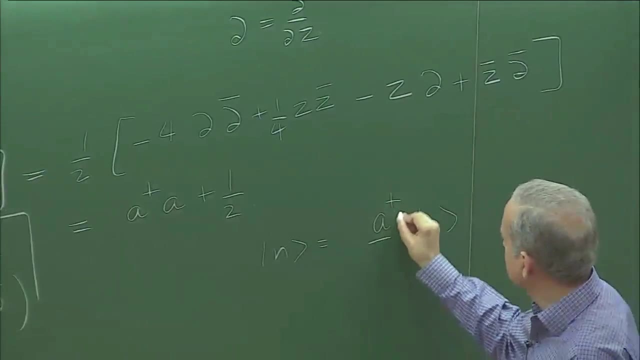 If you had just one harmonic oscillator, then you can construct a single harmonic oscillator. If you had just one harmonic oscillator, then you can construct a single harmonic oscillator. If you had just one harmonic oscillator, then you can construct a single harmonic oscillator. 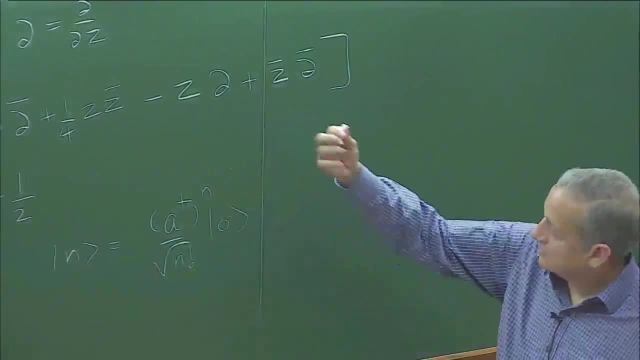 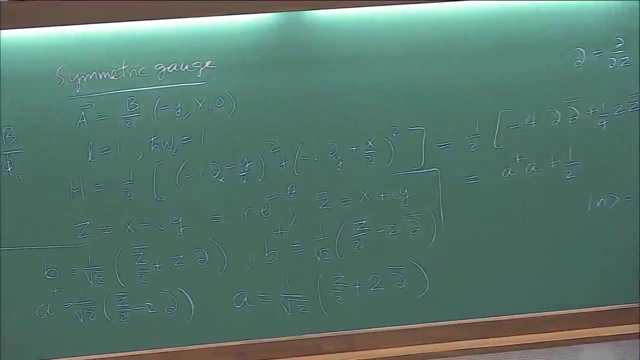 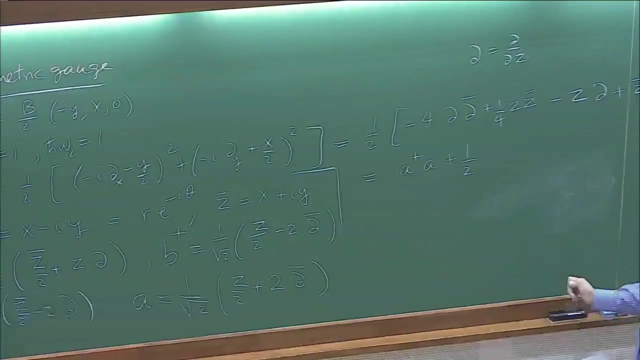 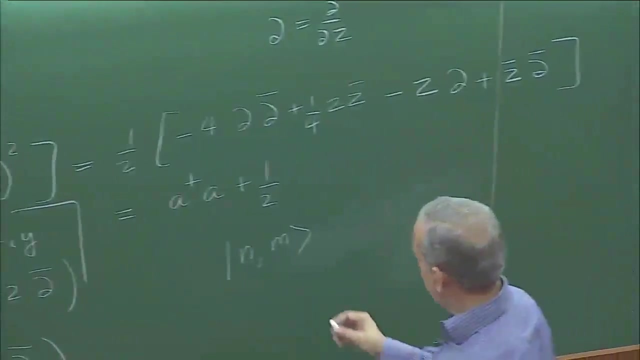 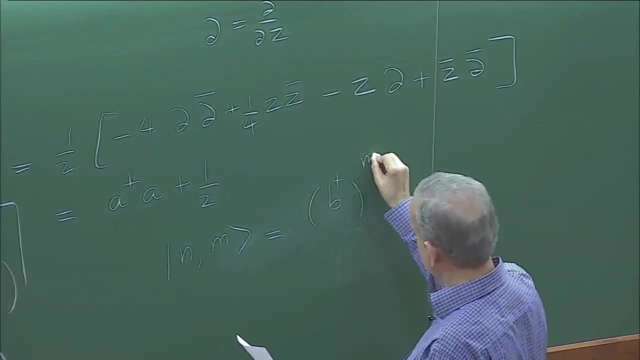 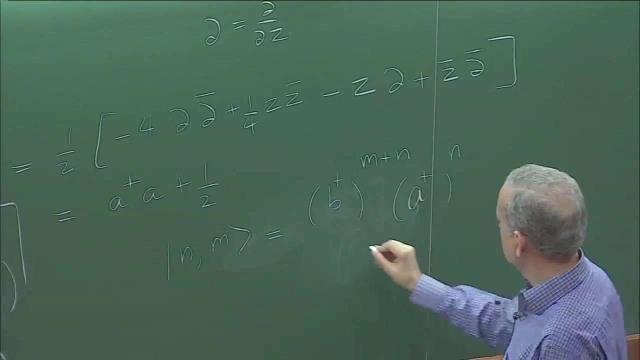 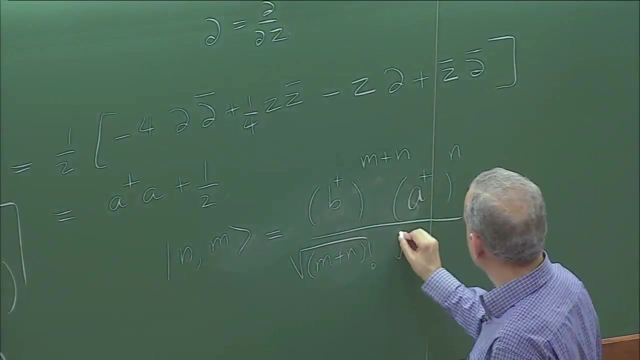 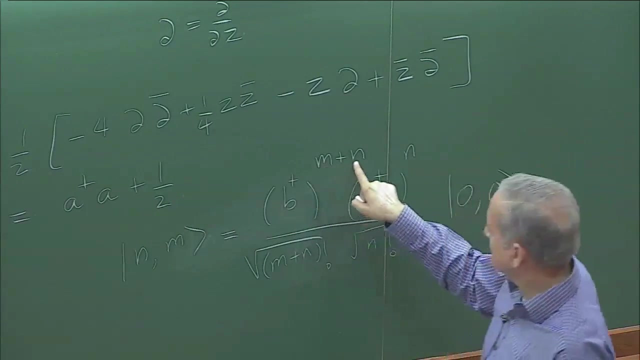 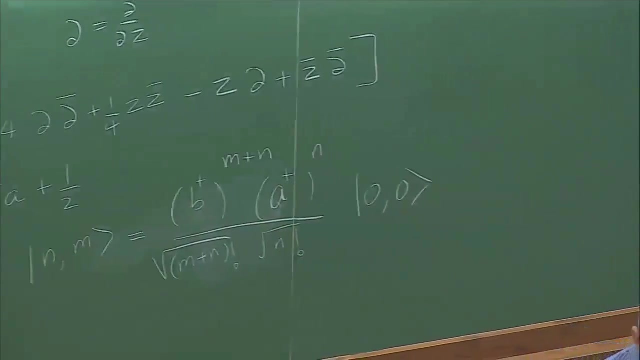 Okay. so I'm going to say that I have two harmonics. We have a and b, So the states would have two integers. They would be labeled by two integers. I will call them n and g. Okay, M, Okay. now it will become clear in a second why I am I mean. so this quantity goes from 0, 1 to 3. so why I have written it in this fashion, I will see in a moment. and the energy. 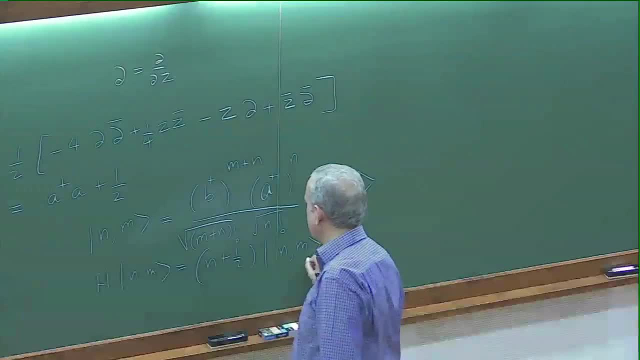 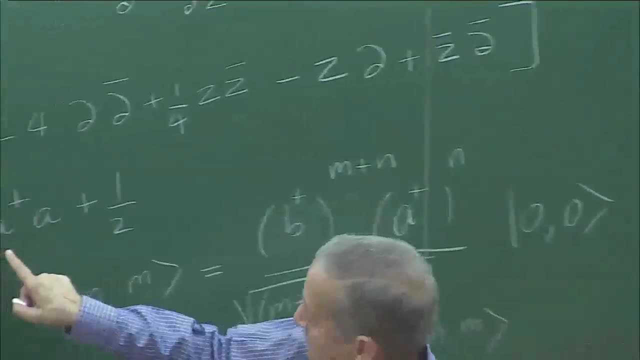 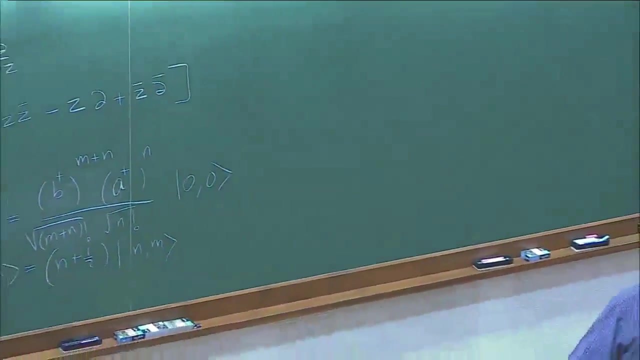 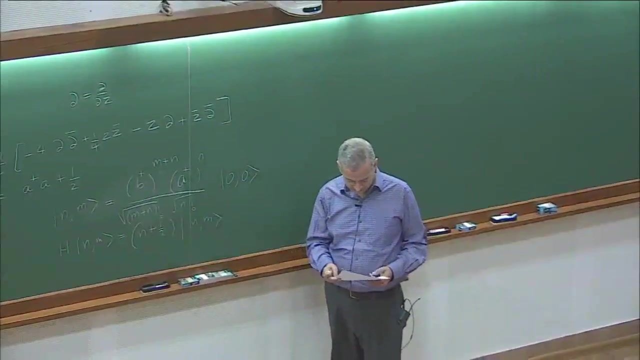 Depends only on n. okay, so remember, this does not contain any b, so in fact it is the b degree of freedom that gives us the degeneracy energy depends only on the n index, which is the lambda level index. Okay, so with this we can actually write wave function. 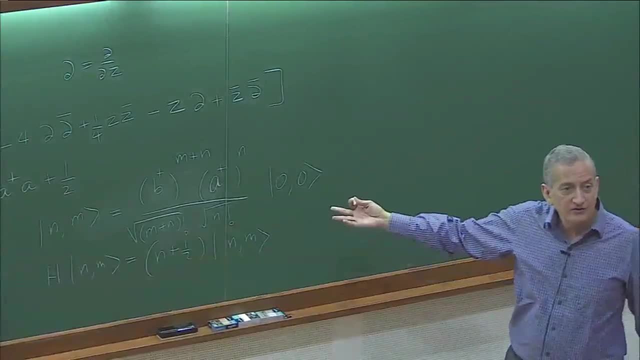 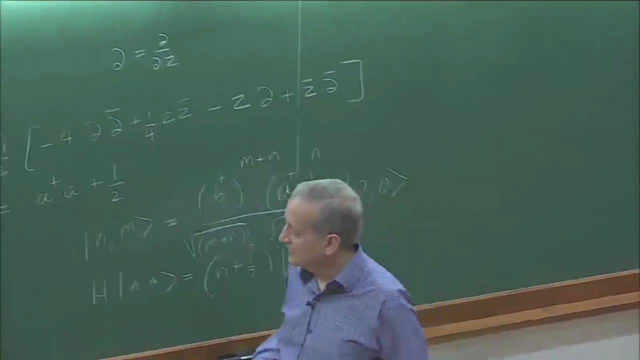 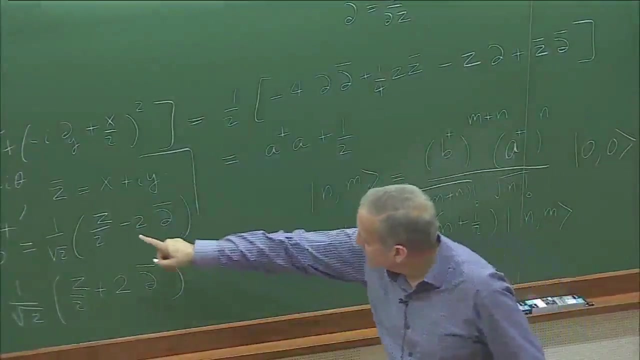 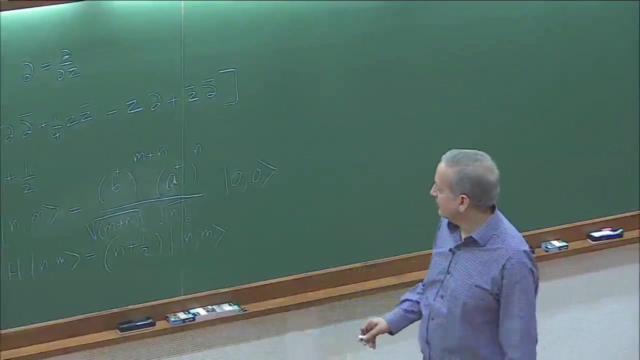 In real space by using the following click. so you ask: what is 0, 0? you see, we know already the form for these operators in real space, although you can work with just the operator algebra. but we know how to write these operators in terms of x's and y's or z and z bar. so we need to know what this quantity is, because 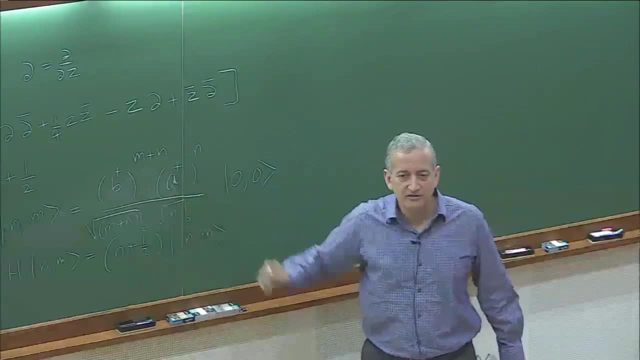 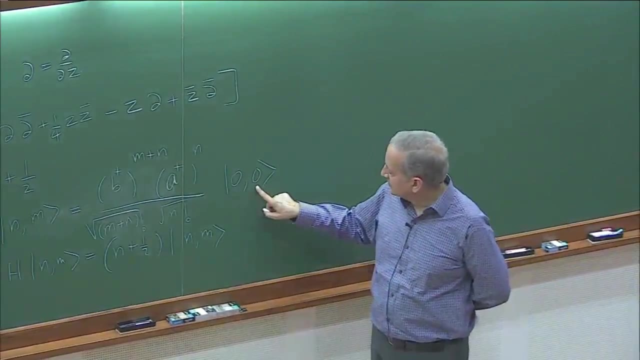 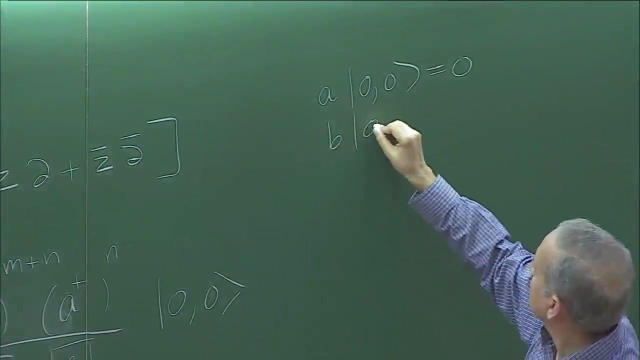 If you know this, we can just- it's just a question of applying it, applying these operators many times to get the actual wave function. this has the property that if I apply a onto this, it gives 0, or if I apply b onto this, I should get 0. this is a lower state. this is a state that's annihilated by both a and b. so with this information, you can show. 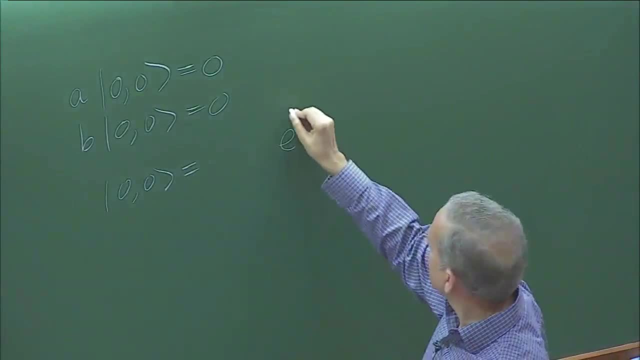 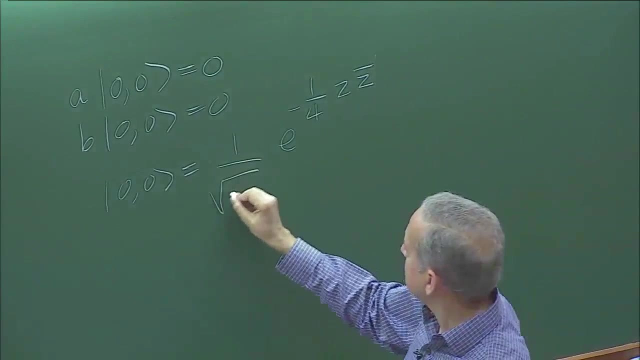 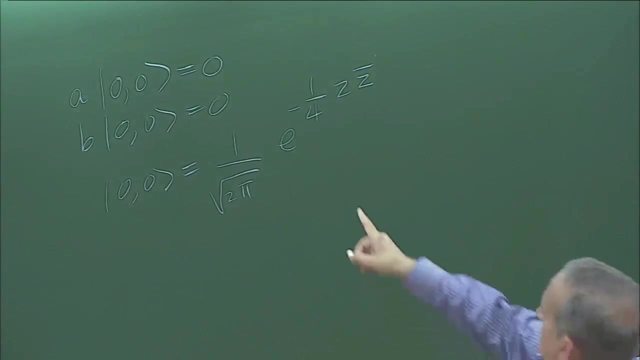 That this is given by e to the power minus 1 over 4 z bar, and I can even normalize it. so let's see. let's take, let's see if it satisfies one of these two equations. you can check for the other equation. so let's apply b onto this. 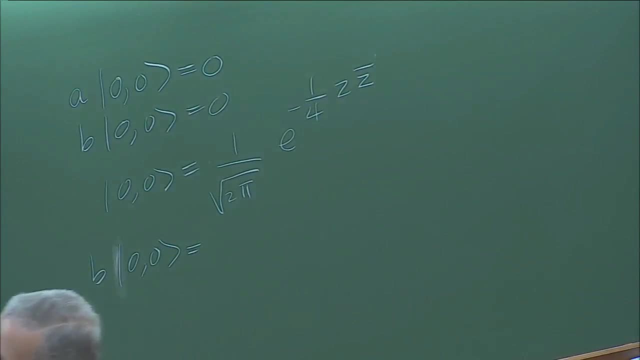 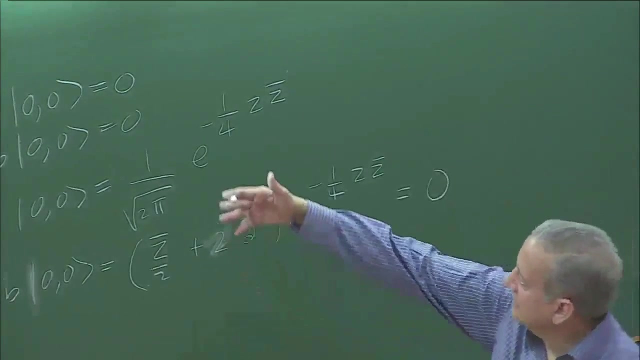 So for b I have this expression: z bar over 2 plus z l. I hope it works out. Yeah, it's 2 del. I was thinking maybe the whole thing I have done is wrong. it's 2 del. so you can see that this gives you 0 right, and similarly, acting a onto this gives you 0. so this is. 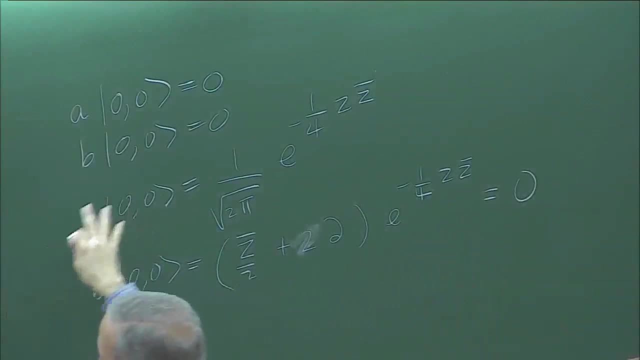 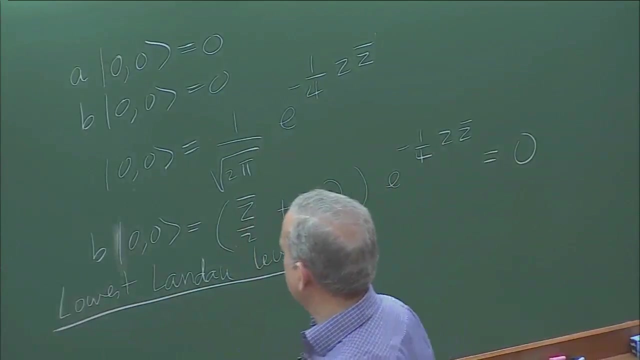 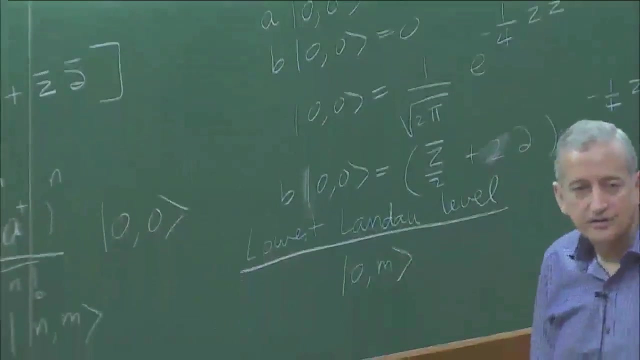 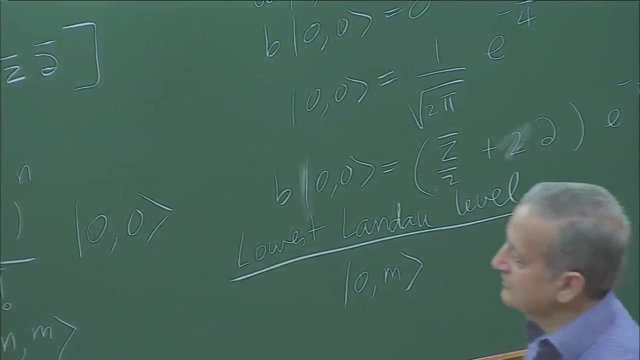 You know, With this substituted here, I can construct the full spectrum for all lambda levels. Now let's just try to see what happens in the lowest lambda level. So in the lowest lambda level, I choose n to be 0. And I choose m to be whatever an integer. all of these states have energy, which is 0 plus a half. 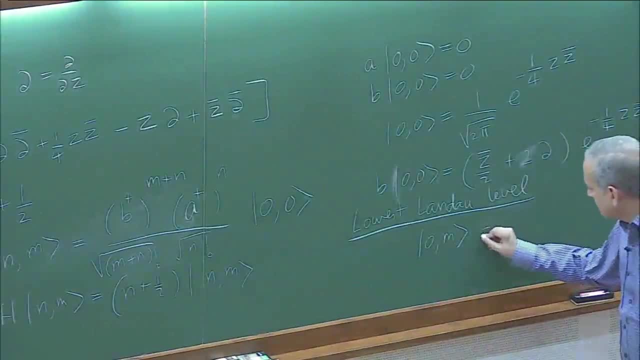 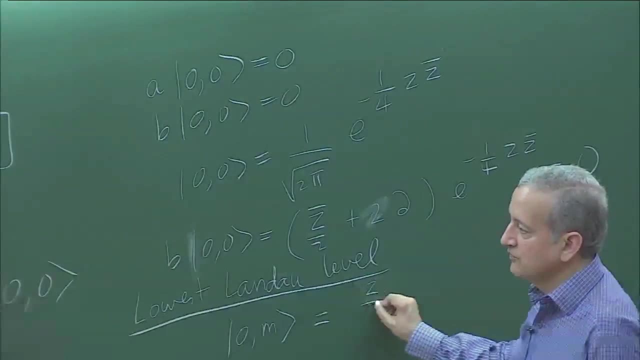 Okay, so they all lie in the lowest lambda level. the form of this is given as follows: so I have to apply b dagger, which is z over 2 minus 2 del bar, so I'm not worrying about the normalization constants. Okay x, So. 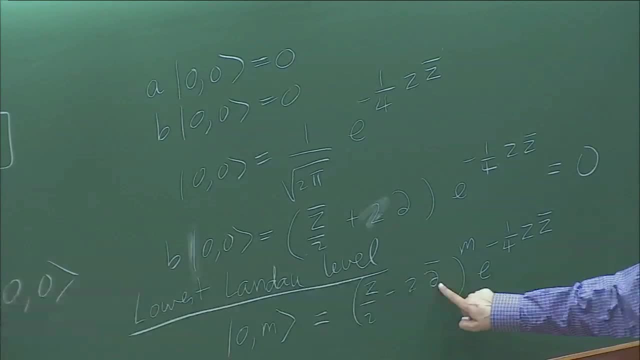 And X on. So You see, if you Act with a single power of del bar, it Pulls out a factor of z. So let's ask What happens when I apply this one of these factors? You can see that. 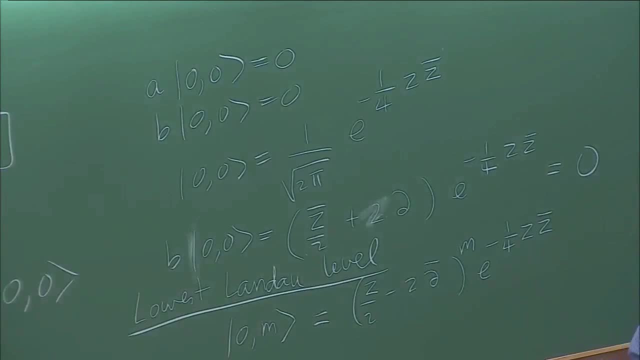 You get a factor of z. Okay, Okay, Thank you, Okay, Thank you, Good, Thank you, Good, Thank you. then, when you apply this again, it commutes with the factor of z and again acts on the exponential. it gives you another factor of this. so basically, this whole thing is proportional. 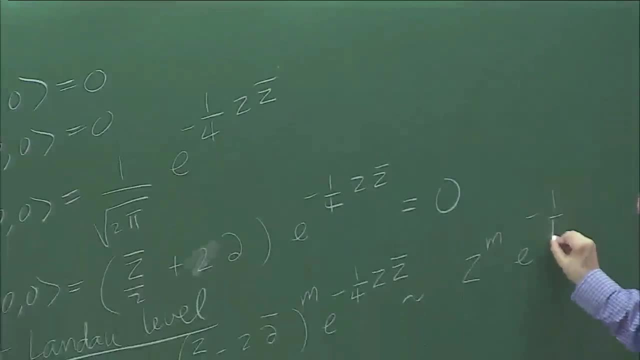 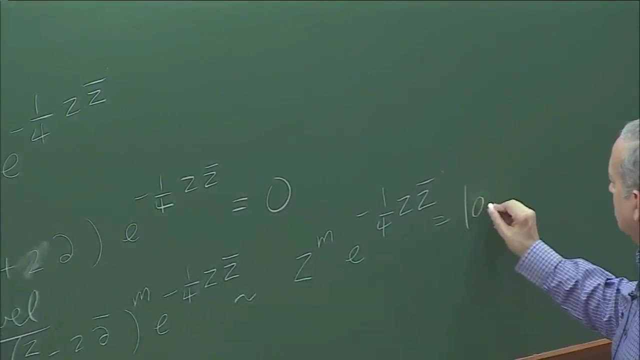 to z to the power, m, e to the power minus 1 over 4, z, that bar, and let's see i can. i can give it a name, so we are going to make use of this later on. so the wave functions, the single particle orbitals. 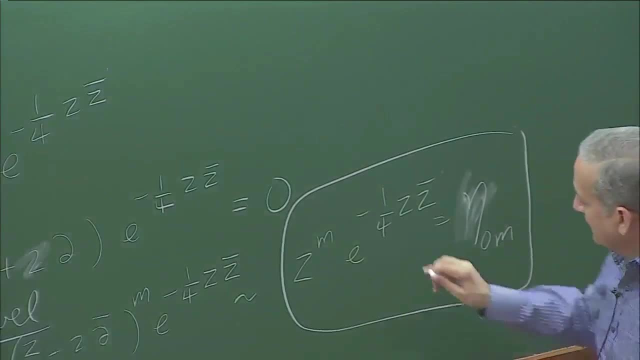 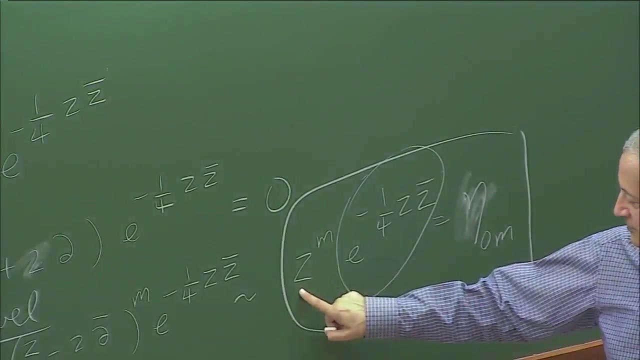 in the lowest slander level have very simple part. there is this gaussian factor which is always there, no matter which lander level you're in. but if you look at so, if you ignore the gaussian factor for a moment, the wave functions in the lowest lander level. they are, they are. 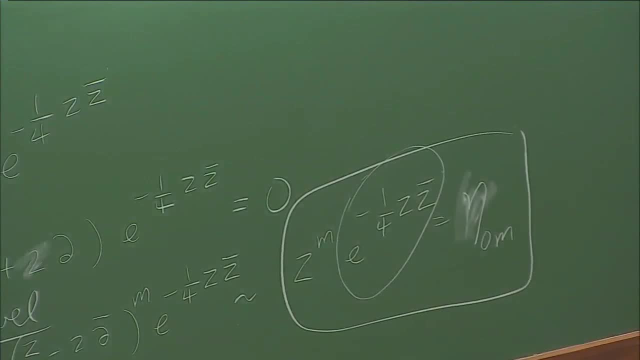 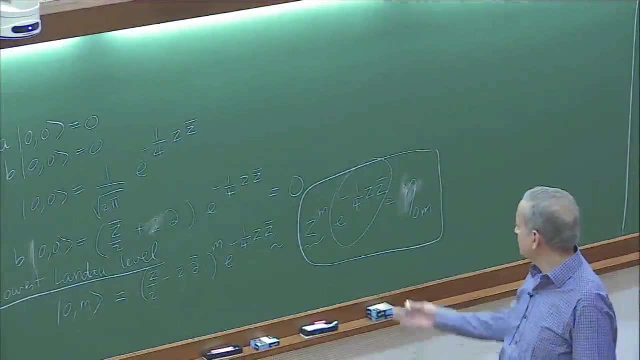 they involve only z. they do not involve any z bar. so sometimes people say they are analytic functions of z. I will: yes, this is so. by putting m equals 0,, 1,, 2,, 3, up to infinity, I span the full. 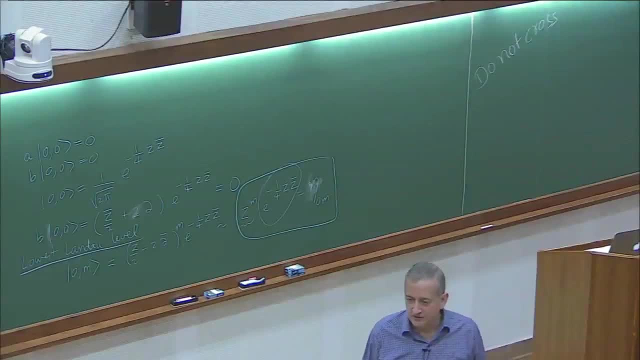 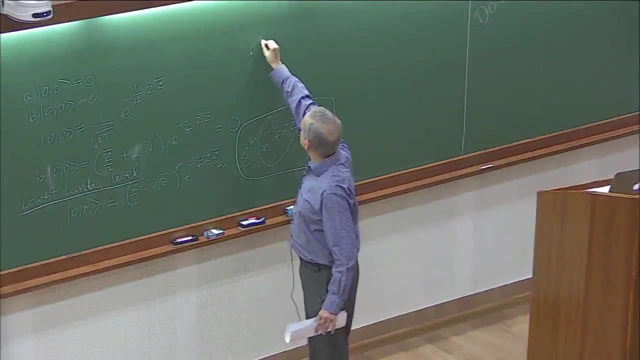 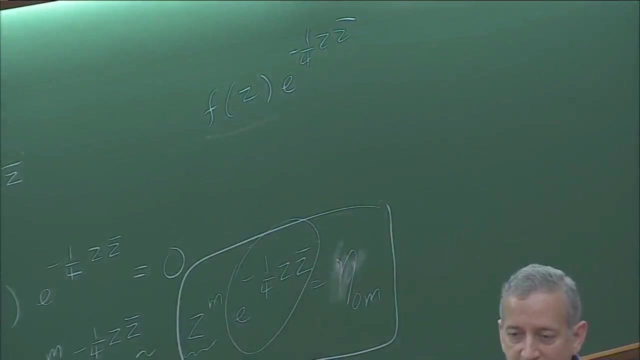 width space of the lowest lander level for a single particle. So in general, if you want to write any wave function in the lowest lander level, you would say that it will have a form where this f is some analytic function of that. ok. 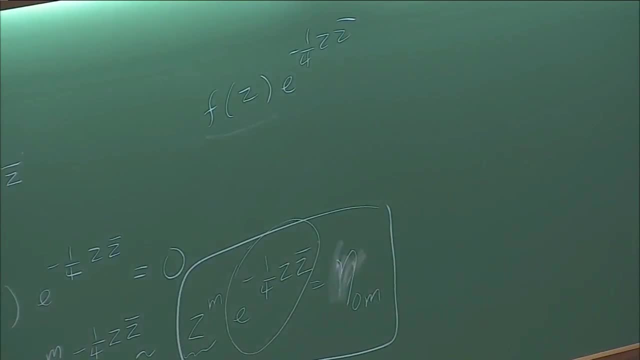 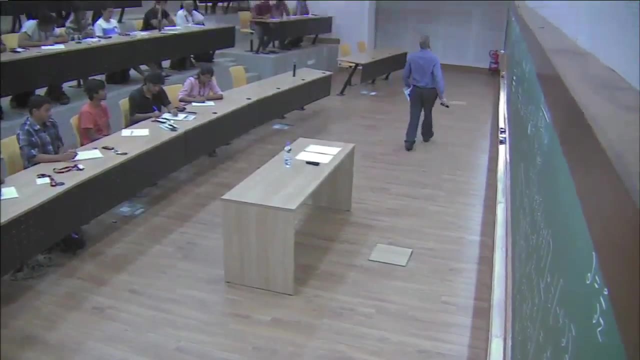 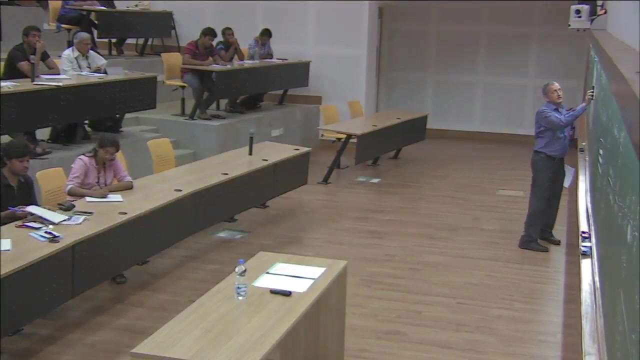 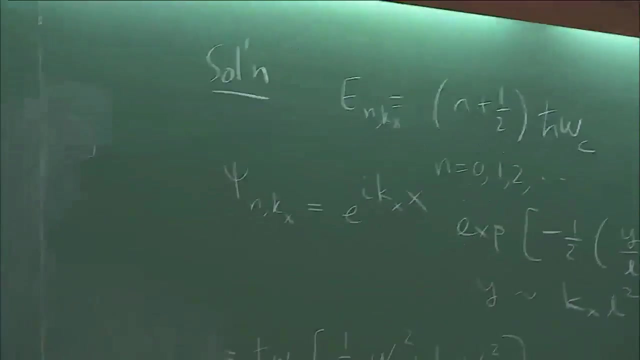 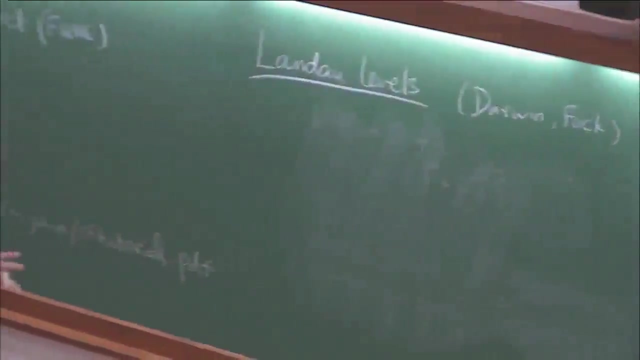 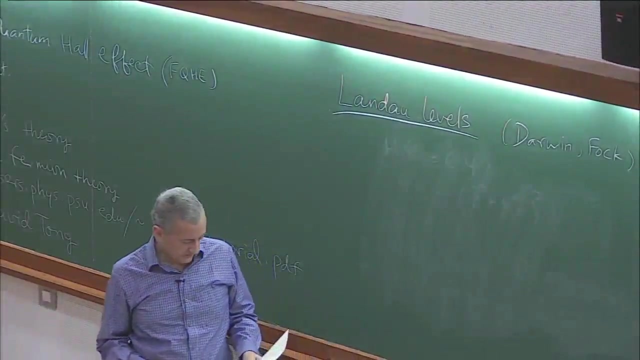 Alright, let me derive a couple more results which I am going to need for later. So So, one thing is to give a meaning to this integer m. So I am going to show that m is nothing but the angular momentum. So the only relevant angular momentum here is z component. 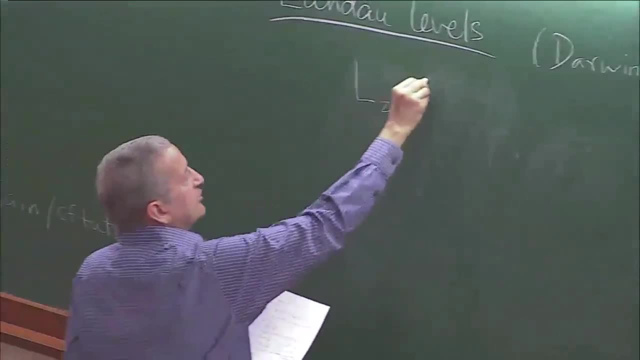 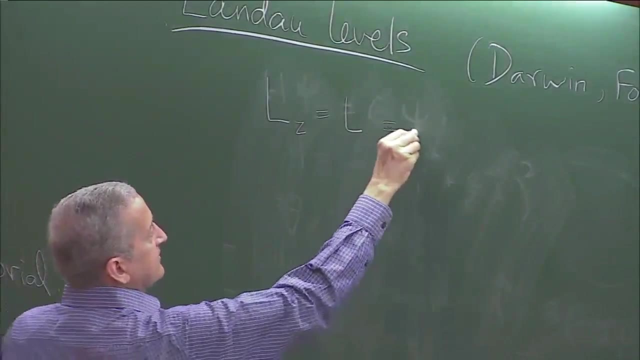 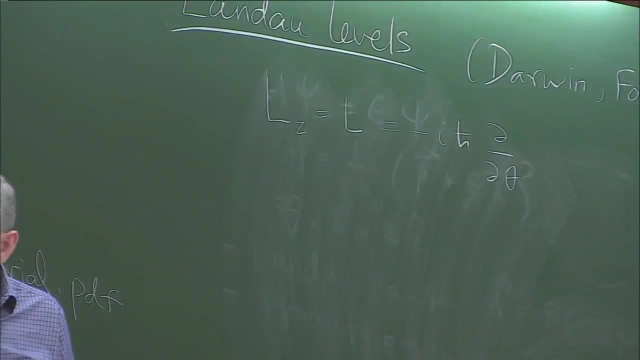 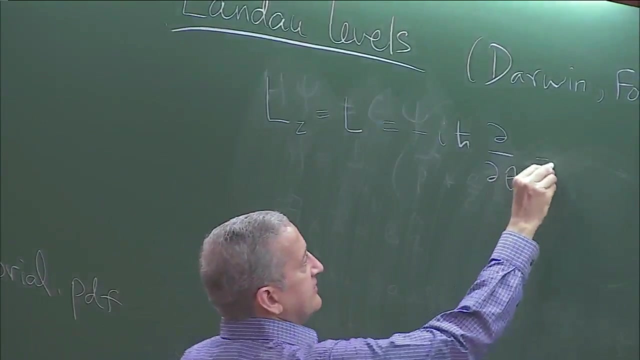 of the angular momentum. So I am just going to call it l, because we do not have any other components for the angular momentum. and this is minus i h bar del del theta, where theta is the angular variable. So again, please do some algebra to show that this is equal. 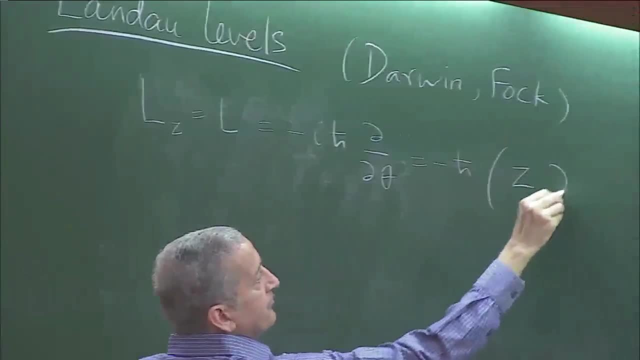 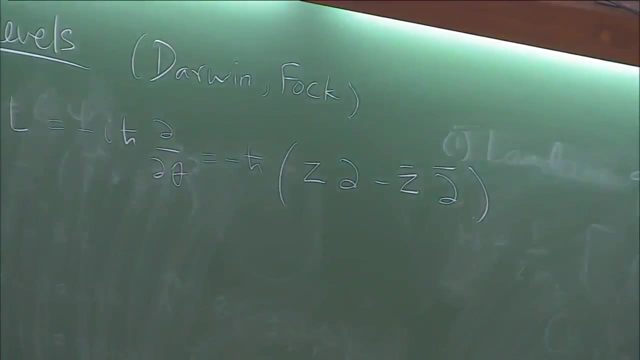 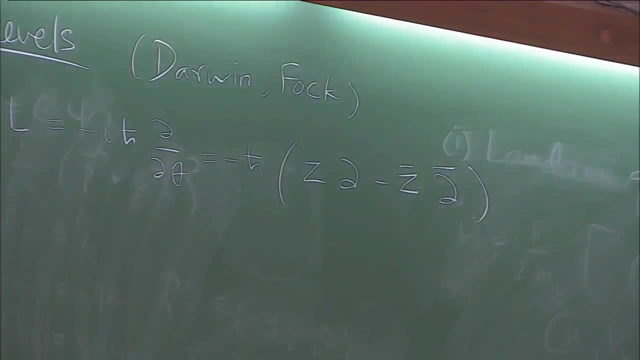 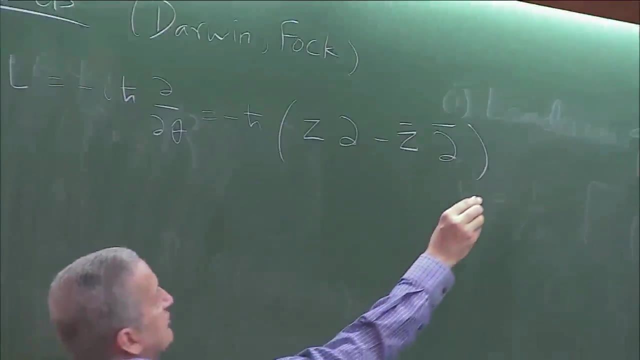 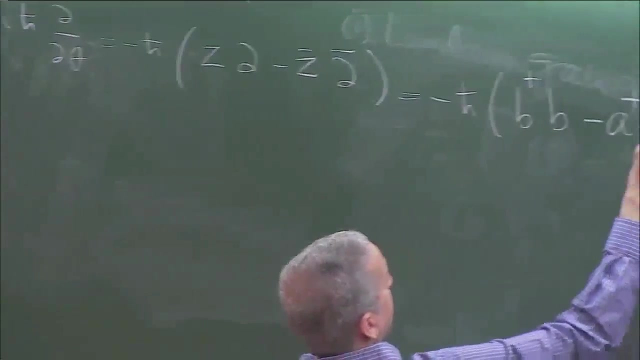 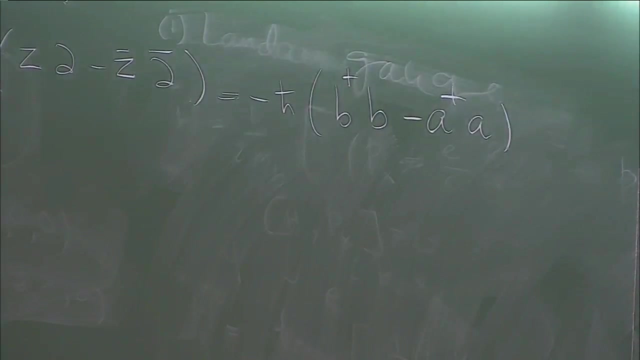 So you can change the algebra here and then do another algebra which is minus. роль is minus 8 is equal to this quantity. ok, So you will need to use the expressions for these ladder operators that I wrote on the right hand side of the blackboard. So these are: 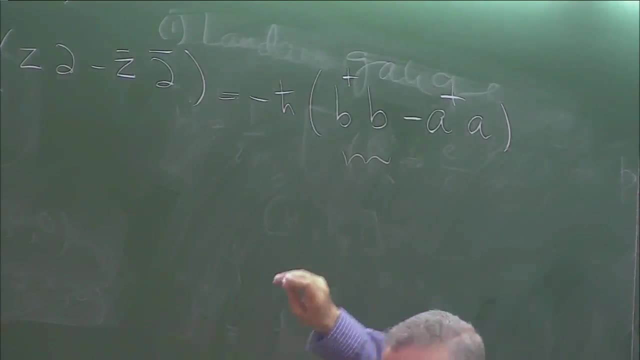 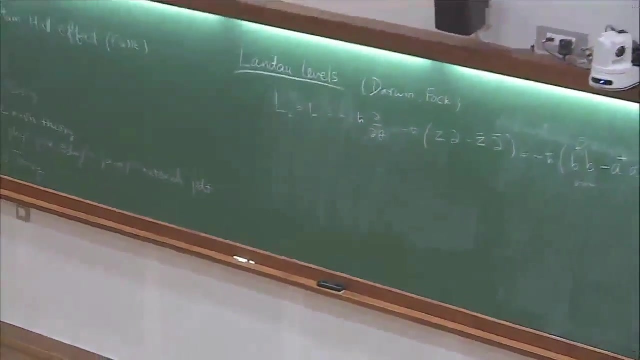 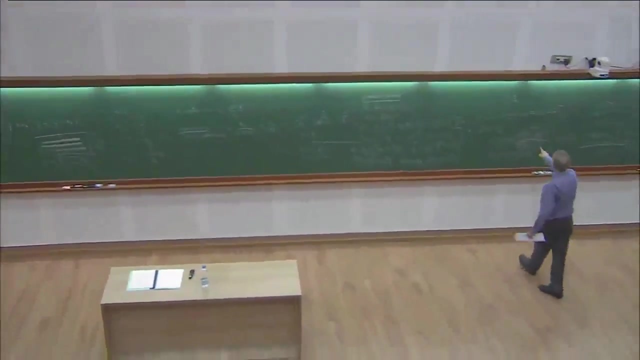 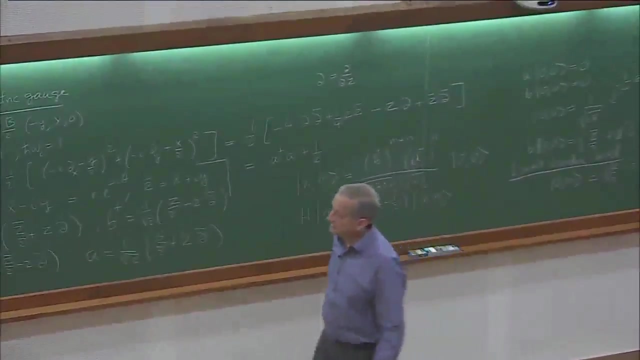 equal and notice that for our, for the wave function that we have labeled as n comma m, n comma m, the expectation value of b dagger b is m plus n and the expectation value of a dagger a is n, So the right hand side there. 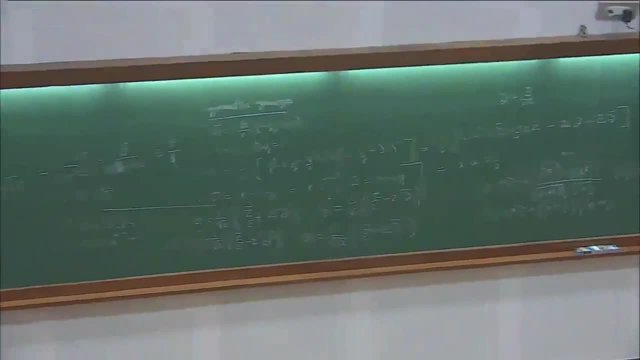 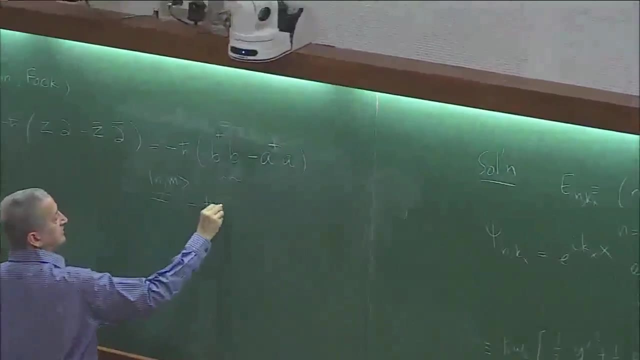 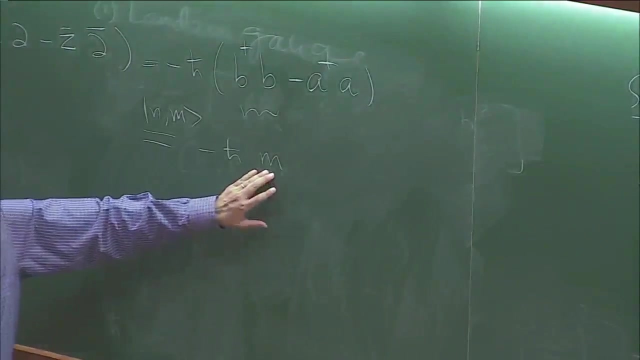 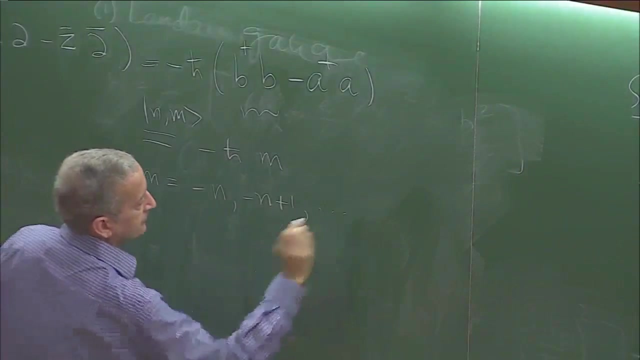 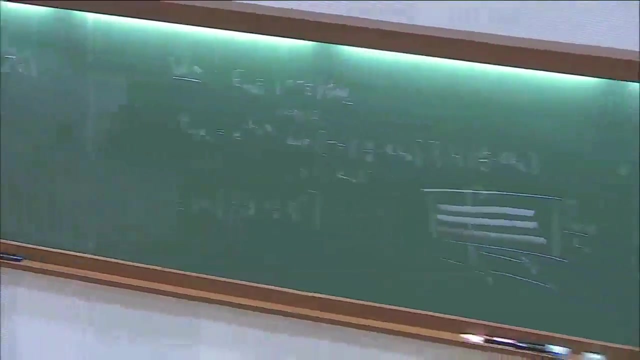 This, for it is equal to m, so this m is called the angular momentum variable, The way these equations are written, m goes from minus n, because it is because this quantity goes from 0,, 1,, 2, 3 onward. So therefore m goes from minus n. 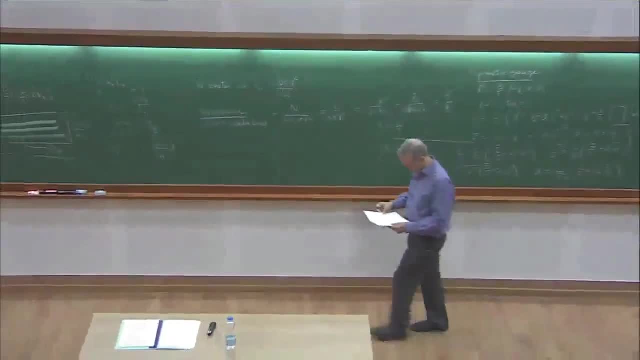 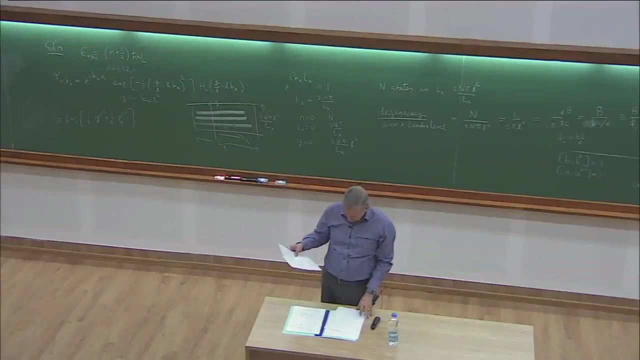 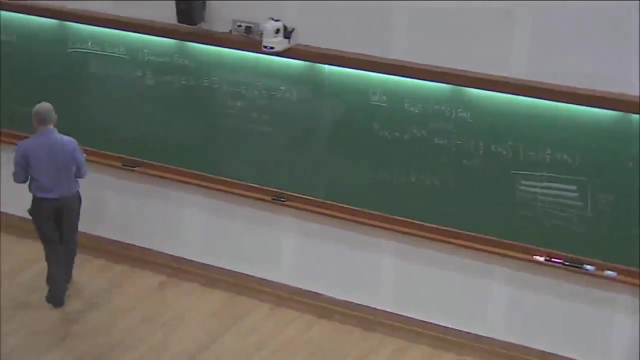 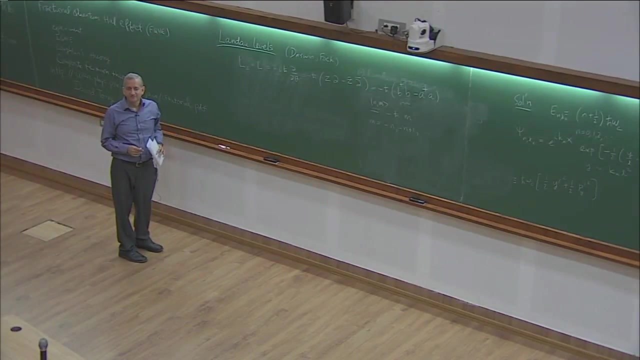 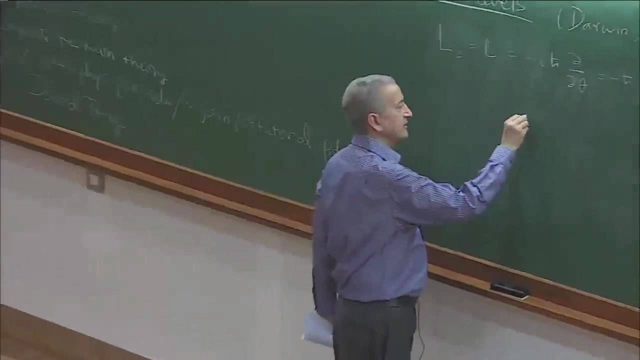 minus n plus 1.. Let us very quickly derive a couple of other results in this geometry. You could ask: what is the degeneracy? So if you, let us consider the lowest Landau level for the moment. So the wave function in the lowest Landau level has the form z. 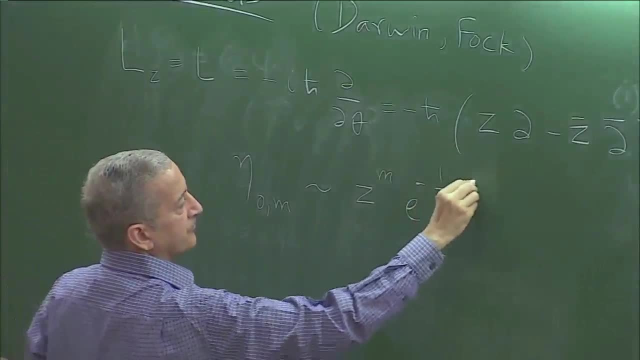 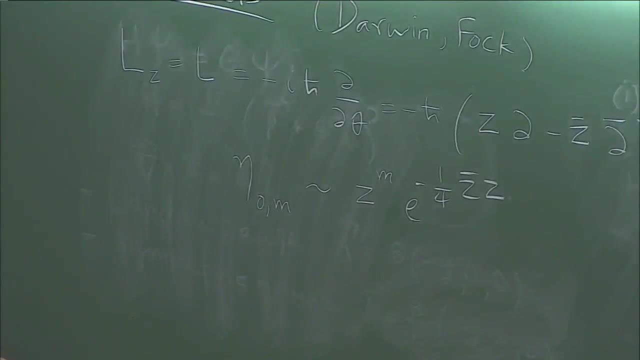 to the m. So what does this look like? Where is this wave function maximally located? Well, to do that, you take mod square of this and find the external point. Take derivative of that with respect to r. So this guy is periodic. 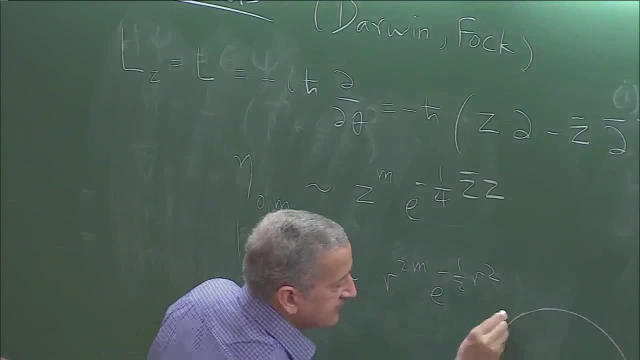 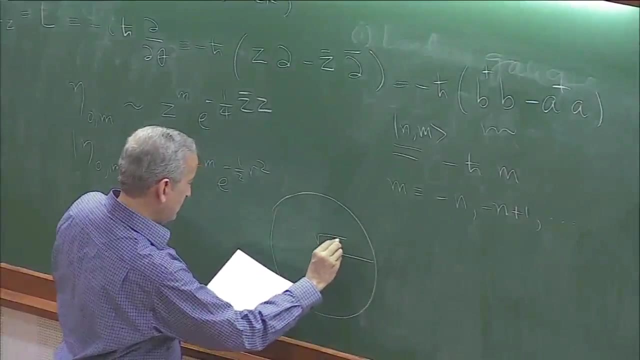 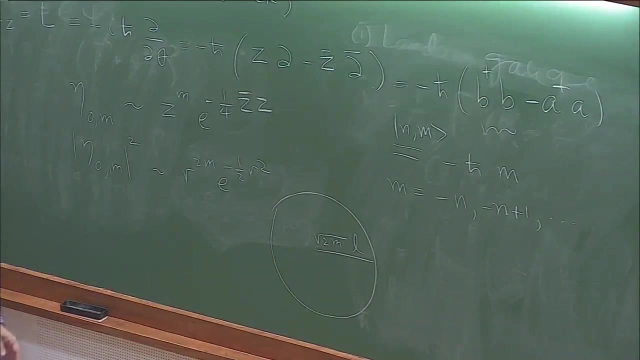 Thank you, Thank you very much, Thank you, Thank you, Thank you. is like as a circular shape. its radius is a square root of 2m and I am putting back the length scale, that is a magnetic length, so you can get that just by taking derivative. 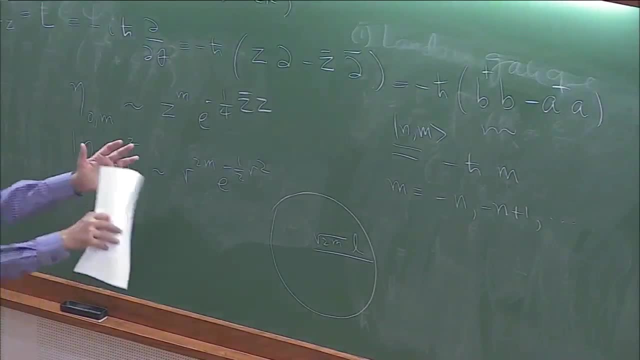 of this and setting it equal to 0, so it looks like this. now you may say: well, this wave function looks very different from what we had in the Landau gauge. there we look like straight lines, but that's only a matter of choice of gauge. you know, because all of these 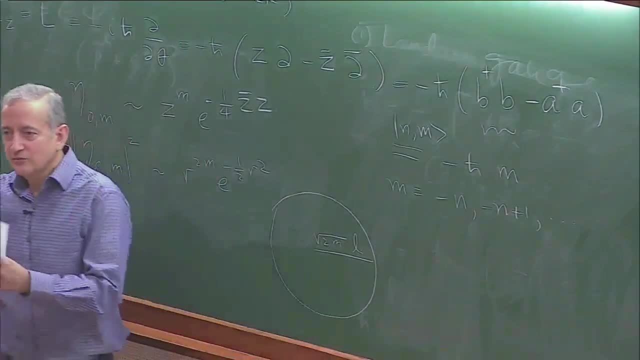 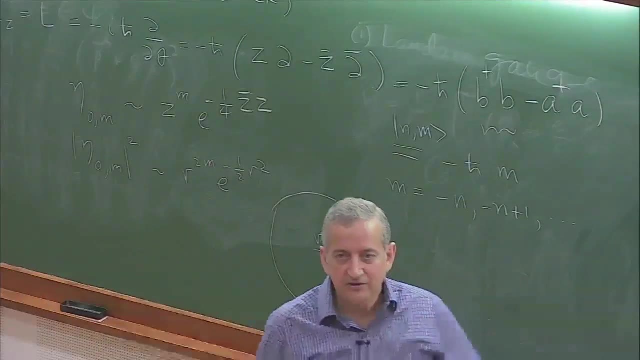 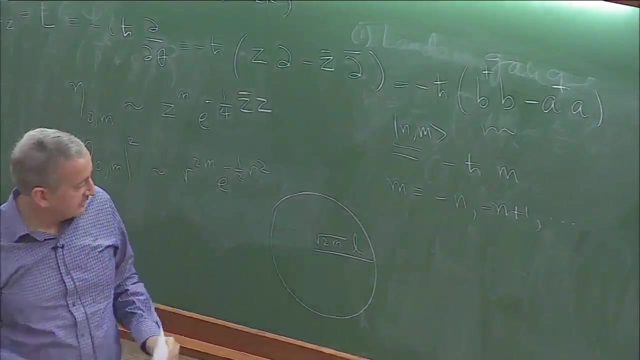 wave functions are degenerate. we can mix and match them to produce many different kinds of shapes. so these wave functions there can be written as linear combinations of these wave functions. they are all. they all describe the same physics eventually. but degeneracy can be gotten. 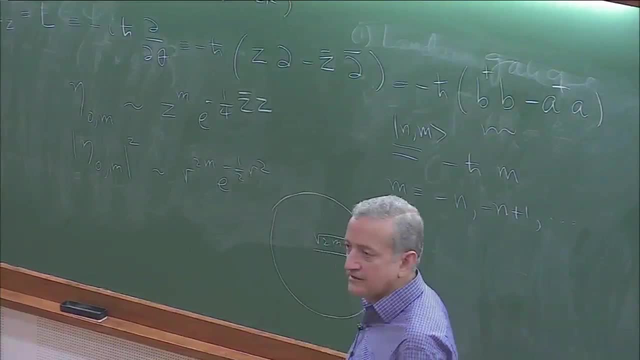 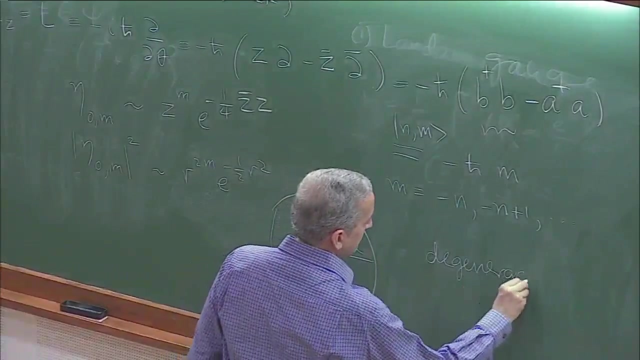 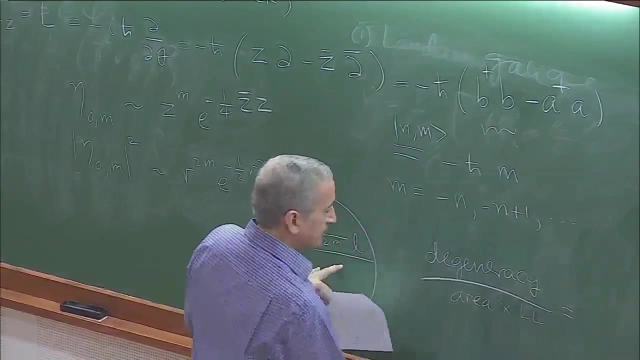 Straight forwardly because in this area I have m states right. so because states begin with 0,, 1,, 2,, 3, so in an area of this I have m states. so degeneracy per unit area per Landau level is equal to m divided by this area. 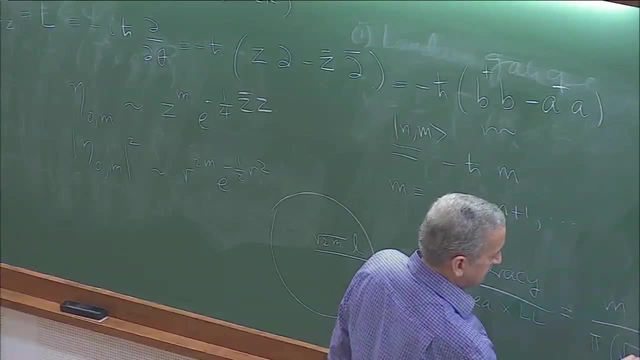 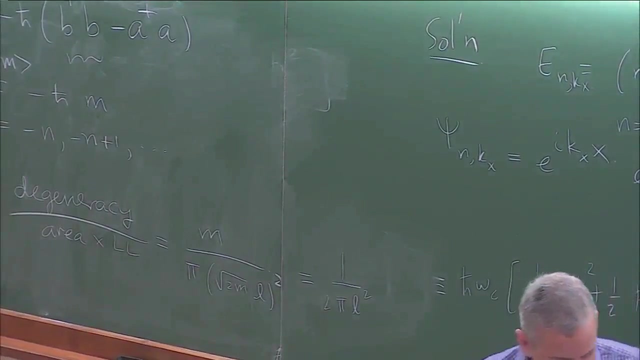 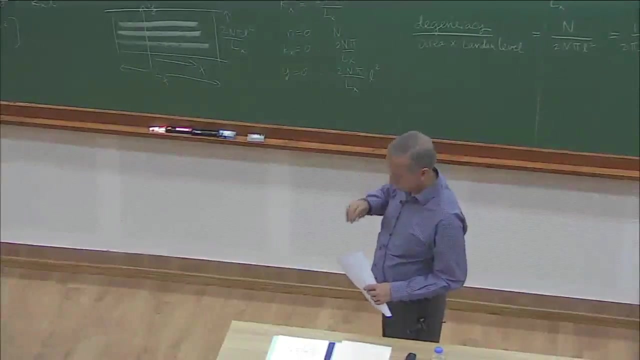 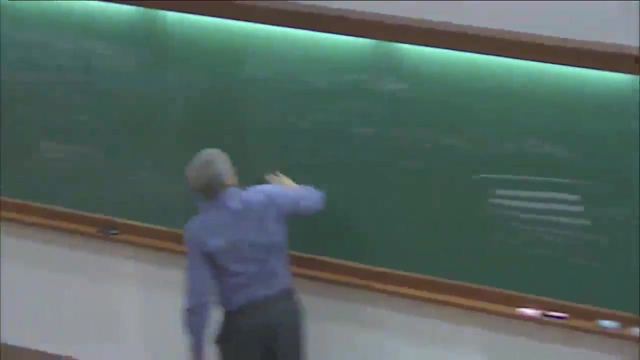 And this area is pi square root of 2m L squared, and you can see that it gives you the previous, gives you the same equation as what we had before. 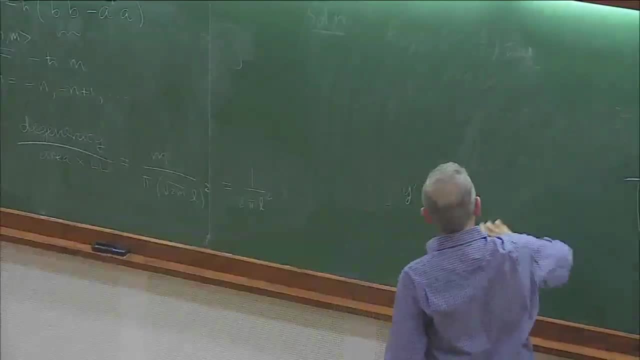 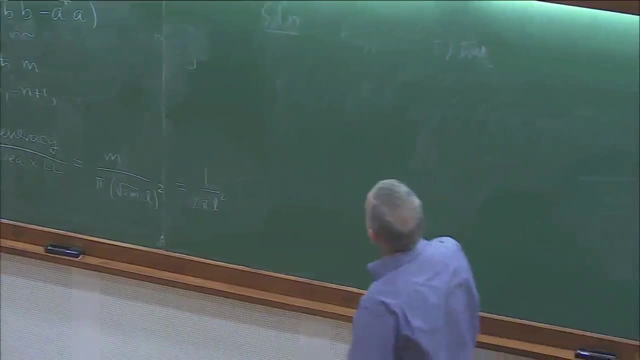 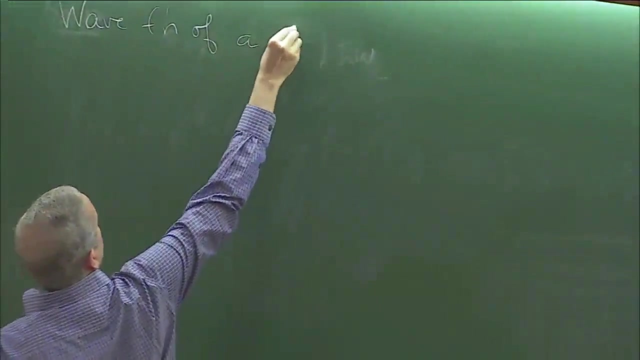 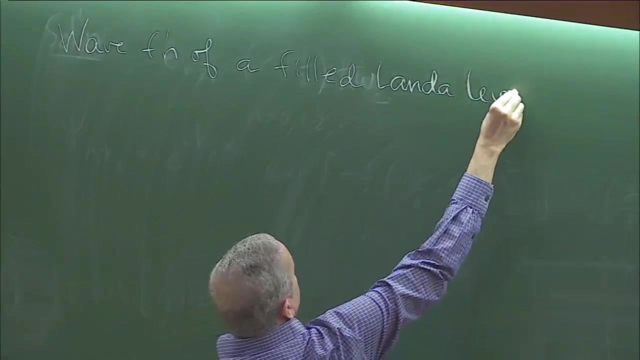 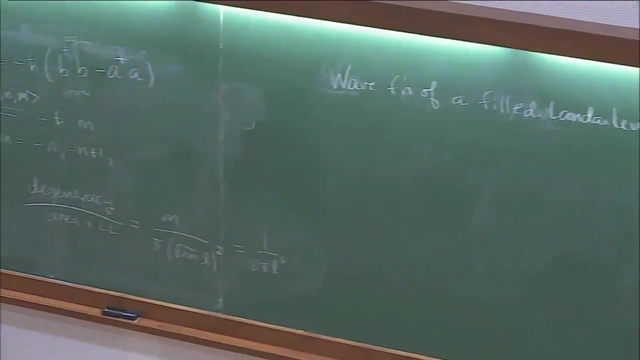 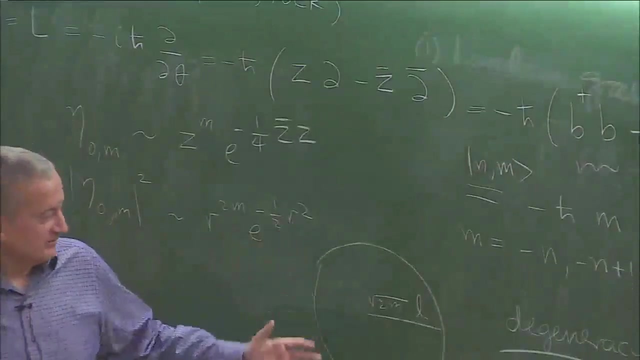 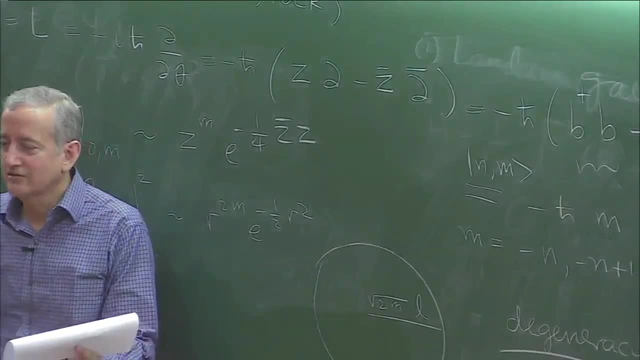 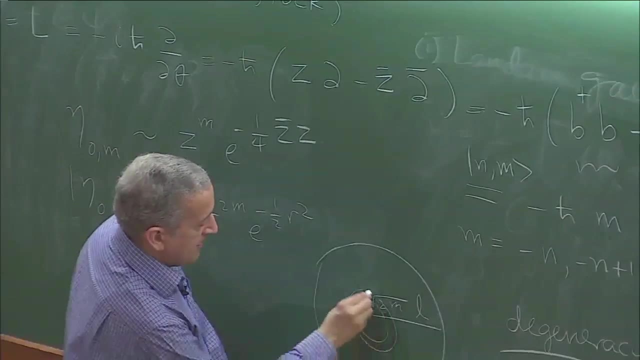 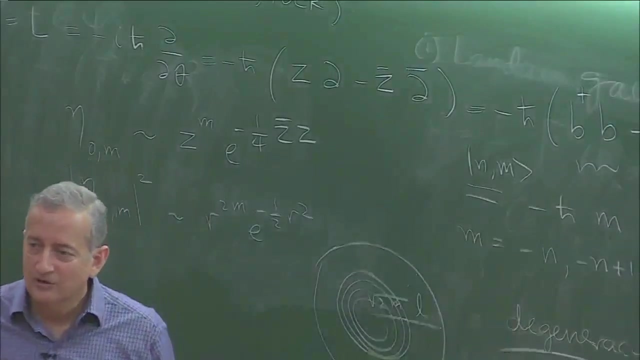 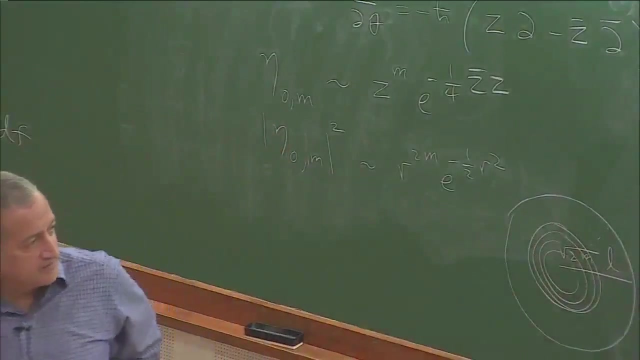 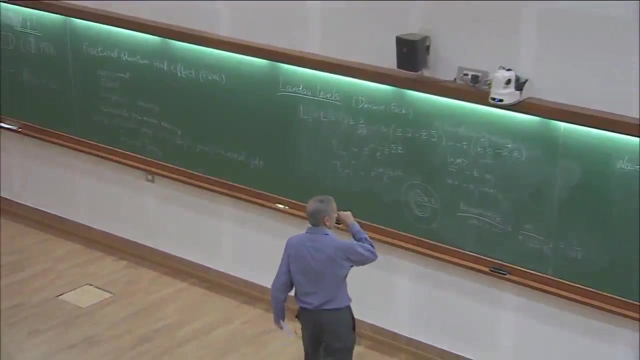 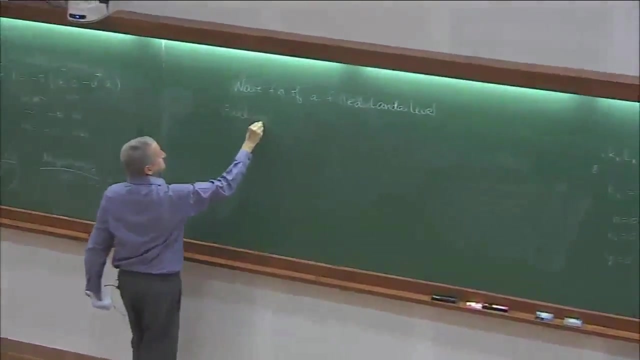 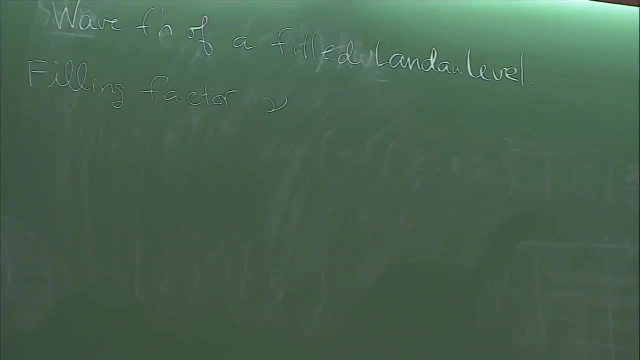 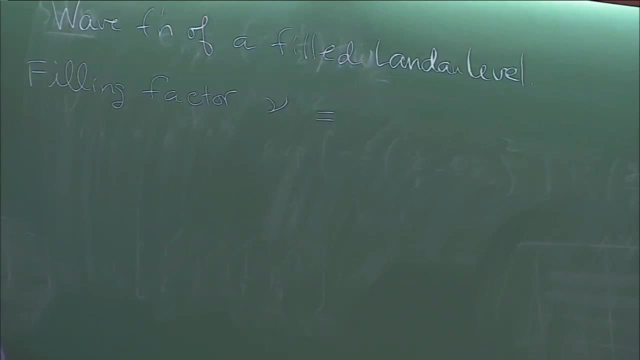 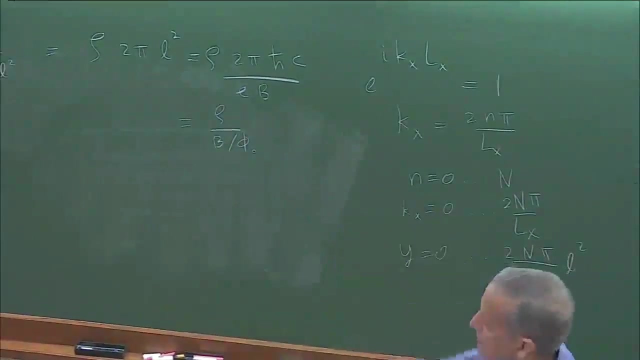 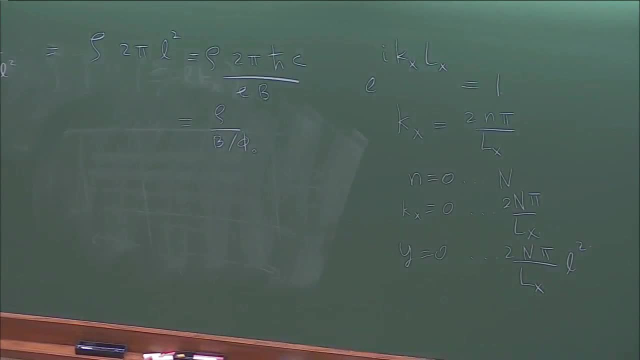 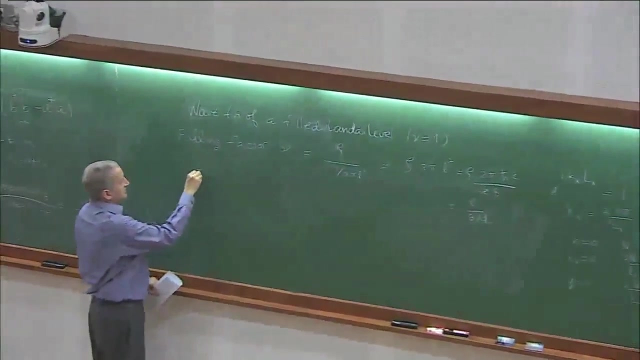 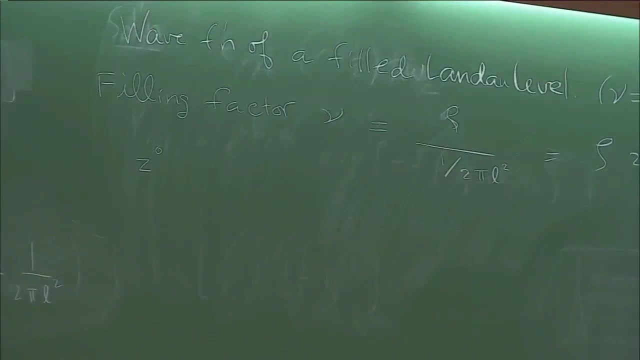 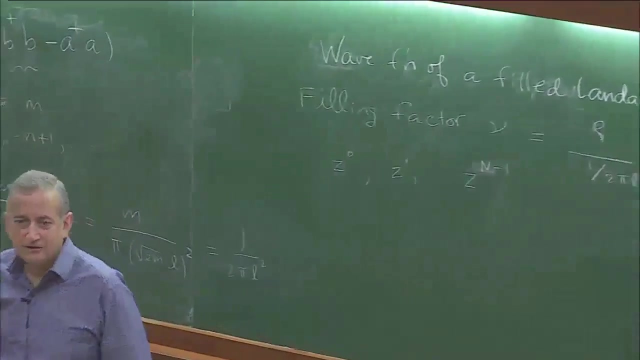 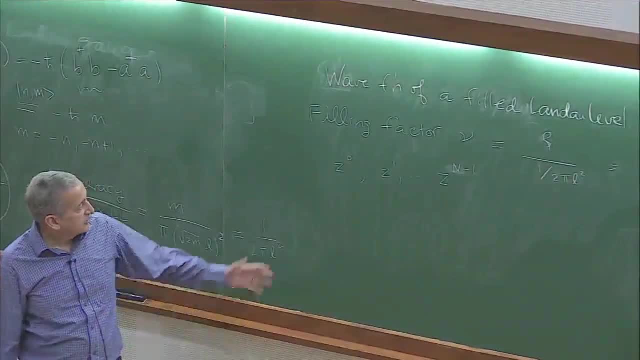 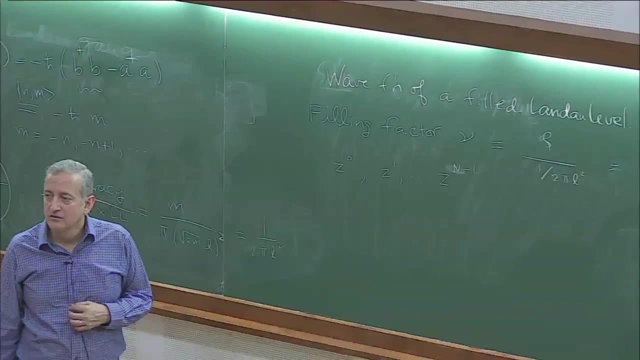 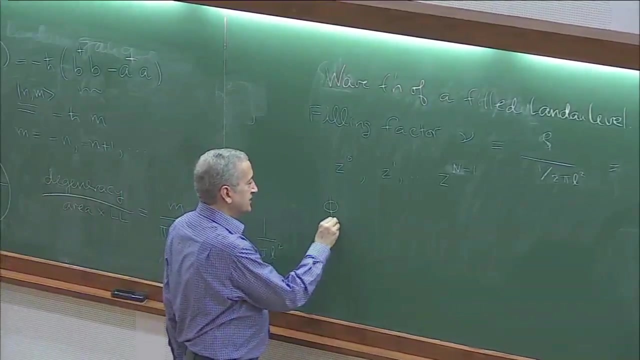 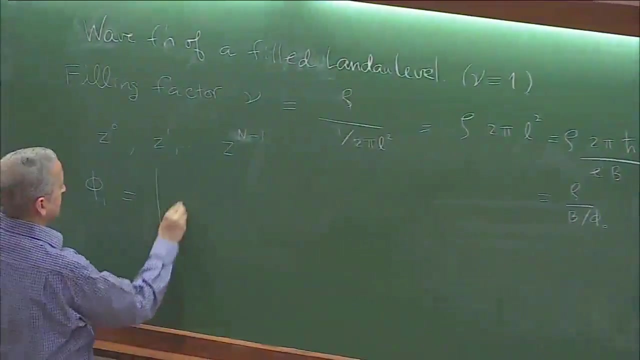 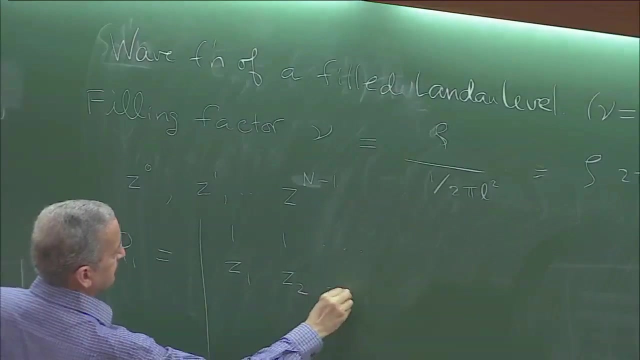 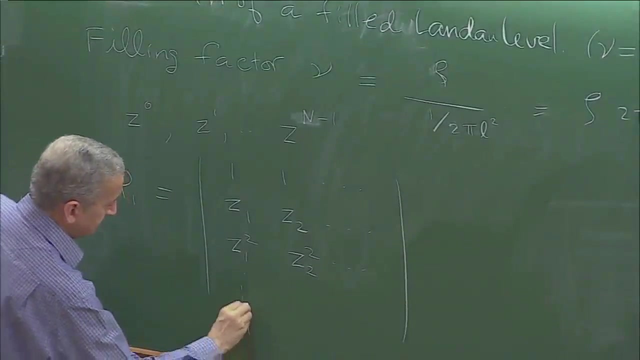 part has to satisfy anti-symmetry. so what do I do? how do I write the wave function of this many body state? yeah, later determinant. so in fact this is, let me call it, phi 1. where phi 1 is the filling factor, the slitter determinant would be: 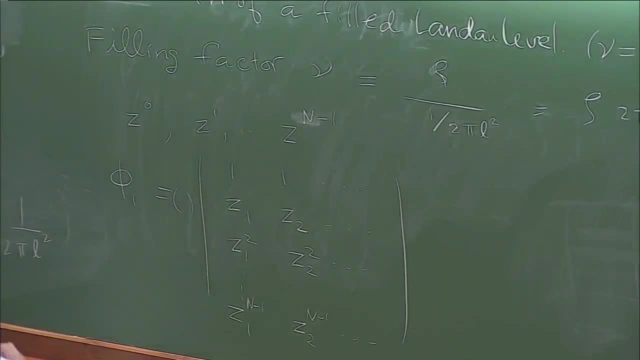 and there is some normalization factor here and we have the Gaussian factor. that's the wave function. now this slitter determinant actually has a name. it's called Vandermonde determinant. so this is the wave function of this many body state. so what do I do? how do I do this? 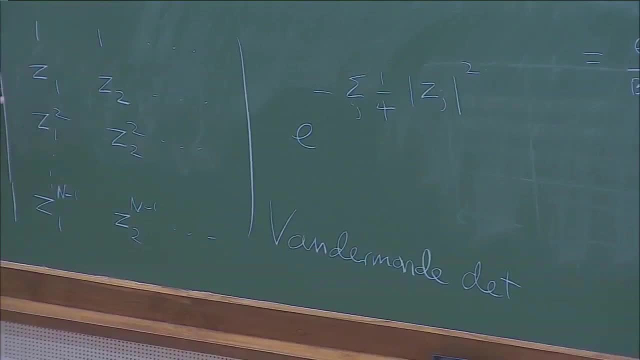 how do I write the wave function of this many body state? there are at least two ways to write I mean. so we have written the wave function explicitly, but it turns out we can write it a bit more simply. so one of the ways is something that. 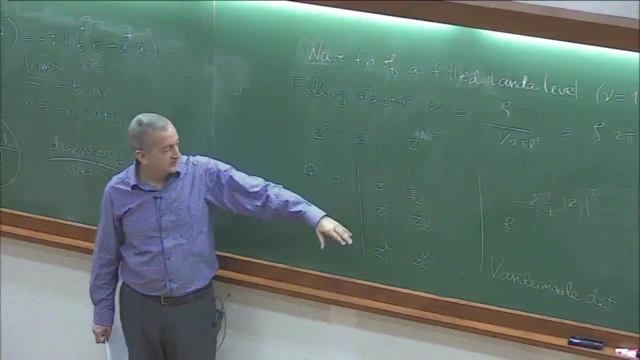 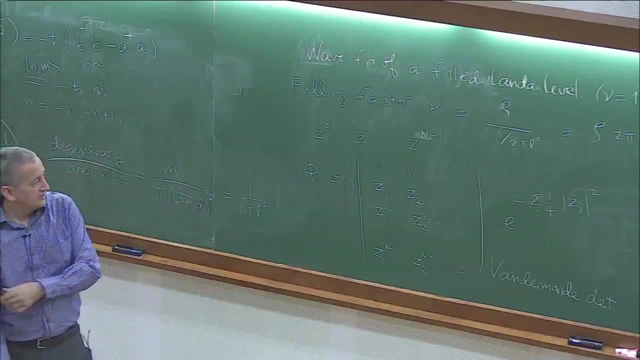 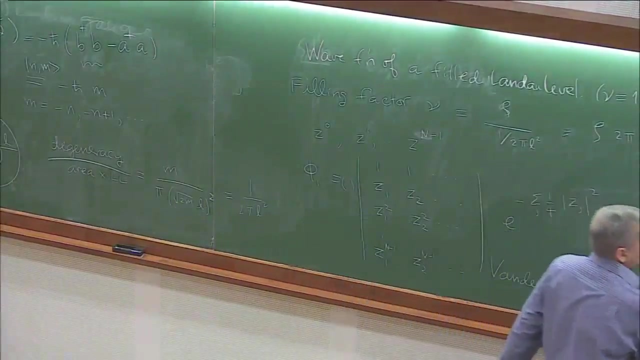 I am leaving for the home assignment for the tutorial session, so you have to do some row operations to derive the form for this, which I am going to derive in a more detailed way. Thank you, Thank you. So we have written the form in a simpler way, so we want to write this in a simpler. 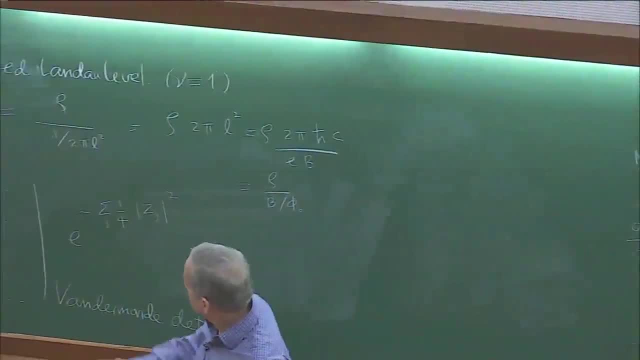 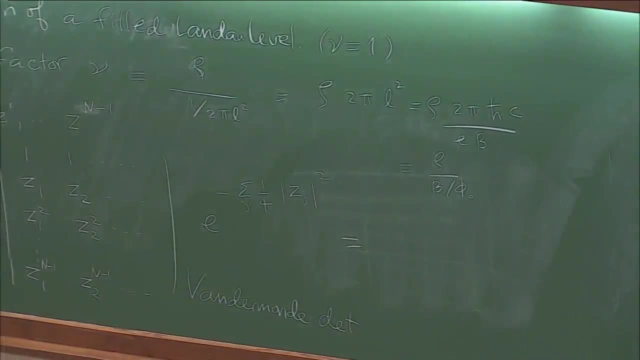 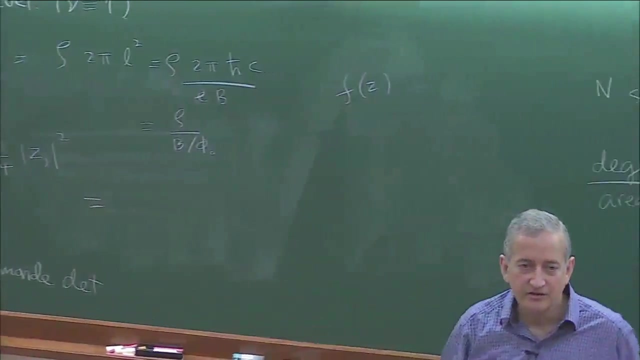 fashion again. let me not worry about the Gaussian part here. see, here I am going to use the fundamental theorem of algebra. so it says that if you have an analytic function of z- and let's say this is a megalithic function- that we have to derive the semitra refrescant. 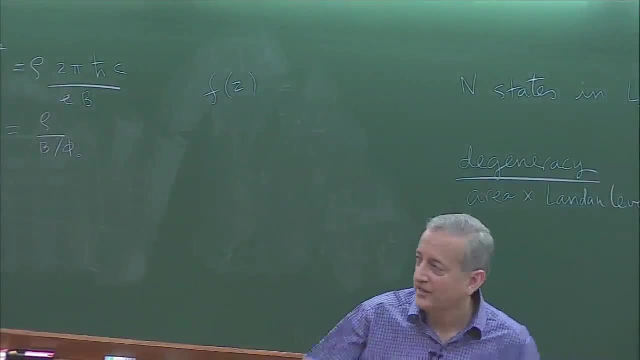 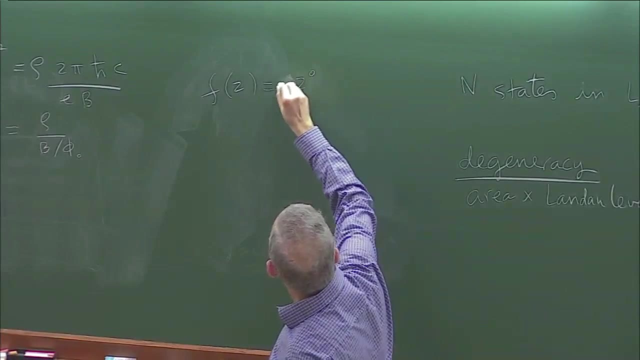 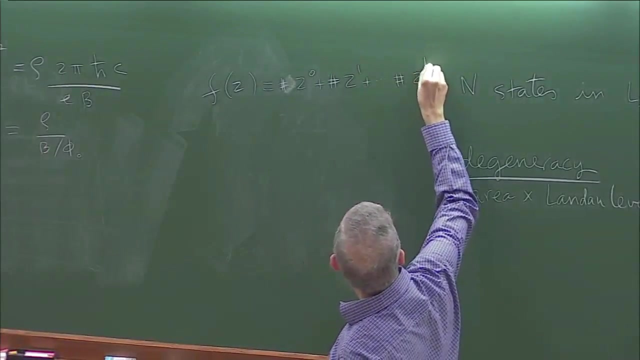 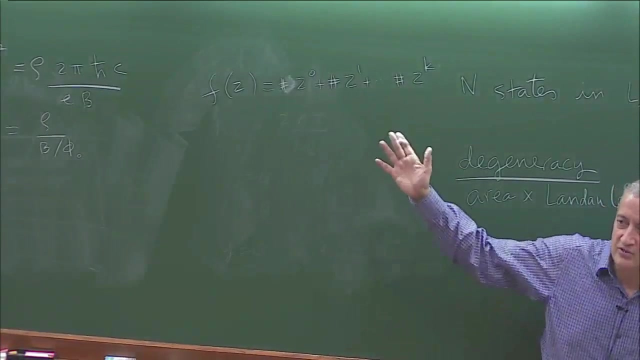 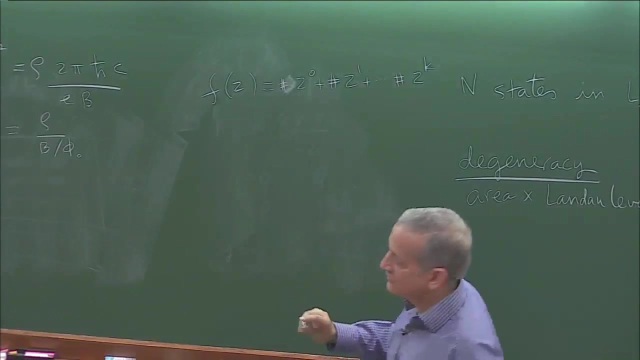 let us say the degree of this function is k. So that means you have some. so the largest power of z that comes in this function is k. let us say you have a function like that. So the fundamental theorem of algebra tells us that this function has precisely k zeroes. 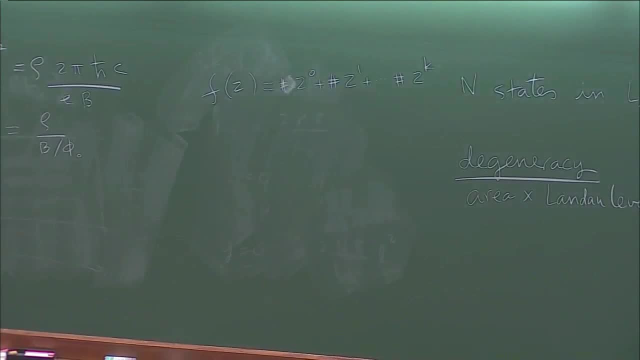 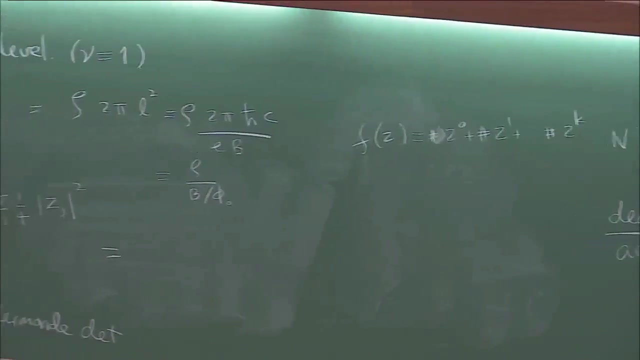 if you find a zeroes that precisely k of them. So I am going to use this. So if I look at this determinant as a function of, let us say, z1, so I am going to treat z1 as a function of z1.. So I am going to treat z1 as a function of z2, as a function of z3, as a function of. 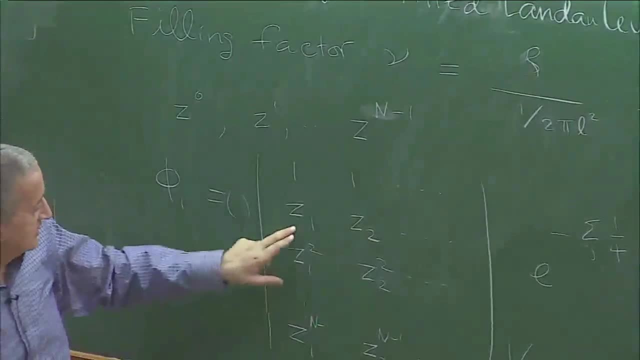 z4 as a function of z5, as a function of z6, as a function of z7, as a function of z8, as a function of z9, as a function of z10, as a function of z11, as a function of z12, z13, z14. 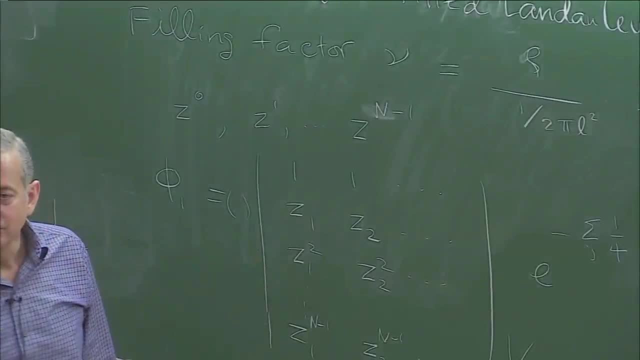 z15, z16, z16, z17, z18, z19, z19, z19, z20, z21, z22, z23, z23, z23. just as some numbers or variables, I treat it as a function of z1.. The degree of this polynomial is n minus 1, right, because 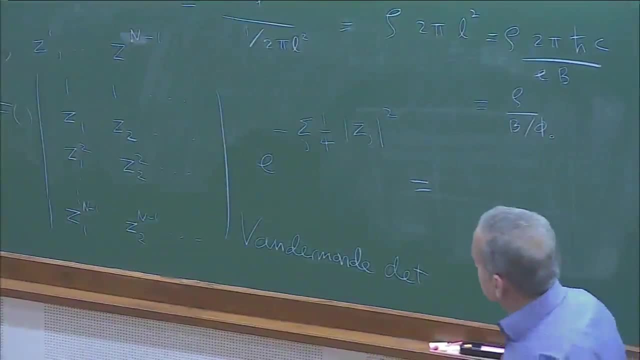 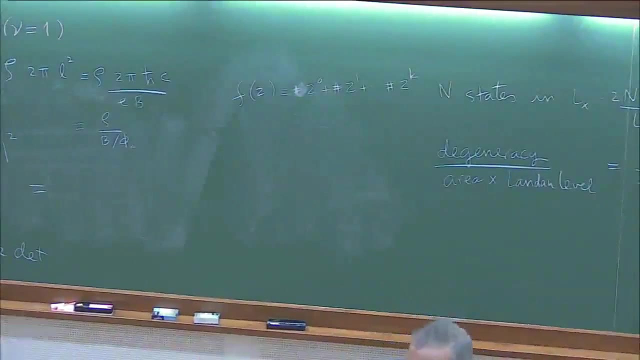 that is the largest power of z1 that occurs. Imagine you expand this determinant. you write it as a function of z1.. So the degree of the polynomial is n minus 1, we know there are n minus 1 zeroes. Do we know where the zeroes are? 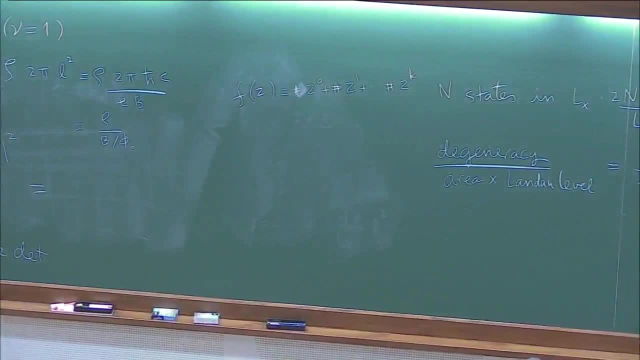 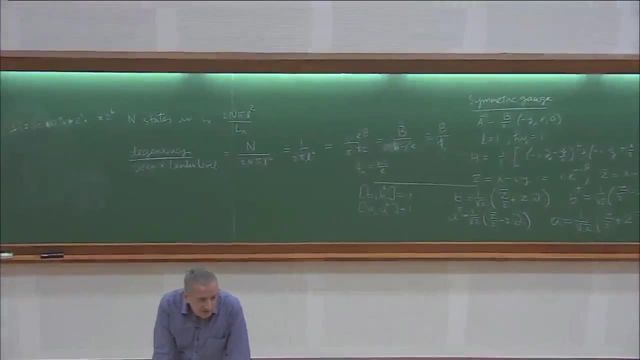 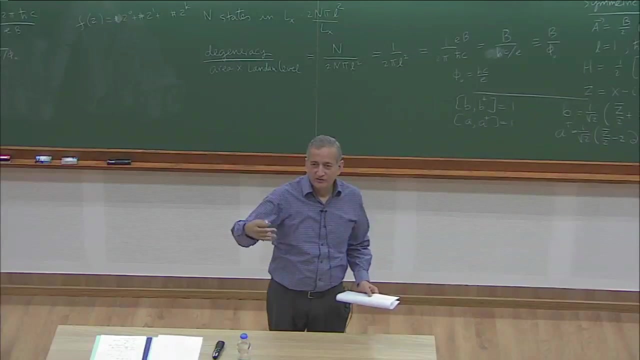 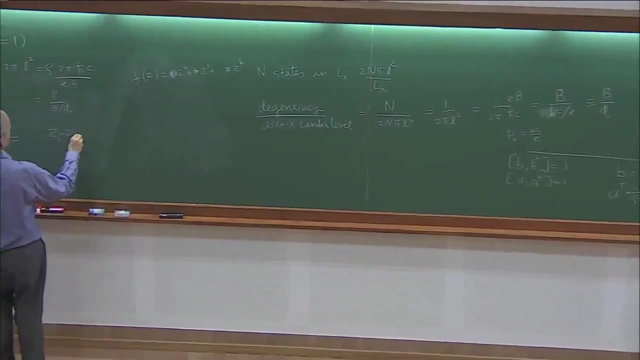 0. 1. 0 is when z 1 is equal to z 2, another is when z 1 is z 3. So 0s are sitting at other particles. So I know that this should have factors like z 1 minus z 2 and this actually. 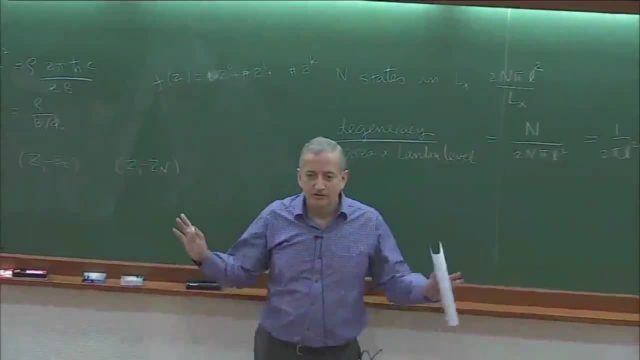 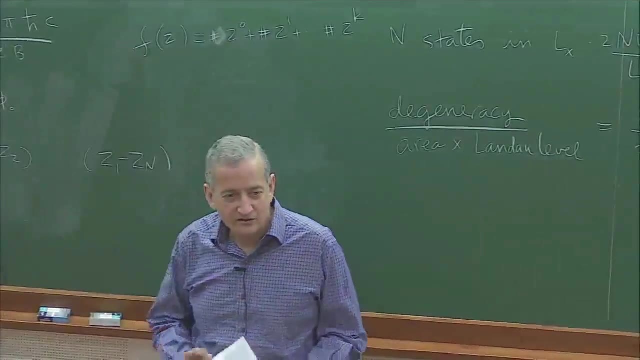 exhausts all the 0s. It exhausts all the 0s because there are n minus 1 0s and there are n minus 1 particles. So this is: there are not any other 0s. But now I should do the. 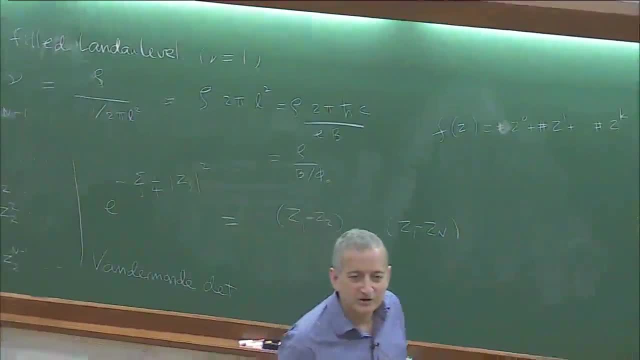 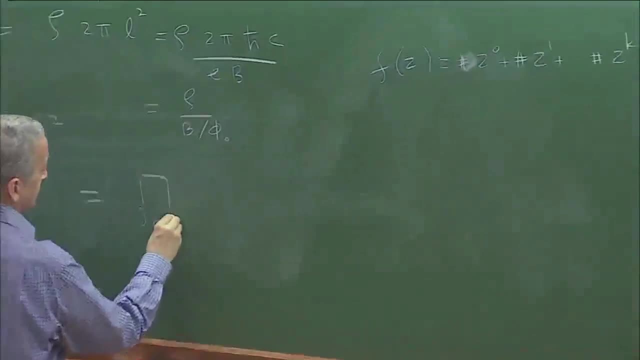 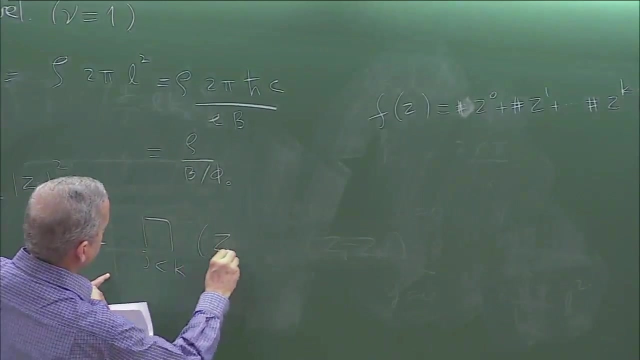 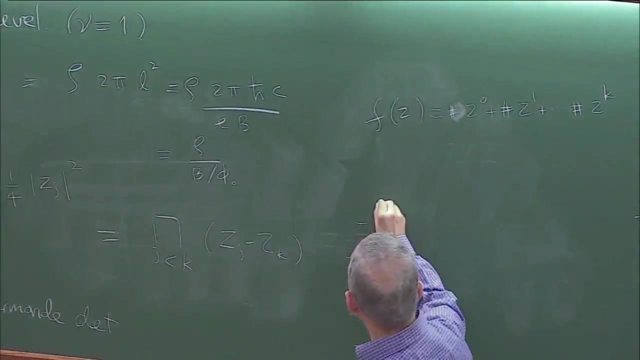 same thing for z 2.. Z 2 sees 0s and all other particles and so on, And therefore this wave function looks like this: apart from normalization factors or signs of plus and minus 1, etc. And of course we have the Gaussian factor. So this Vandermonde determinant has a very 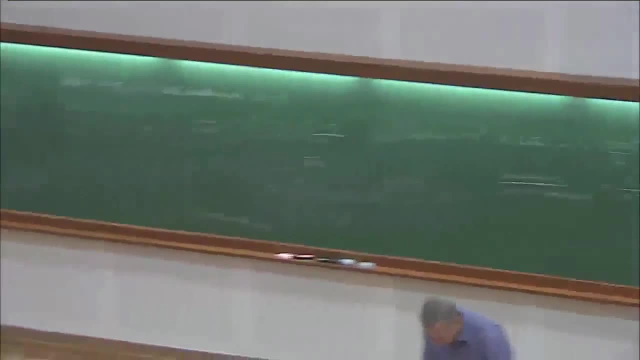 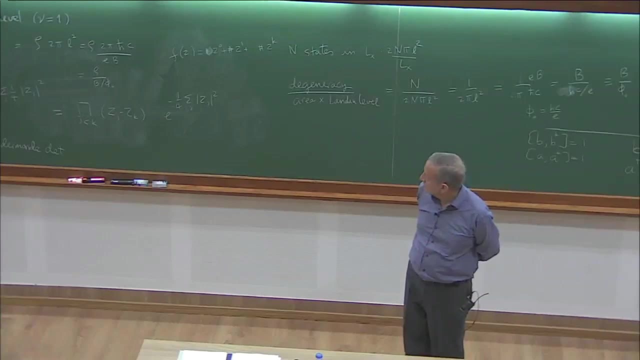 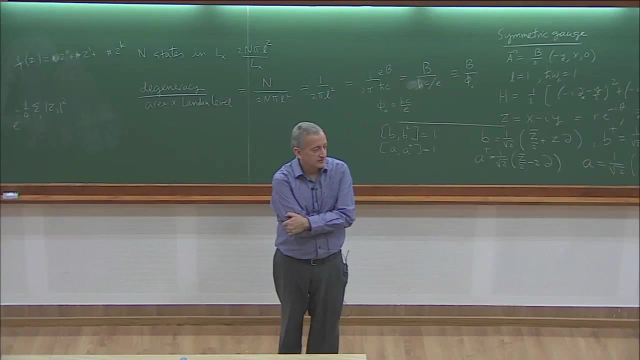 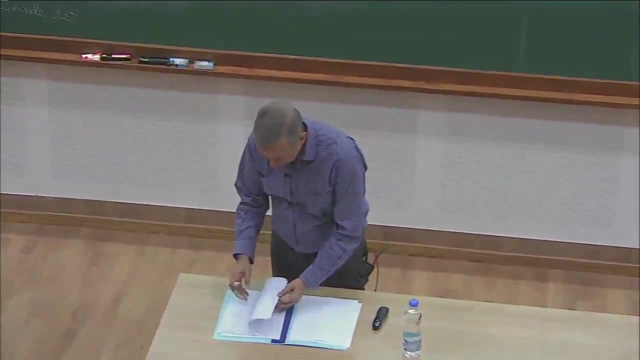 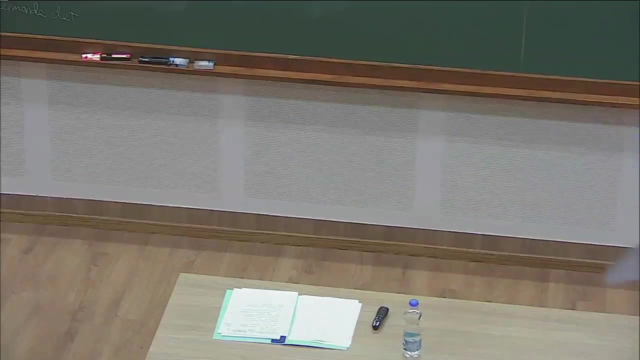 simple form and we are going to make use of this later on. This brings us to the next topic, which is integer quantum Hall effect. So I am going to do that relatively quickly, because that is not the main, that is not the emphasis. 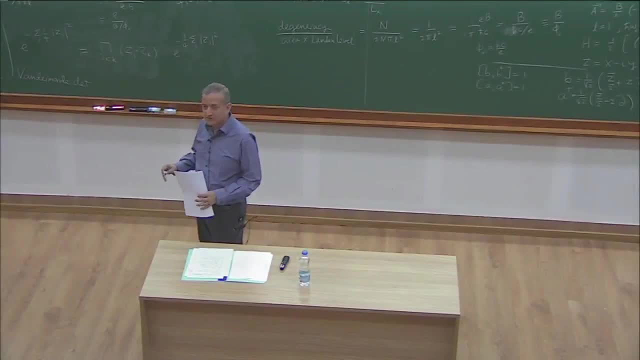 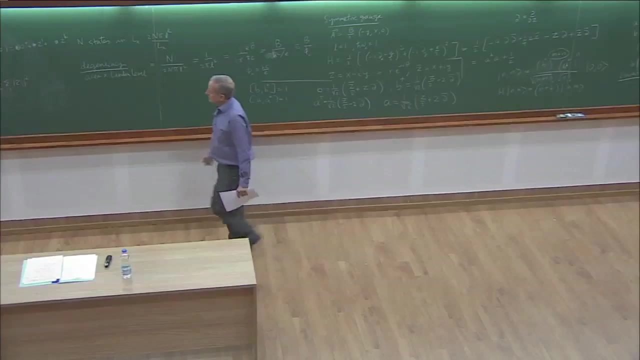 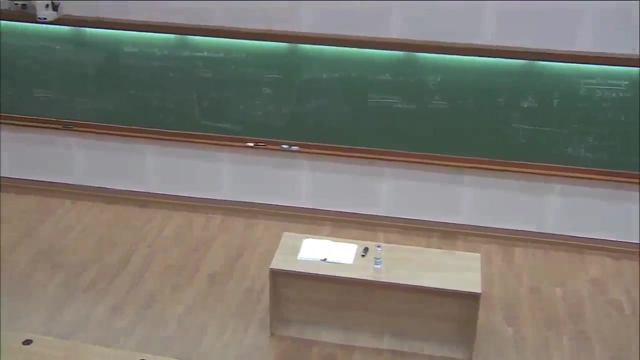 of this, of this, of these lectures, But still, knowing how integer quantum Hall effect is explained is crucial for the understanding of the fractional quantum Hall effect. So let us begin with just a classical Hall effect. 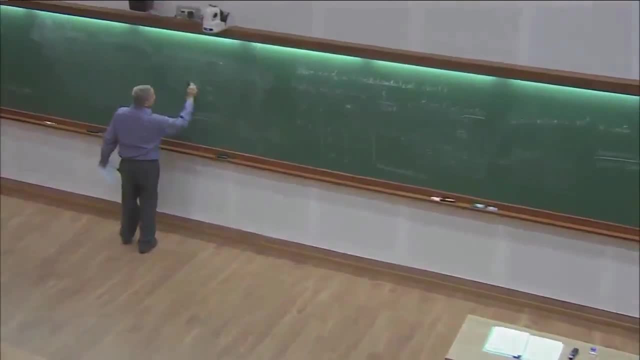 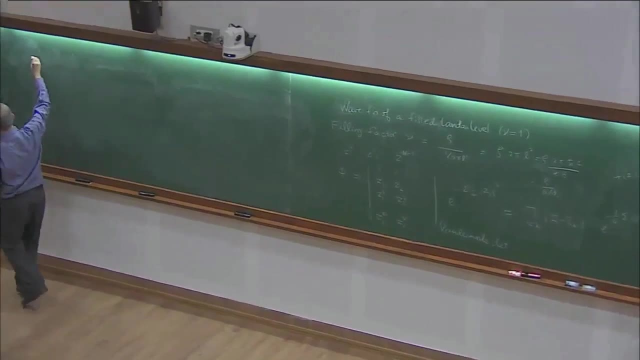 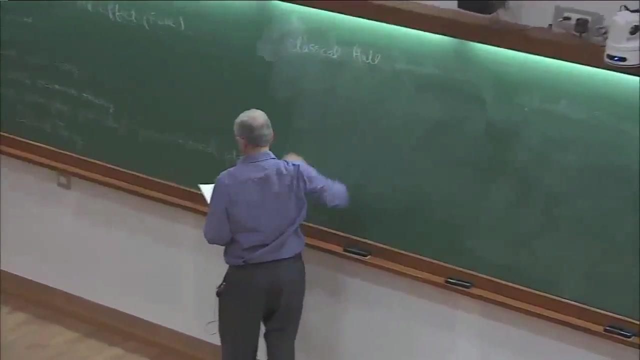 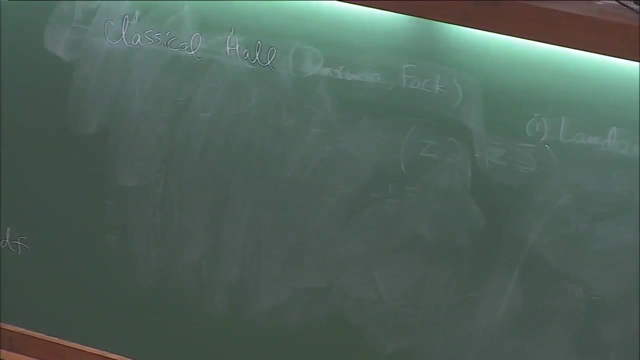 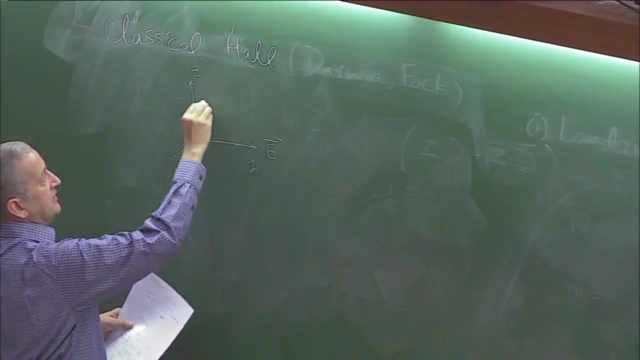 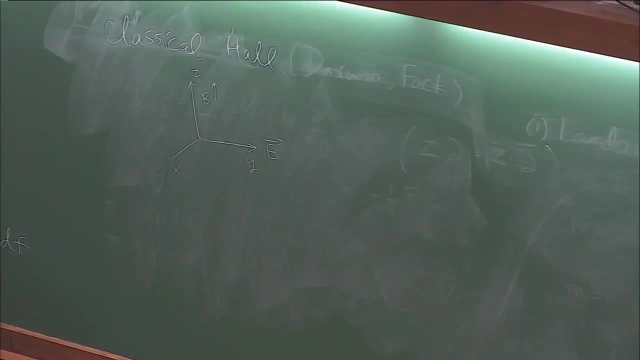 You may remember. so let us see, I am taking. so let us say the electric field is in this direction, the magnetic field is in this direction. then the actual trajectory of the charged, 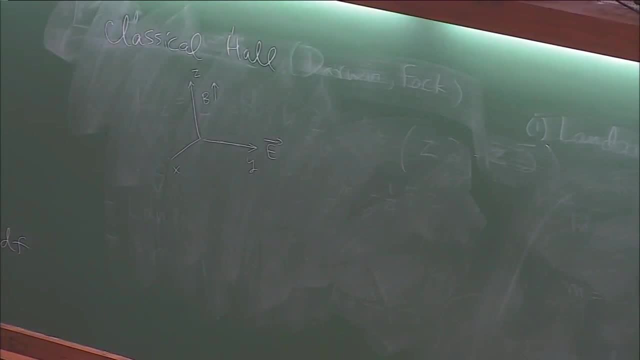 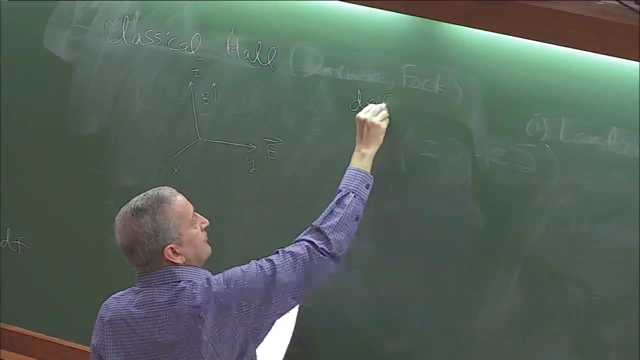 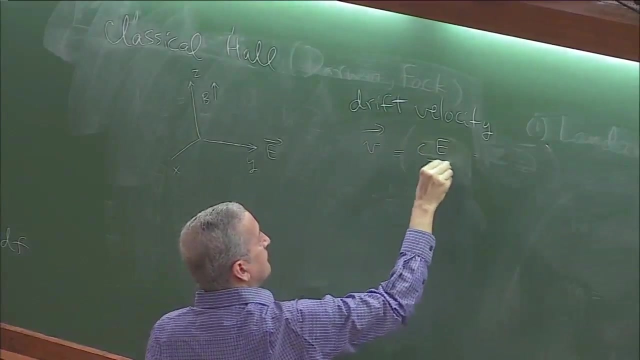 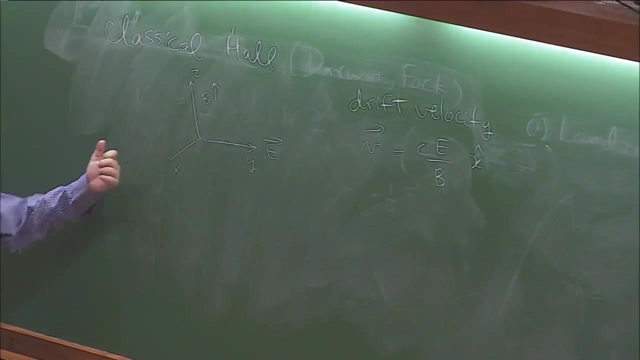 particle depends on the initial conditions, so it can go like this or it can go straight, but the main point is that it has a drift velocity and the drift velocity has a very simple form. So it has a drift velocity going along the x direction. so perhaps the simplest way to 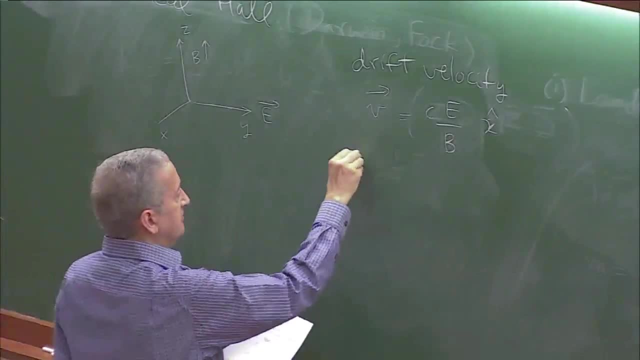 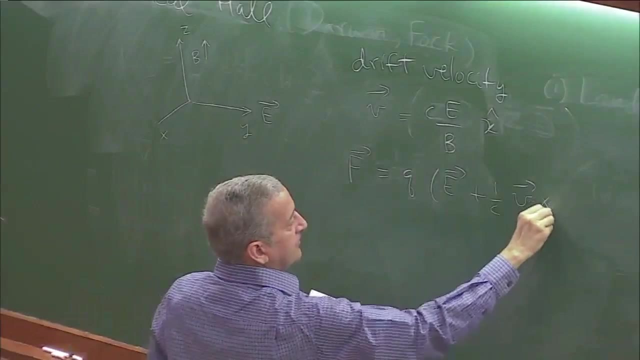 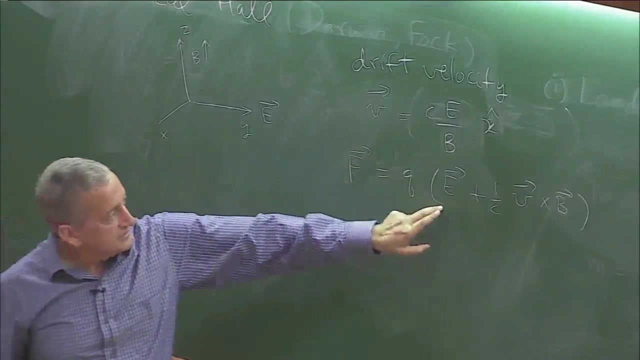 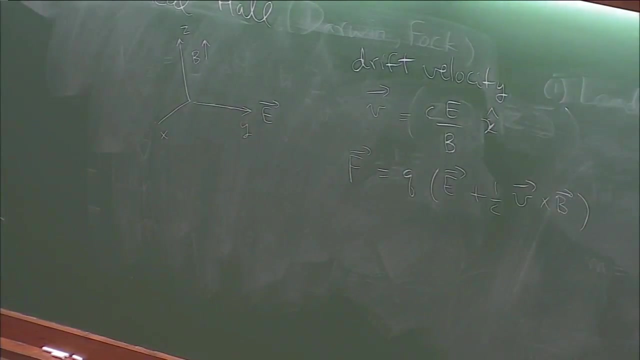 see, that is to just look at the Lorentz force law. and if you look at a particle with this drift velocity, then these two terms cancel, so there is no force and therefore the particle just continues to go in the x direction with this velocity. 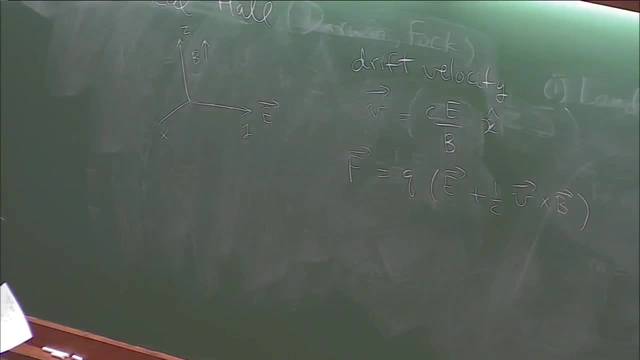 Okay. so let us ask: what is the Hall resistance? so the current density is charge times, rho times, velocity. Okay, Let us do in any dimension the Hall resistance. so I am here defining Hall resistivity, not the Hall resistance. we will come to Hall resistance in a second. 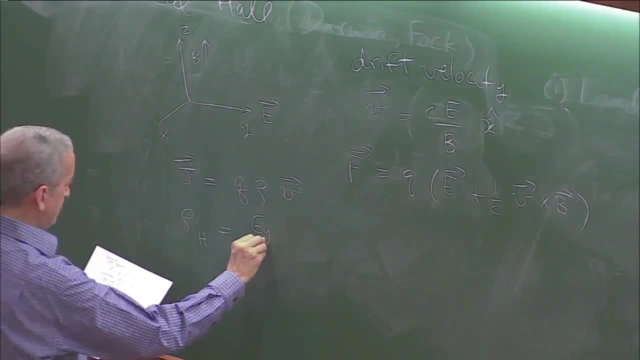 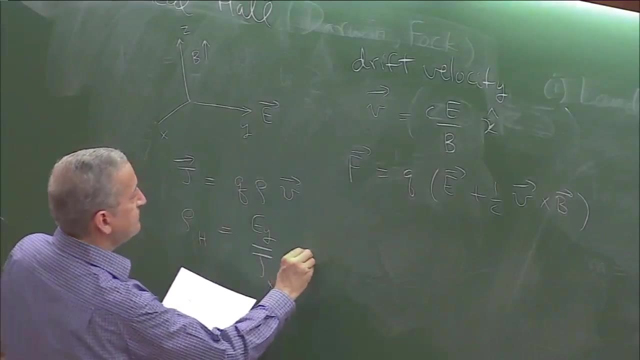 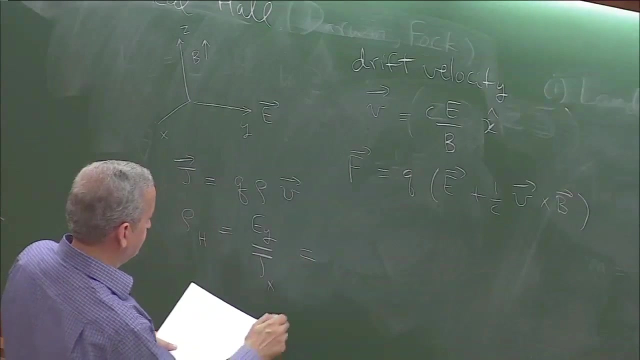 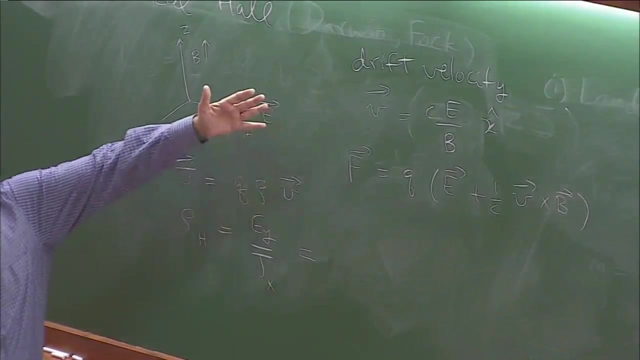 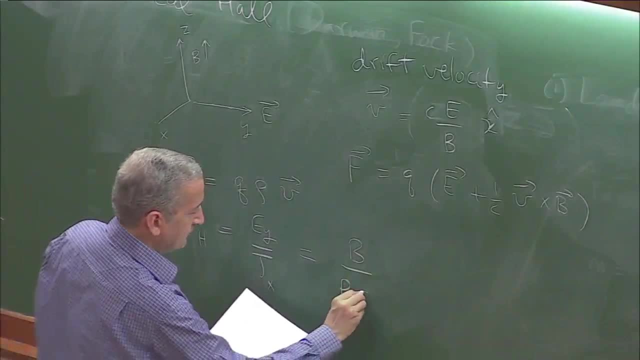 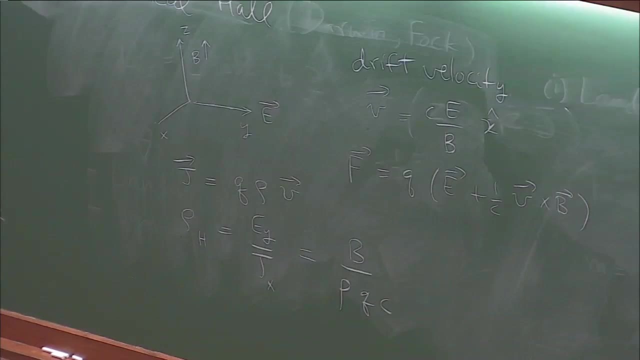 these quantities here and you will end up with this, this relation that I had shown on one of the slides. Okay, So all I have done here. this is the definition for the Hall resistivity. here I substitute for Jx this quantity with V, given by this equation, and I get the quantity on the right. 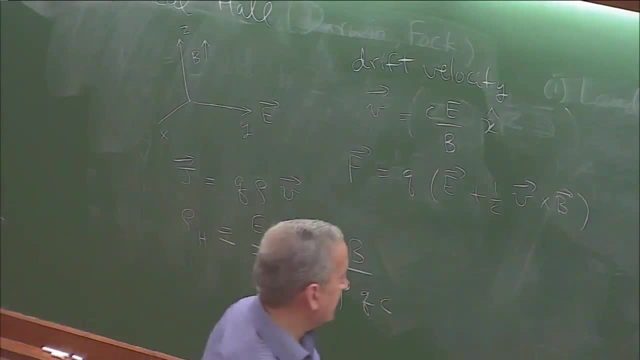 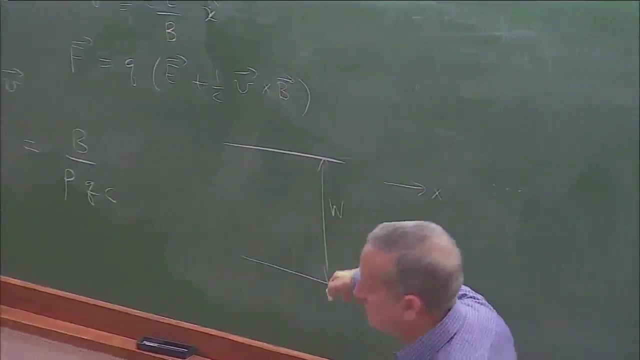 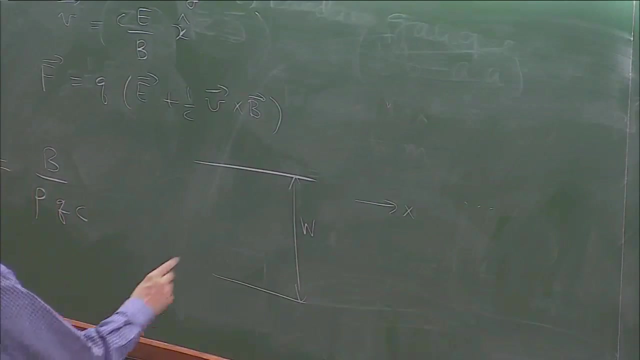 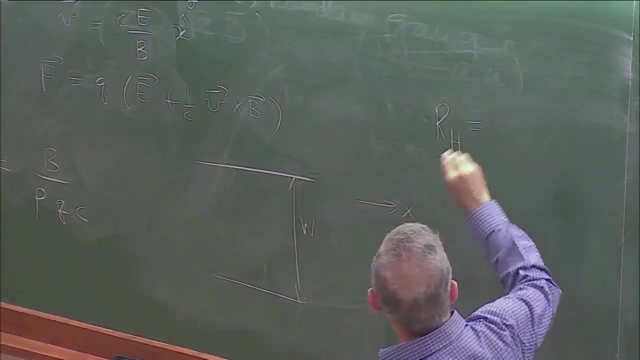 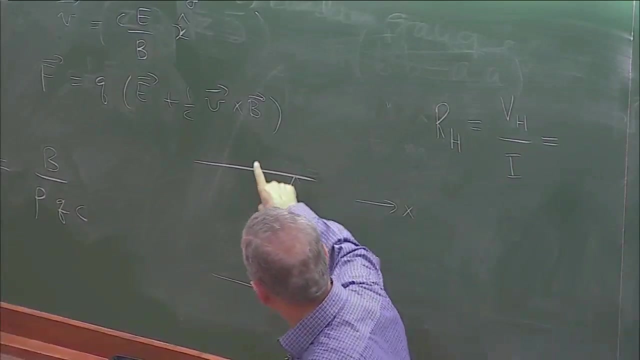 hand side. Now let us consider a two dimensional system. let us say: this is my x direction and the width of my sample is some W, and now I am going to write an expression for Hall resistance. So that is all voltage divided by current. all voltage is given by what? If I know the 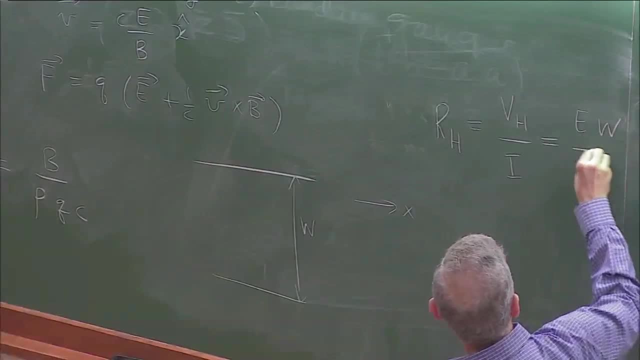 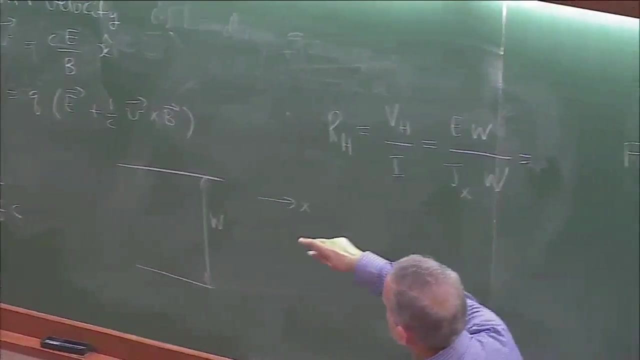 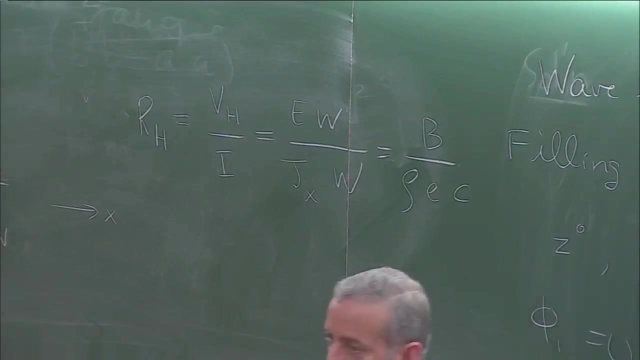 electric field. it is just electric field times the width, and the current in the x direction is Jx times the width. So in fact the width cancels out and we end up with the same relation for the Hall resistance, which is P, divided by rho, and let me put E, C and in.